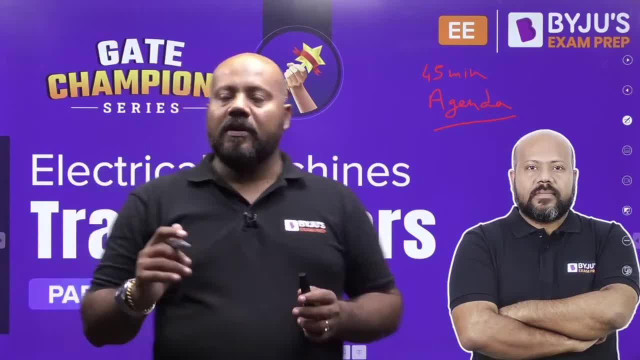 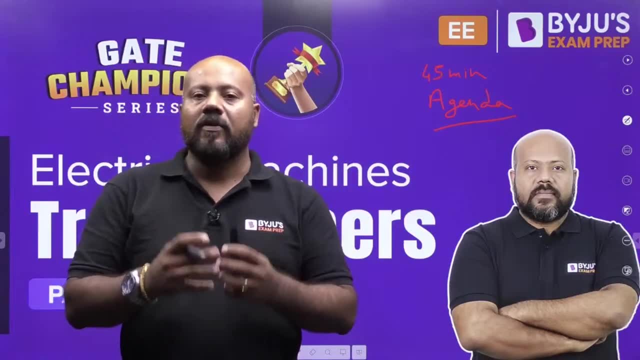 them with confidence. This session belongs to the gate champion series. Already lot of subjects, lot of sessions we have covered. So if you have missed those sessions, you can watch those sessions in the recorded form that is available on the playlist. on Byju's exam prep: All the candidates- 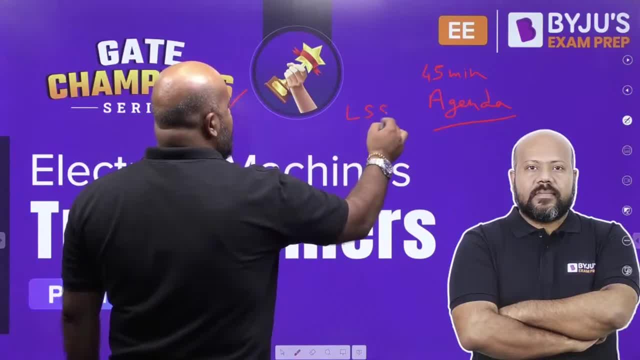 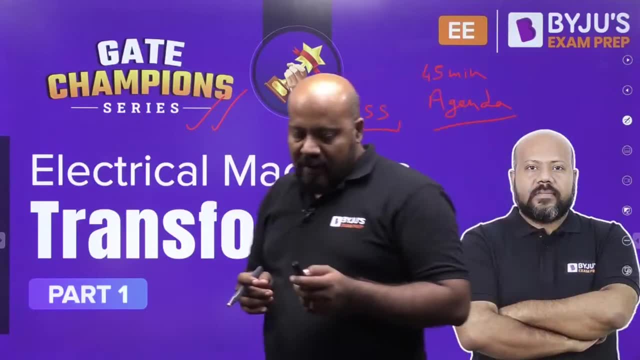 who are joining me live just quickly, like the session, share it with your friends and colleagues and subscribe to Byju's exam prep so that you do not miss any of the important sessions. So everybody, just tell me in the comment section: are you there, So that we can start. 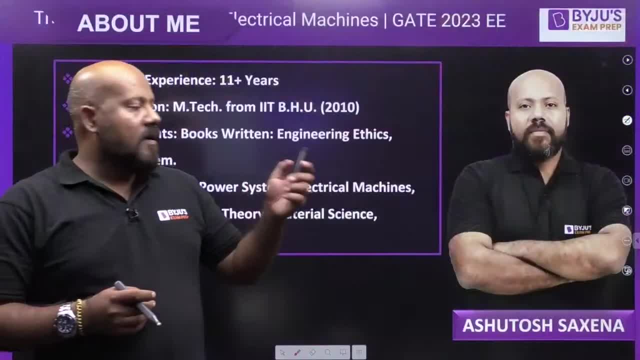 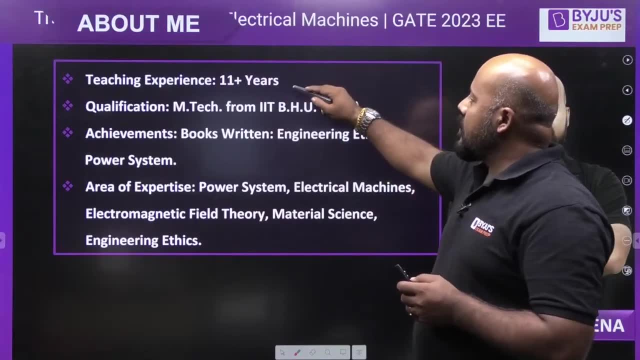 with the session. Yes, everyone, Some of you may be joining me for the first time, So there is a brief introduction about myself. My name is Ashutosh. As you can see on the screen, I have 11 plus years of teaching experience. I am from ITBH in 2010,. written couple of. 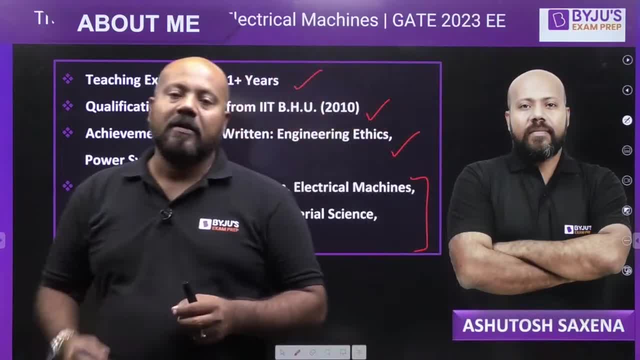 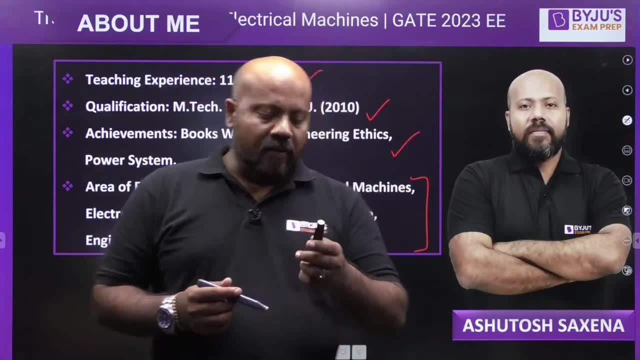 books, and my areas of expertise are power system, electrical machines, electromagnetic field theory, material science, engineering, ethics and current affairs. So let us start. Yes, Rohit Hi, how are you Welcome to the session? Before we start the session, if you are. 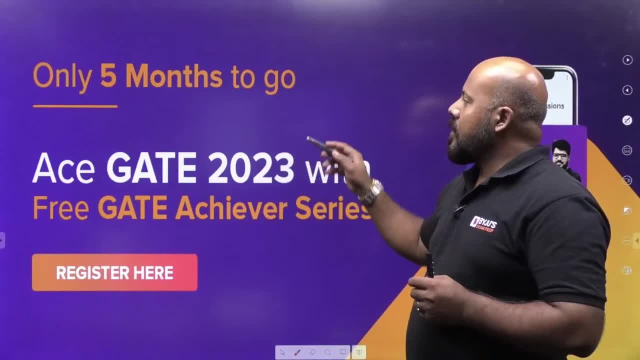 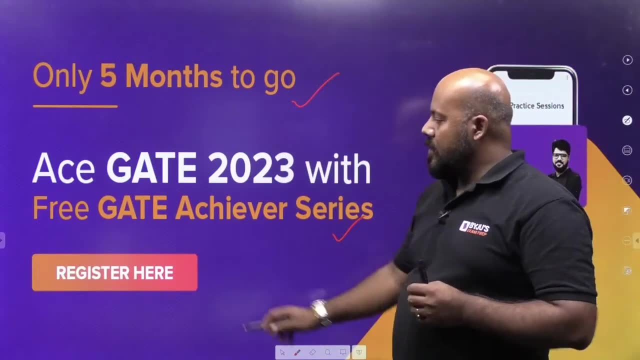 serious about GATE 2023 preparation, then you can complete your preparation in five months and you can join ACE GATE 2023 with free GATE Achiever Series, which is available on Byju's exam prep app, But you have to register for that particular series on Byju's exam prep app. 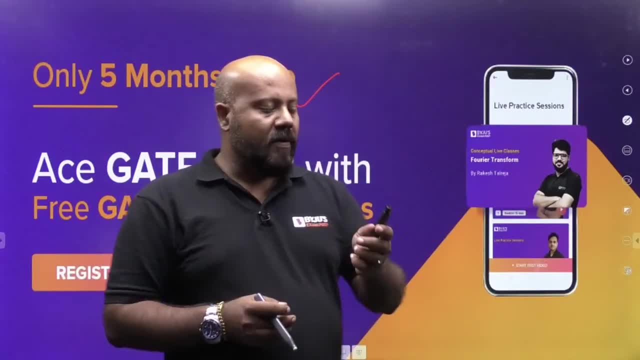 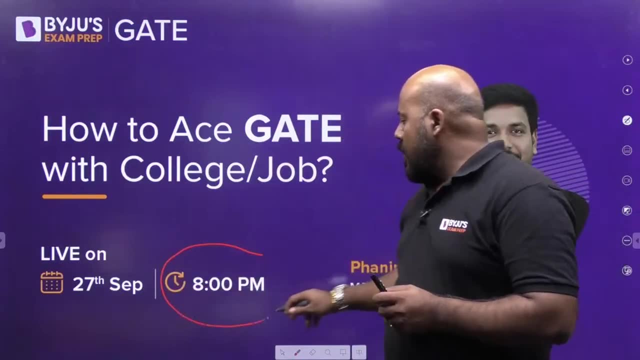 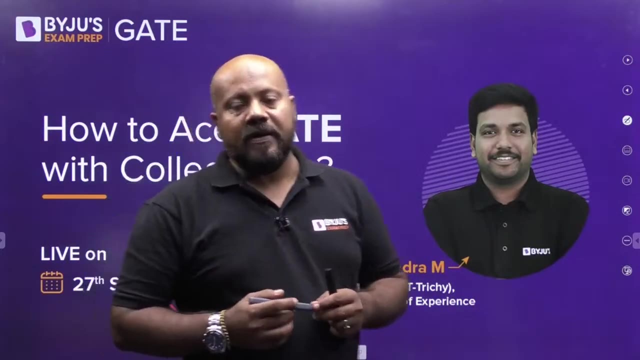 You can go to the app, follow the simple instructions and you can get yourself registered. The session itself: 8 pm in the evening. One of the most reputed faculty of instrumentation, that is Faneen sir. He is having more than 11 years of teaching experience. He is going. 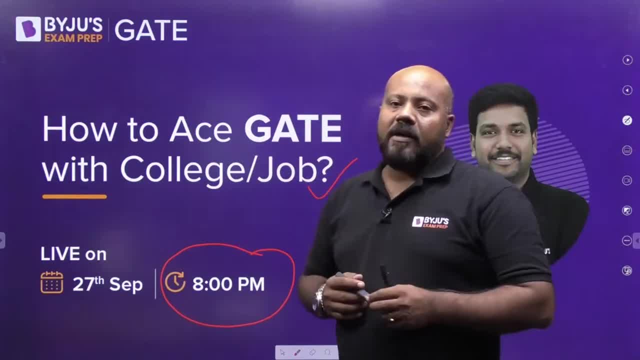 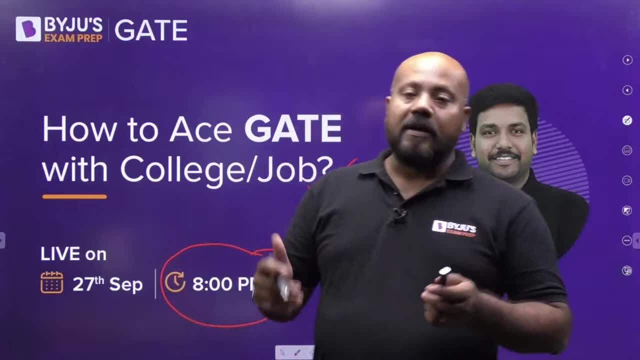 to discuss how to ace GATE examination. if you are a college going a student or you are a working professional, So this workshop is going to be important for all those candidates doing some job or already in the college. So if you are willing to join this workshop, 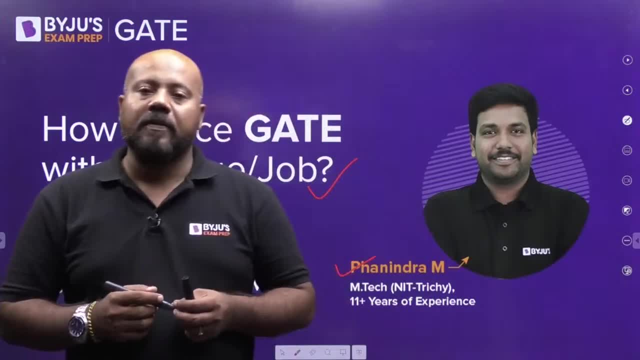 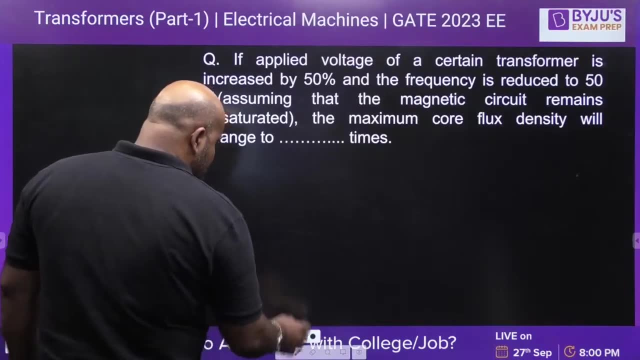 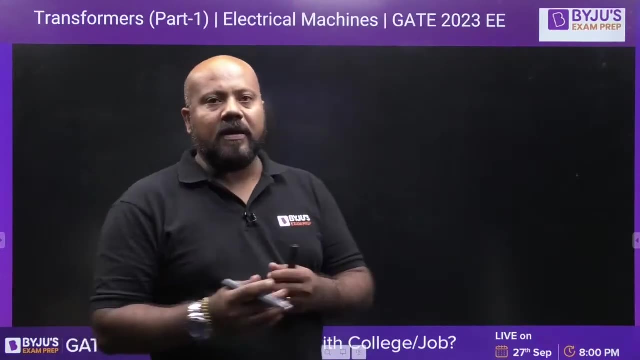 prep app. today itself, 27th of September, then you have to register yourself on the app. Let us start with the first question. but before I start with this question, let me just give you some brief idea, some background about the transformer, so that you can synchronize. 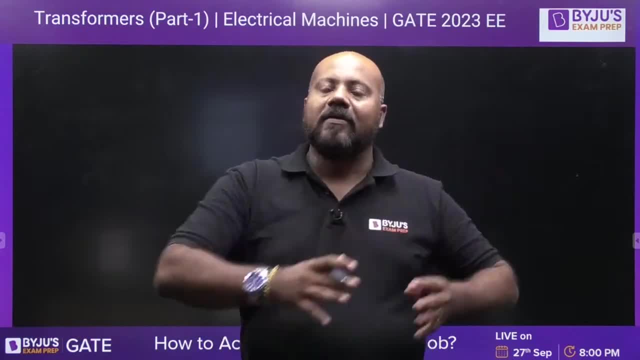 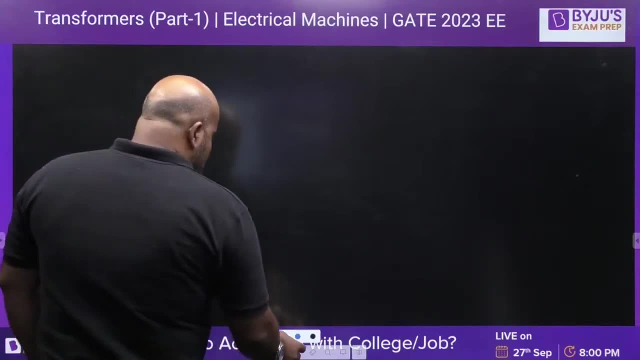 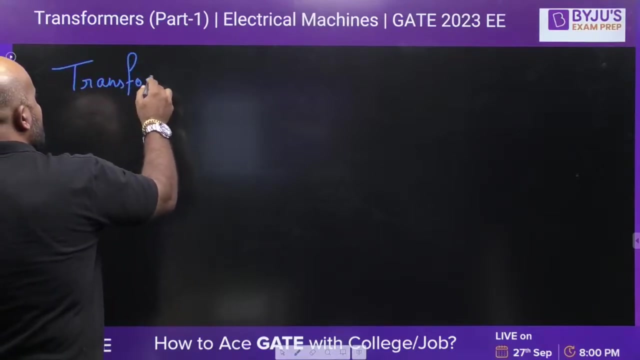 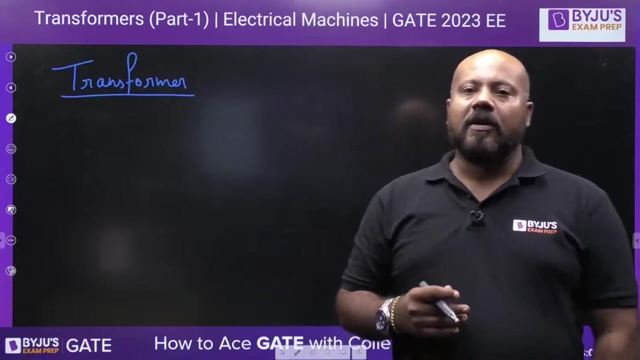 with what we are discussing and you will be having a better understanding of the questions related concepts. Everybody is okay with that? just tell me in the comment section. So let us first start with some basics about the transformers. The most fundamental concept related to transformer is the concept of MMF balance. 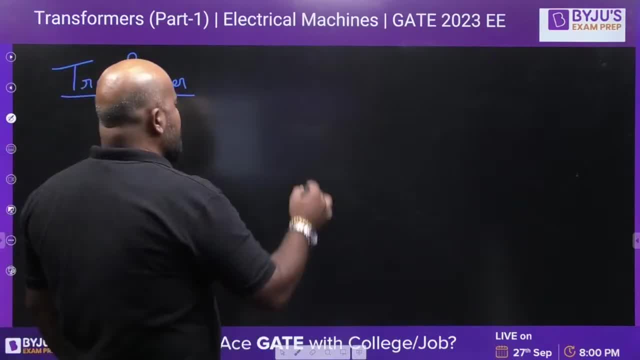 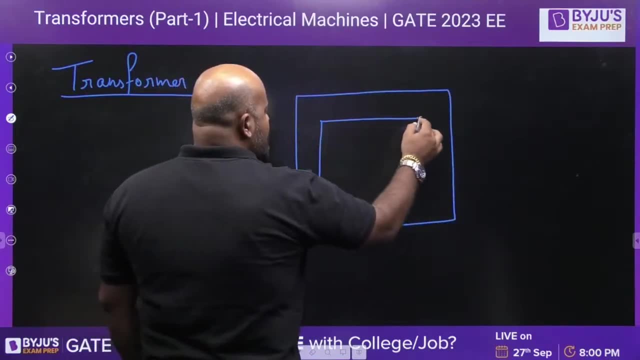 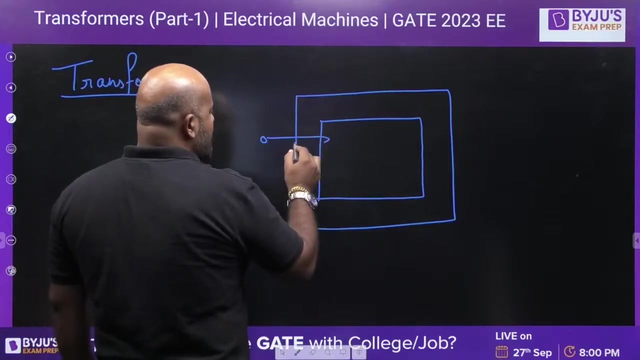 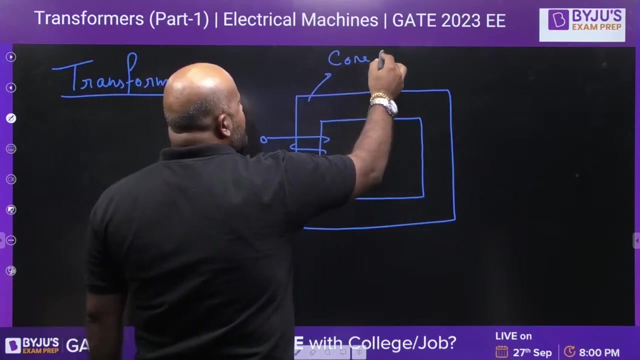 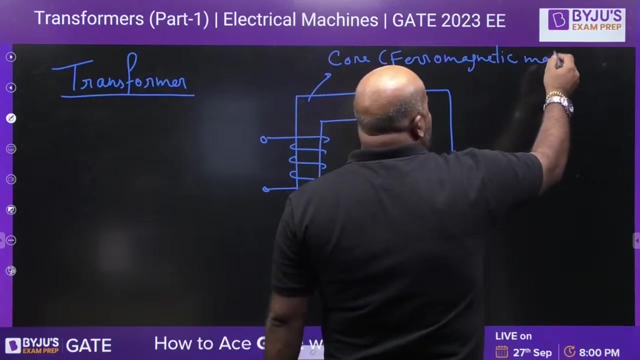 Good evening, Vishwanathan. Okay, So we will try to understand that concept. Okay, So this is the simple constructional diagram for transformer. This is your core. you must be knowing that this core is made up of ferromagnetic material. Why this is made of ferromagnetic material? 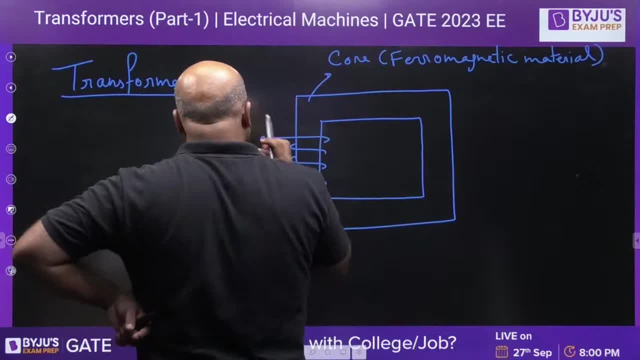 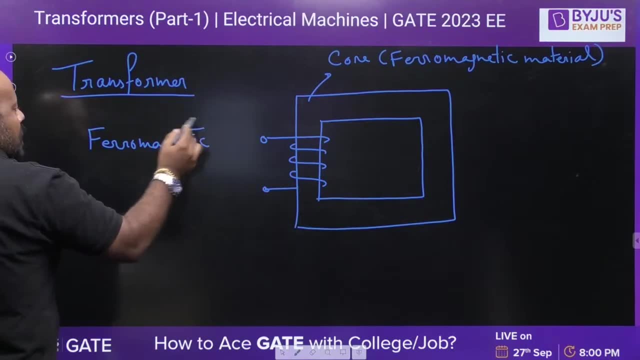 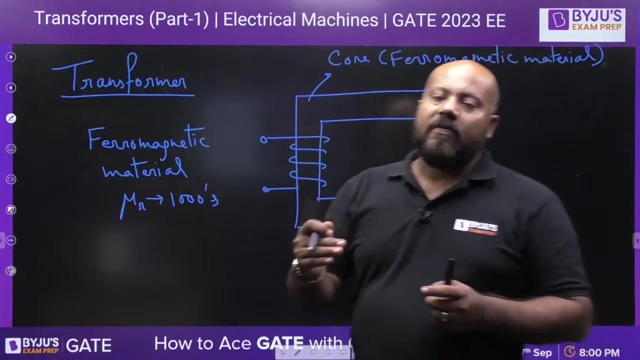 Because if you see for ferromagnetic material, Okay Okay. So if you see, for ferromagnetic material the mu r value is very high, it is in thousands, it is in thousands. So when the mu r value is such high, then to establish flux, the requirement of the magnetizing, 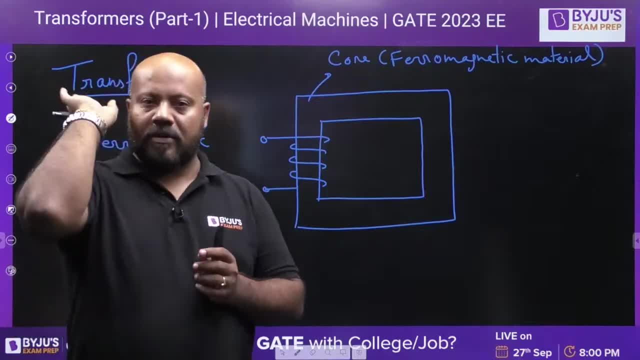 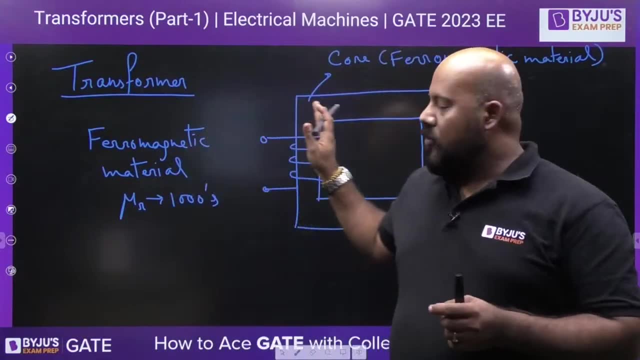 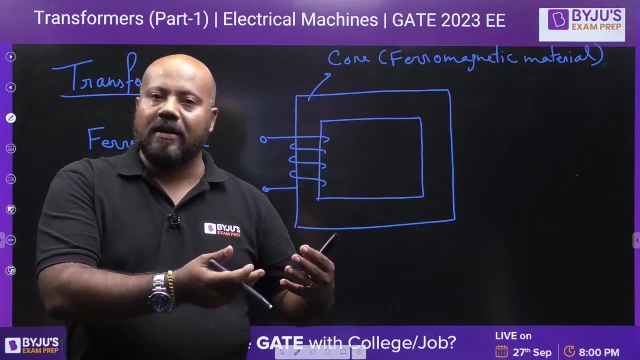 current is very less. it means a very small amount. very small, tiny amount of magnetizing current is going to be sufficient to establish flux in the core. and that is what we want, because transformer is going to work on the principle of induction. It works on the principle of induction. 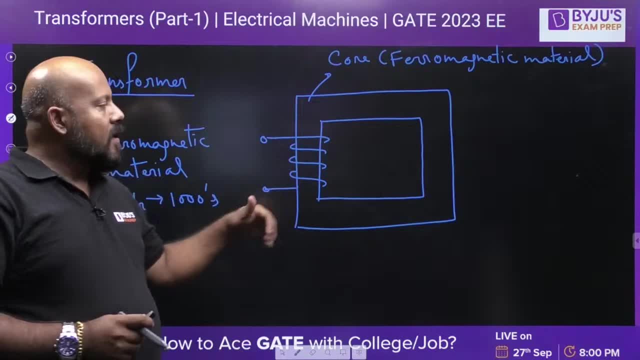 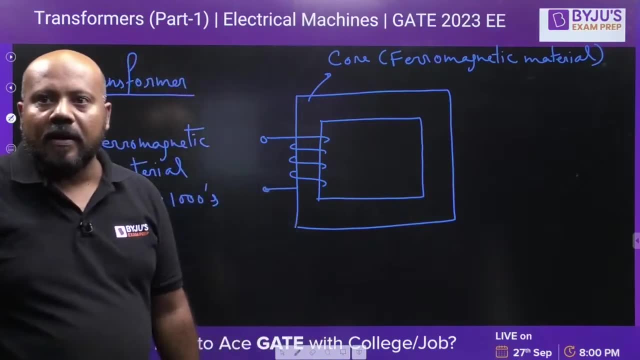 One winding you are going to provide the excitation, that is, the power supply. in the other winding, you are going to connect the load. yes, Ramesh, you are right. Good evening Pradhan. how are you welcome to the session? So this is the core, transformer, core. 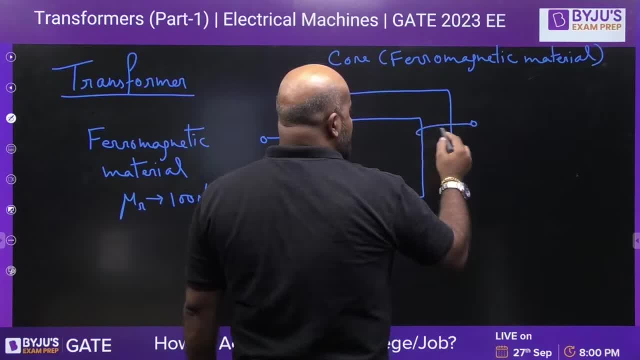 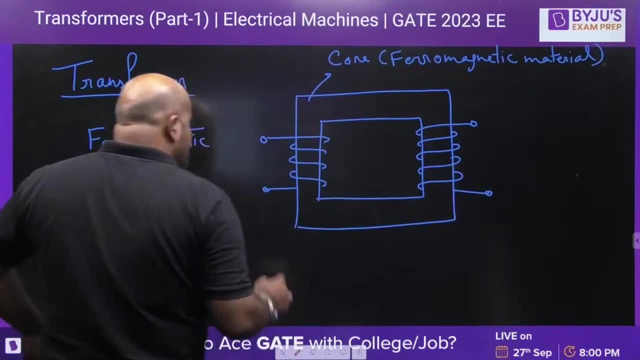 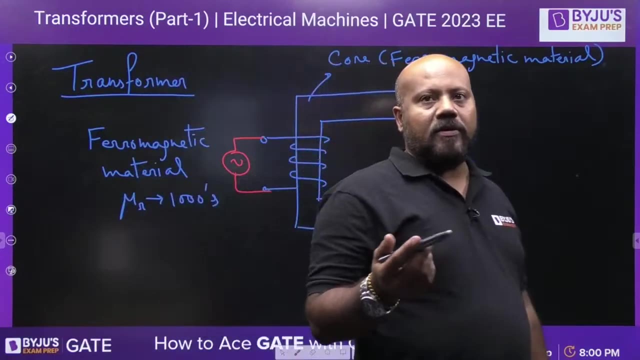 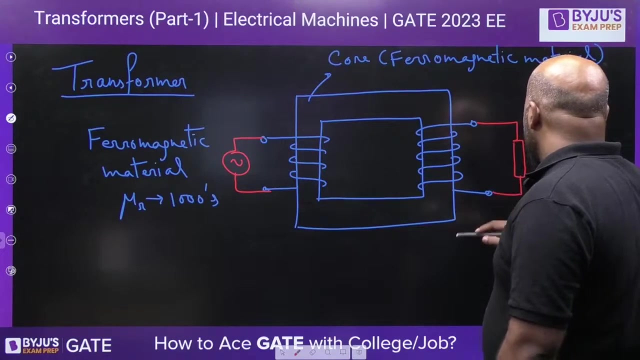 This is the primary winding. Okay, This is the secondary winding. Is it clear, everybody? now we are going to connect the source here. obviously it is going to be AC source. we do not operate transformers with the DC source, you know, because the winding can be damaged. yes or no, the winding can be damaged. is it clear? now, suppose in the starting. 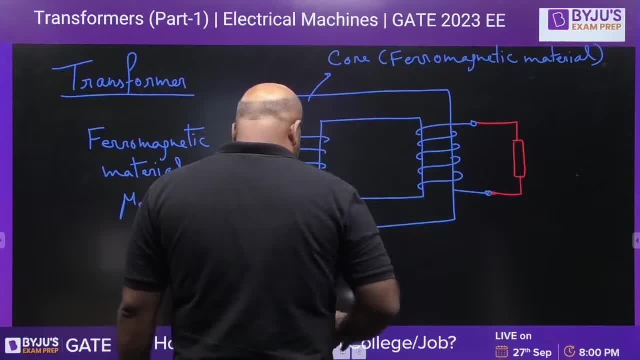 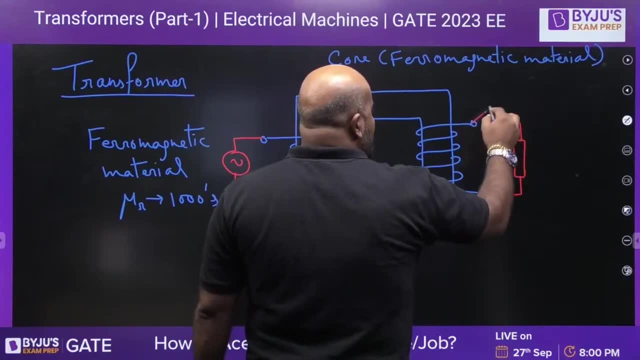 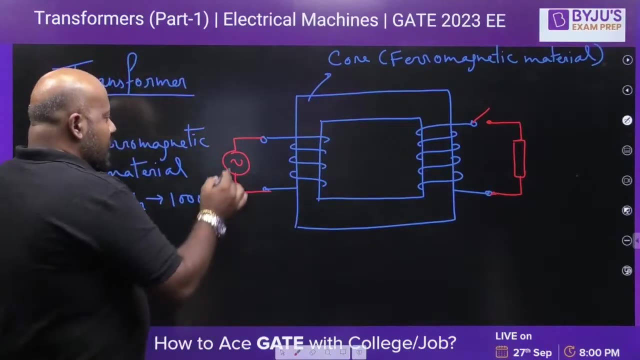 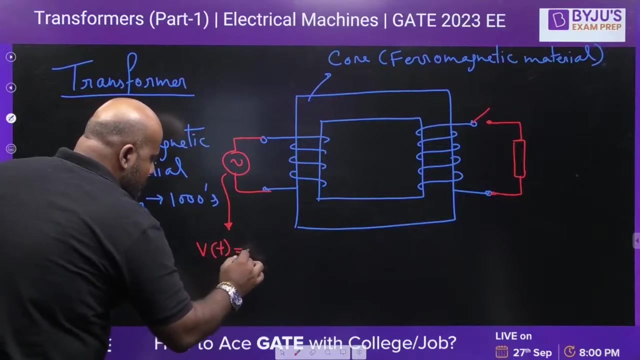 part. we are saying that this switch is open. Suppose this switch is open, it means at the secondary the load is not connected to the circuit. it is open circuit. but when you are giving the excitation, suppose this excitation is, it is root. 2 v sine omega t. 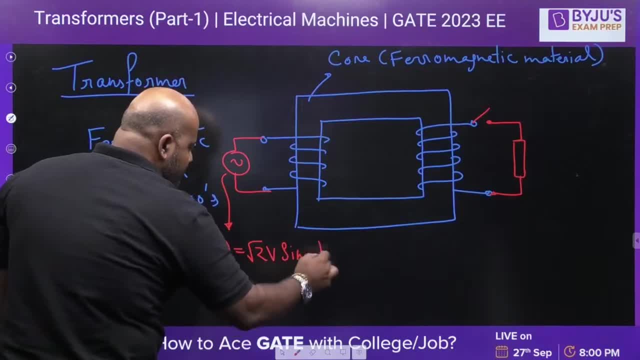 Where v is going to be 2 timesui d omega t. In what is the excitation going to happen? So the excitation is going to be 2 timesui d omega t, Yes, to be the rms value. that is why we are writing it like this: root 2 v sine omega t, because for 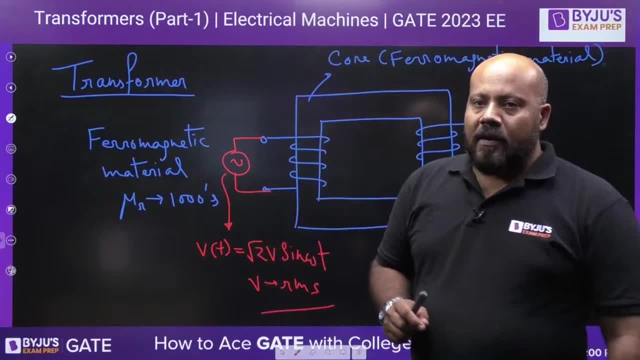 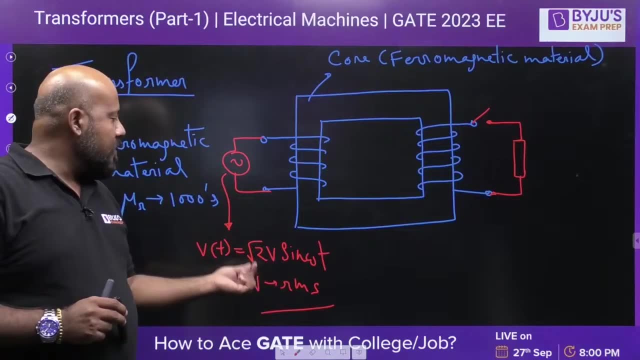 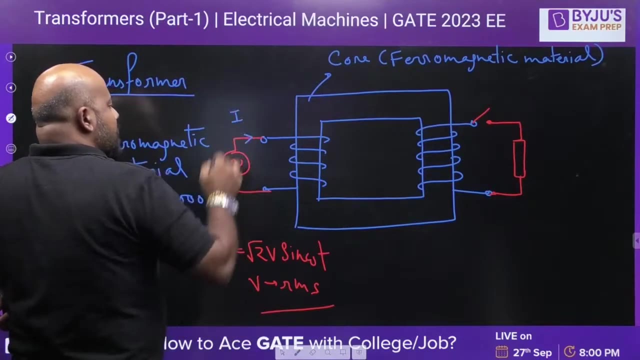 sinusoidal functions. we have to write it. yes, we have to write it in terms of peak value. that is why we have multiplied v with root 2. anyways, now you will be having some current here. suppose the rms value of the current which is coming here is going to be i. okay, now this current is passing. 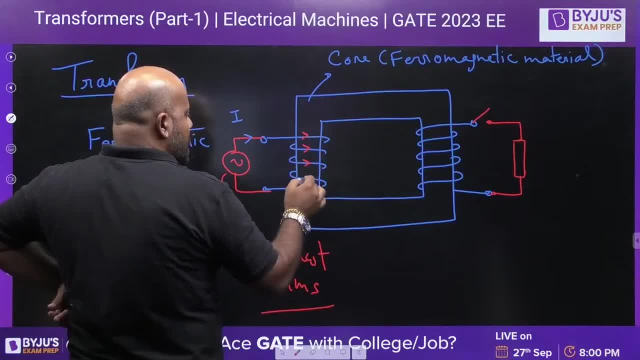 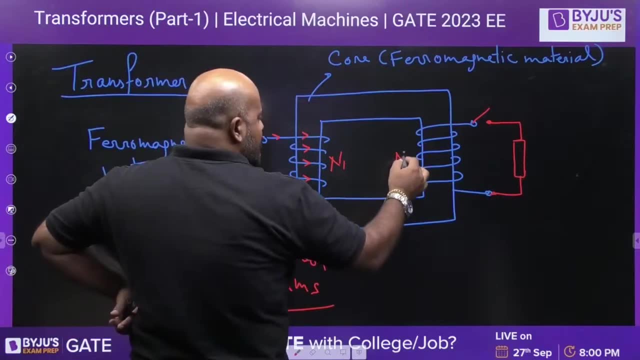 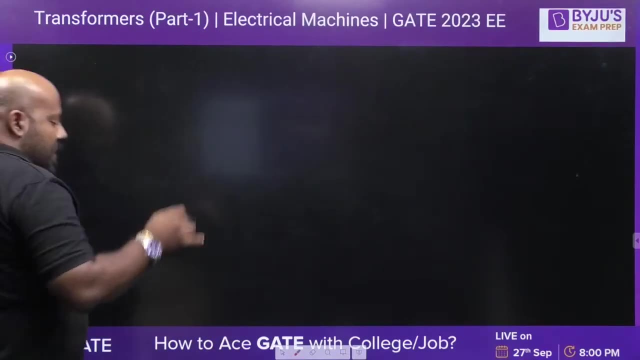 in the primary winding like this, yes or no? suppose the number of tons of the primary winding is n1 and the number of tons for the secondary winding is n2. now see what is happening. when i1 current is flowing in the n1 turns of the primary winding you will be getting. 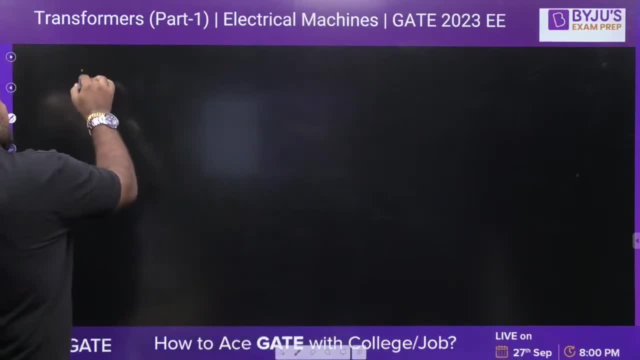 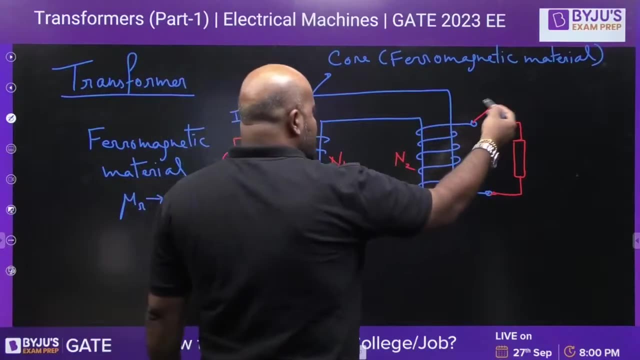 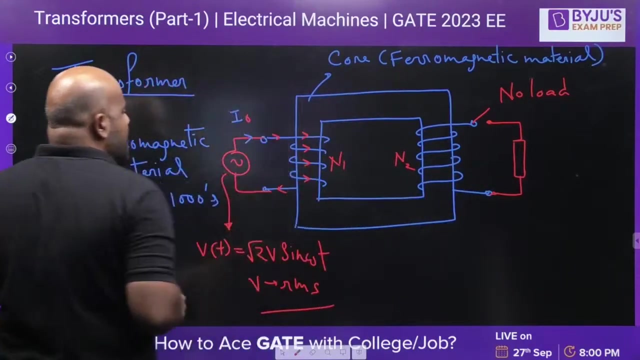 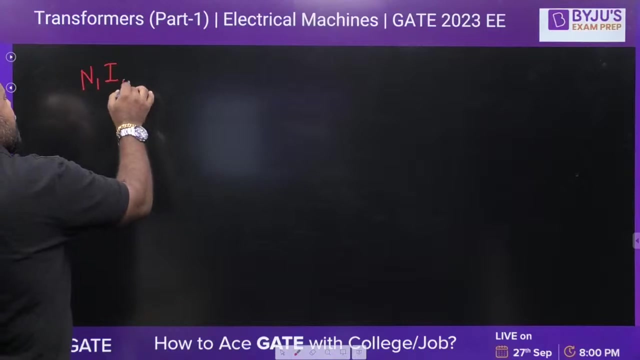 the primary mmf yes or no. primary mmf n1, i1. but because this is the open circuit condition, this is the no load condition, because load is not connected. so we are writing this current as i naught. we are writing this current as i naught. so the mmf in this condition at the primary side is: 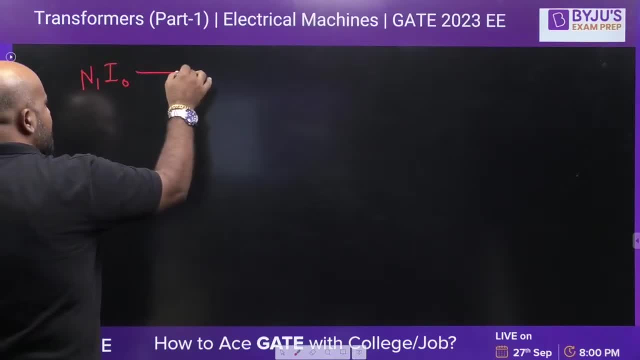 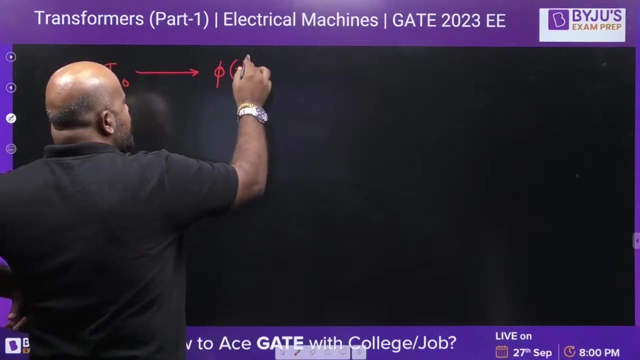 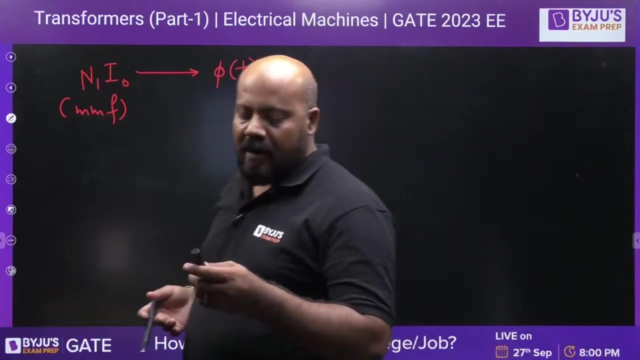 going to be n1. i naught this mmf will be responsible for setting up flux in the core. suppose the flux is going to be phi t. why the flux is phi t? because the source is alternating. if the source is time dependent, definitely the current is going to be time dependent. if the 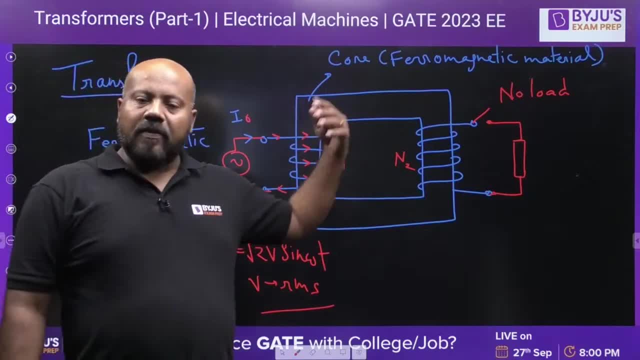 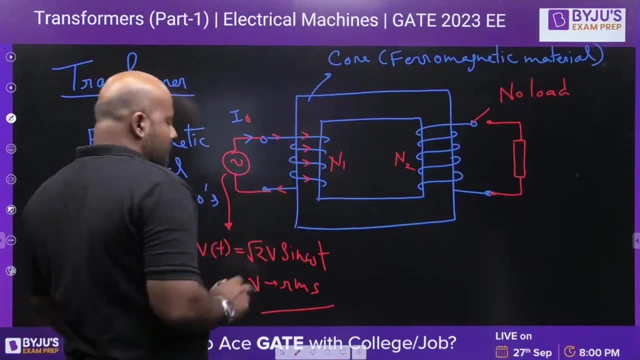 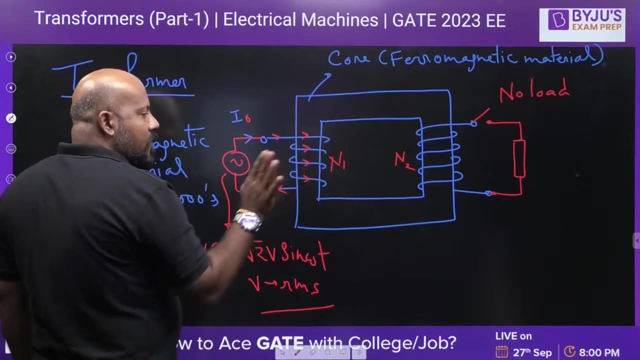 current is time dependent, then the developed flux is also going to be time dependent. so if you see for this particular direction of current, in this situation, what is going to be the flux, the direction of flux, you can find by using the right hand thumb rule: move your fingers, move your fingers. 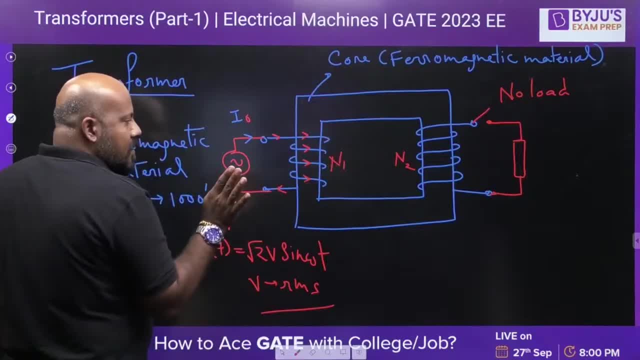 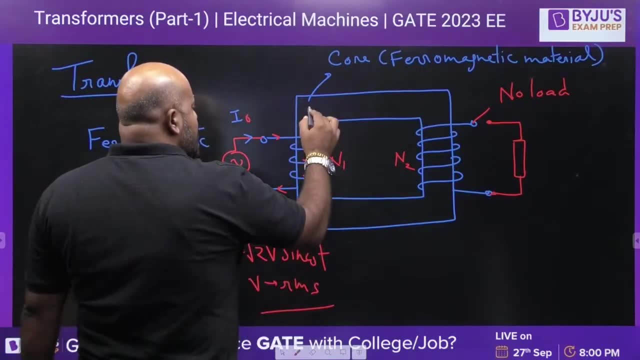 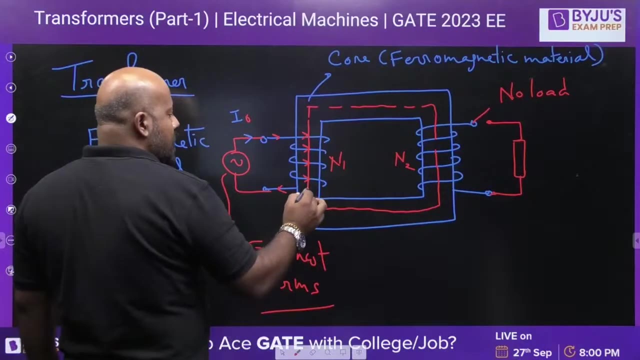 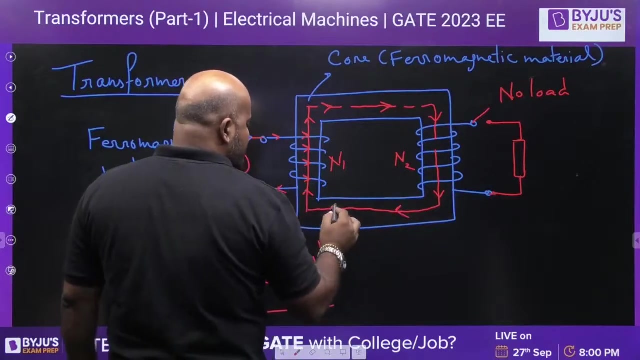 in the direction of current sense, current flowing. that is my left to right, and thumb, thumb is going to point towards the flux. so your flux direction is going to be something like this: yes or no. something like this, this is going to be your flux direction and this is a time dependent flux. this is a time varying flux. 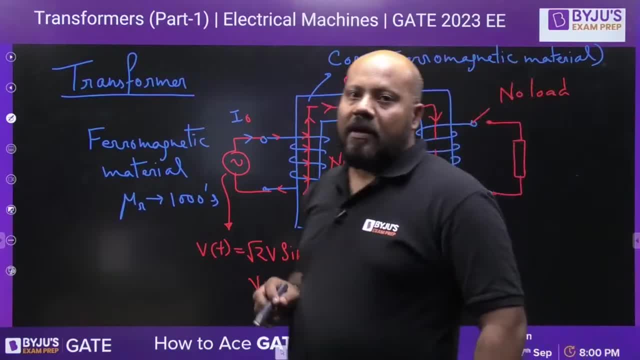 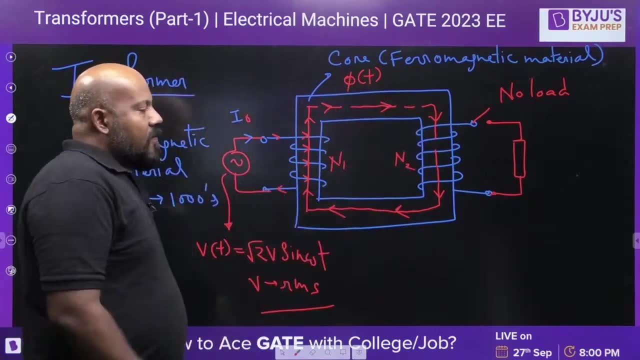 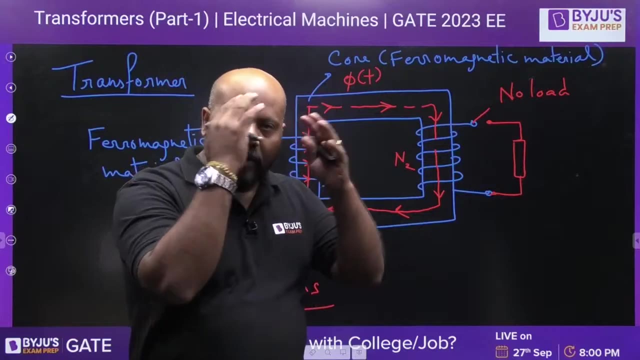 this time varying flux. this time varying flux is linking two windings, the primary winding and the secondary winding, when the two windings are having a linked flux, which is a time varying flux. so, with all due respect to faradays, there will be some induced emf. 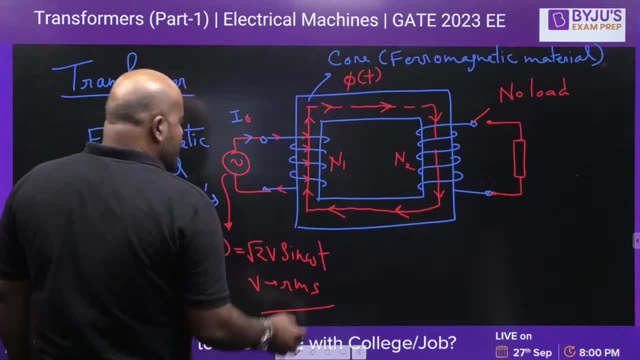 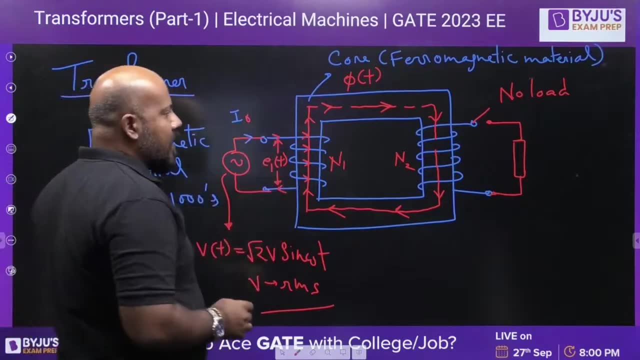 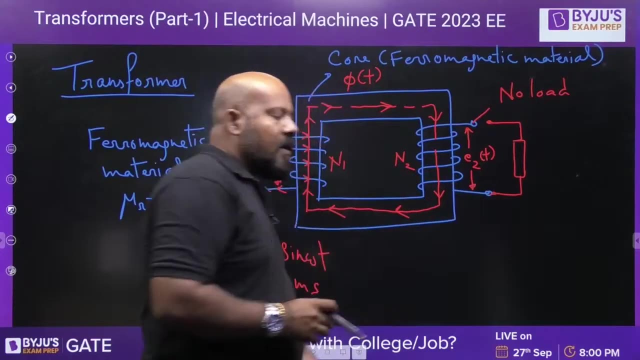 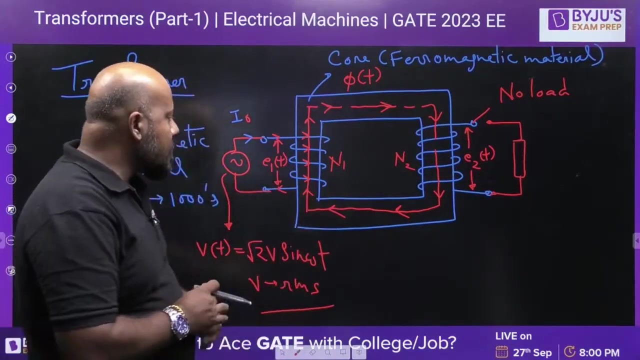 let the induced emf is. let the induced emf is e 1 t at the primary side and the induced emf is e 2 t at the secondary side. in the secondary side there will be no load current because load is not connected, but definitely emf will be induced, yes or no? emf will be induced now. please try. 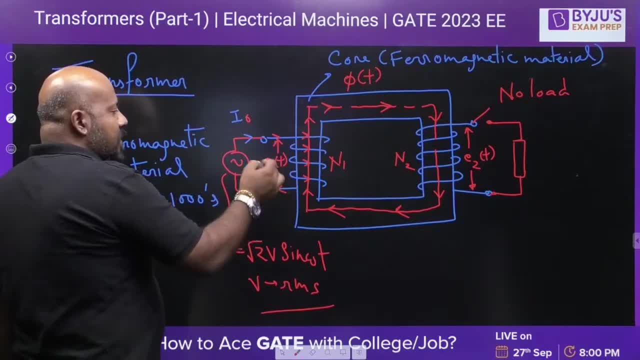 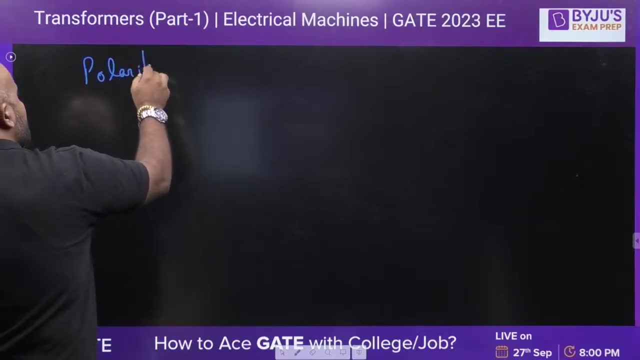 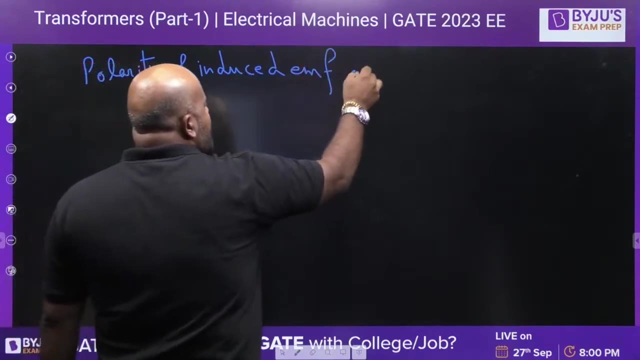 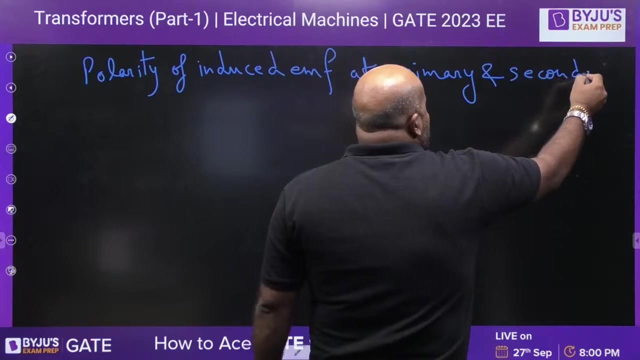 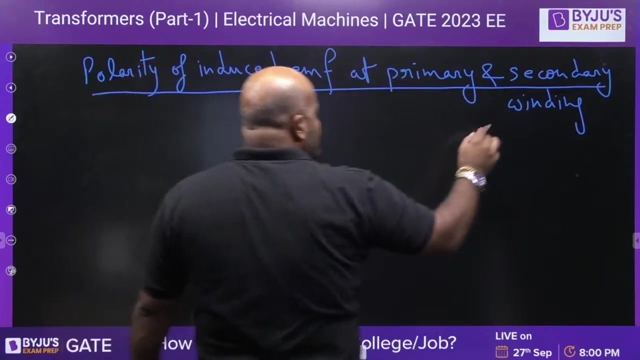 to understand what is going to be the polarity of these induced emf: e 1 and e 2. what is going to be the polarity of this induced emf? polarity of induced emf: this is very important at primary and secondary winding. now please try to understand how we are defining the polarity of e 1 and e 2. 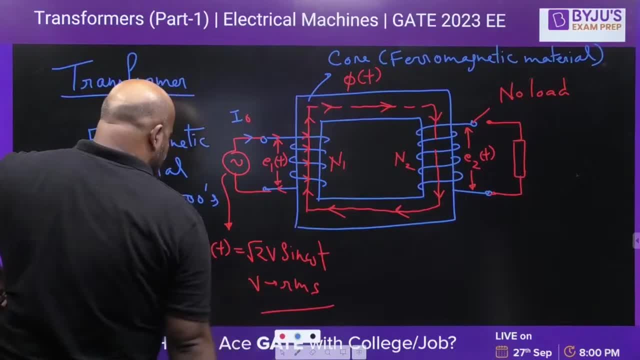 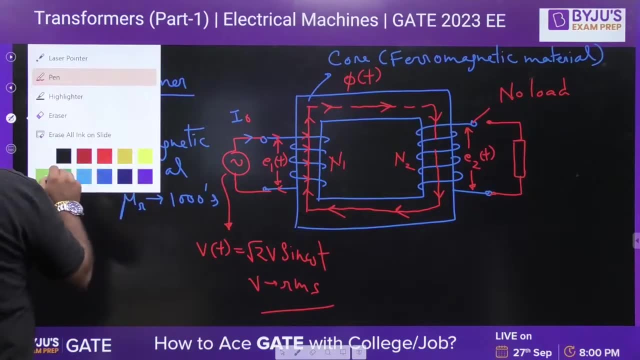 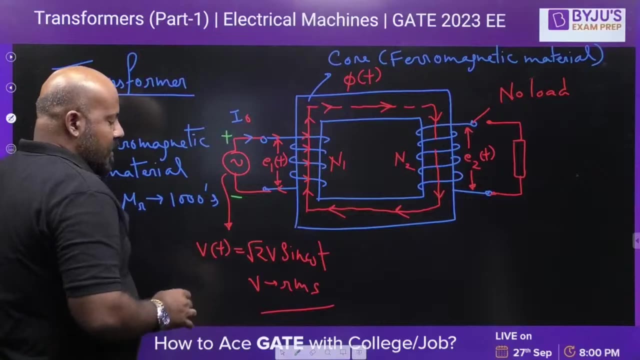 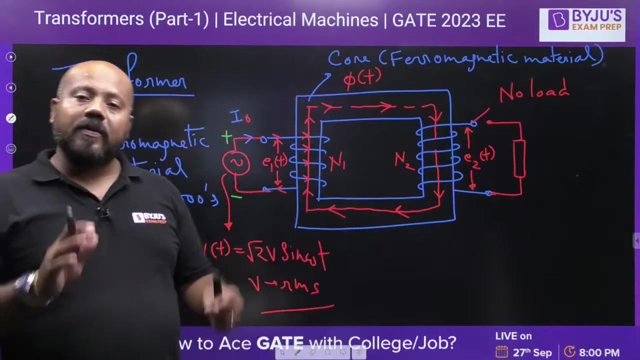 suppose, at any point of time, let me use some another color. yes, suppose the polarity is going to be like this: plus and minus for the given situation, for the source. okay, how we are defining the polarity of e 1 and e 2. please try to understand. 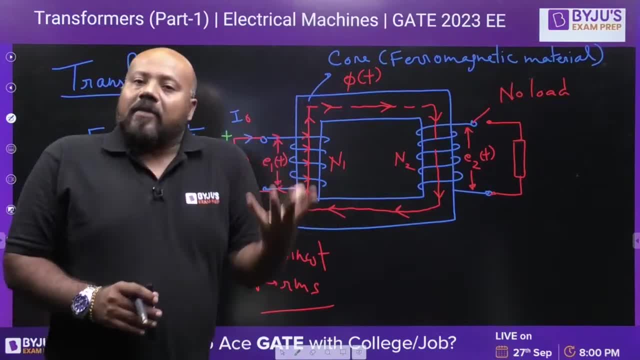 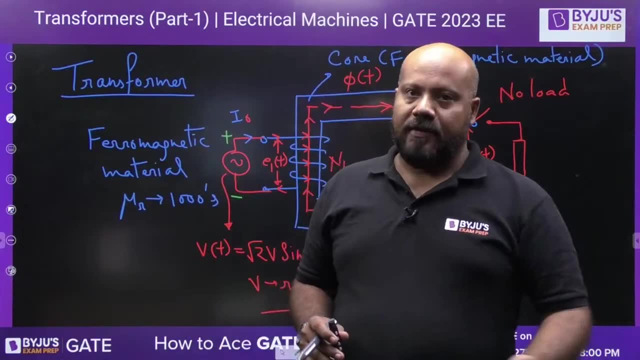 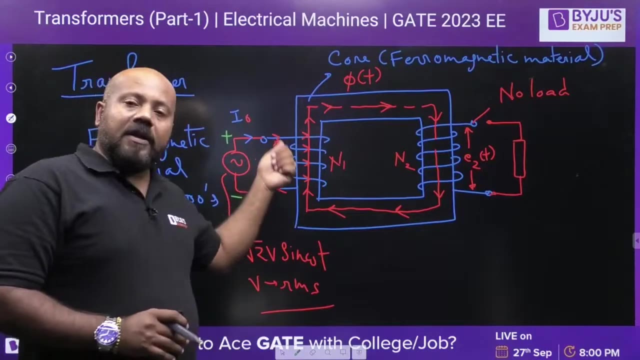 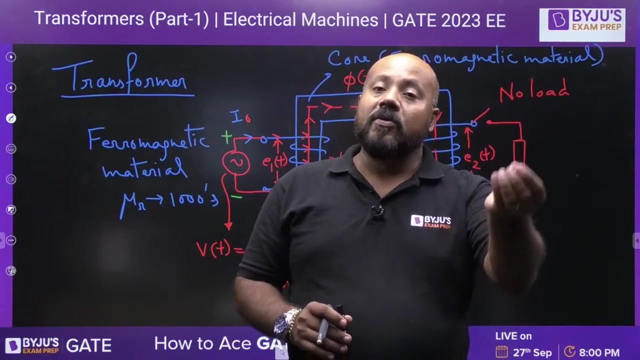 the polarity of e 1 will be such that that, given an opportunity, it will try to flow a current which is going to oppose its own cause, as per the lens law, yes or no. given an opportunity, e 1 t, this induced emf will try to flow a current in such a direction so that it can oppose its own. 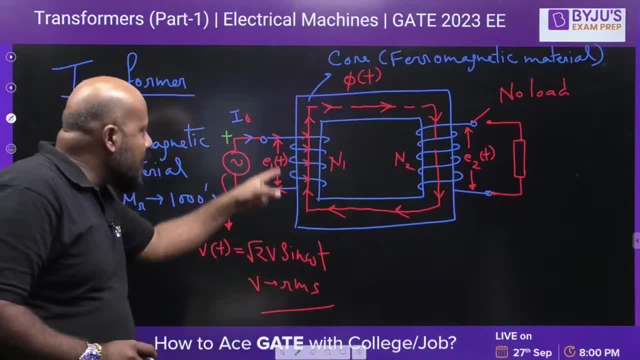 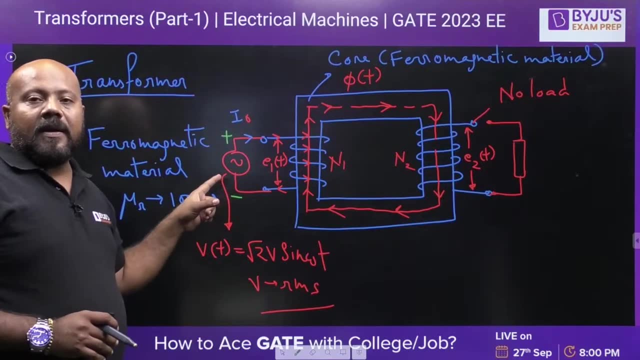 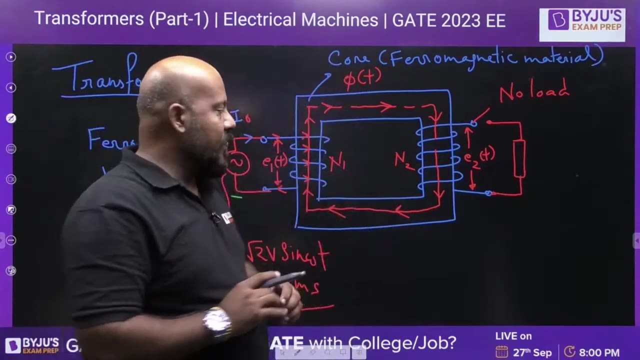 cause. now you tell me what is the cause. why e 1 has developed, why even has induced? because there was a current. why there was current? because there was a source. it means the polarity of e 1 is going to be such that it is going to oppose the source itself. so at any point of time, if this 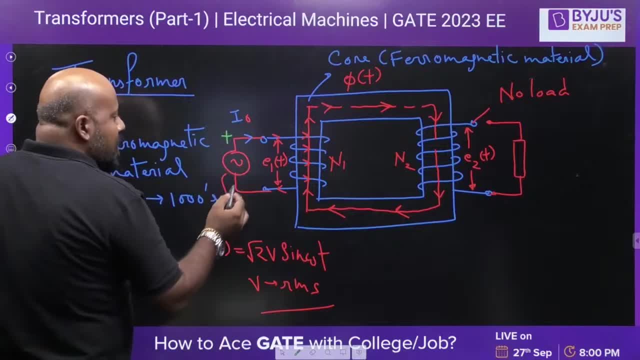 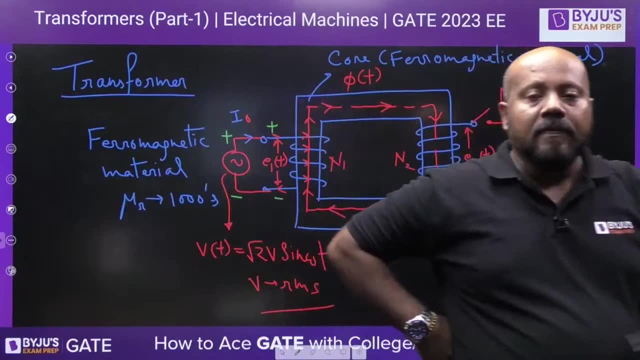 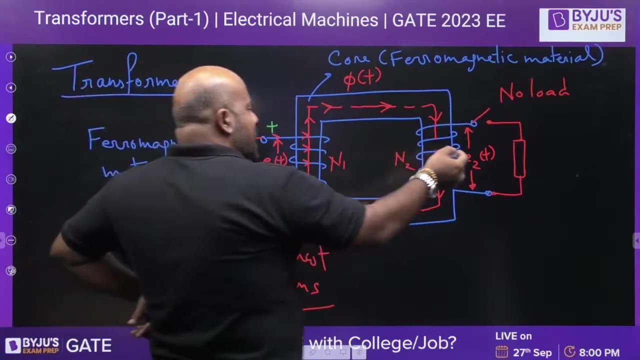 is the polarity plus and minus for the source. then the polarity of e 1- t is going to be like this: plus and minus. is it clear? everybody, everybody, just tell me in the comment section, say yes or no. yes, now let us try to understand the polarity of e 2. 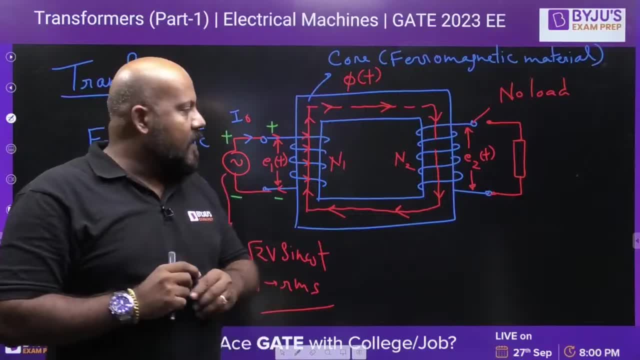 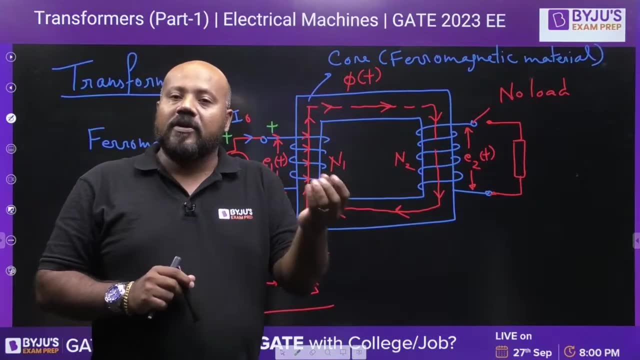 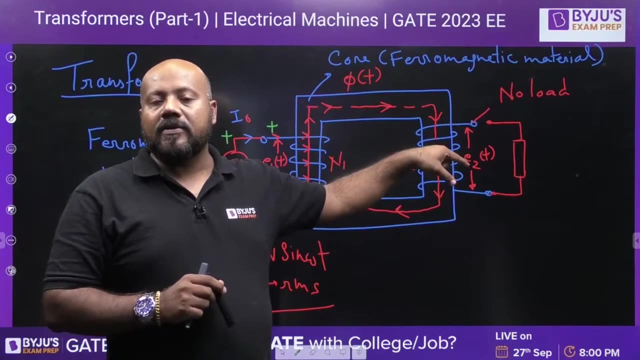 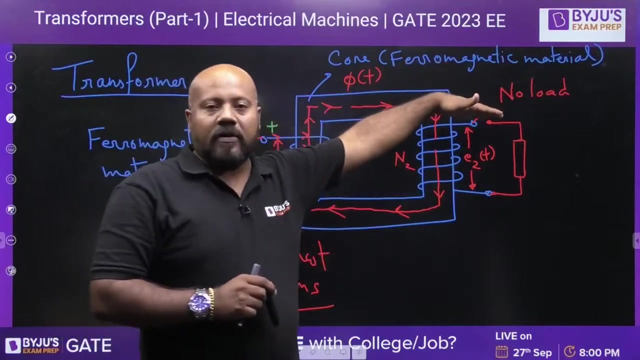 the polarity of e 2 is going to be such that, given an opportunity, this e 2 t will try to flow a current which is going to oppose its own cause. now, what is the reason why e 2 has developed, why e 2 has induced? the reason is time varying flux, yes or no? so, if suppose, if this switch is closed, 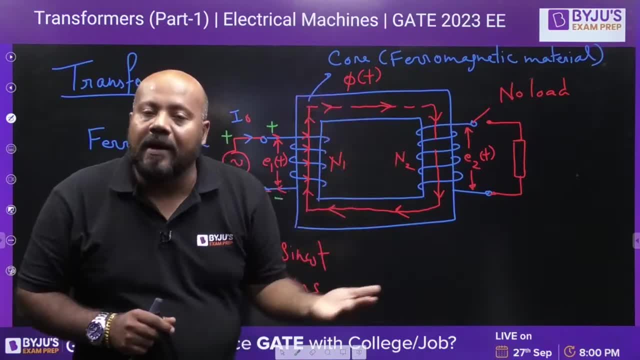 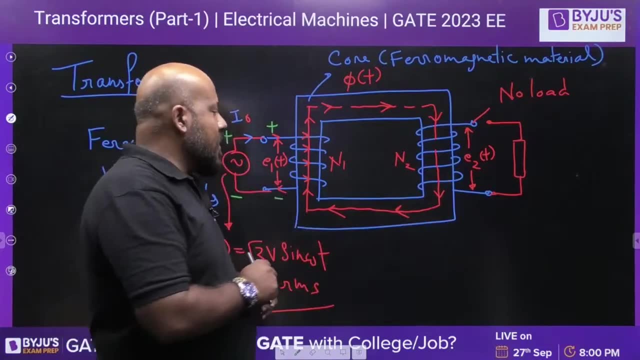 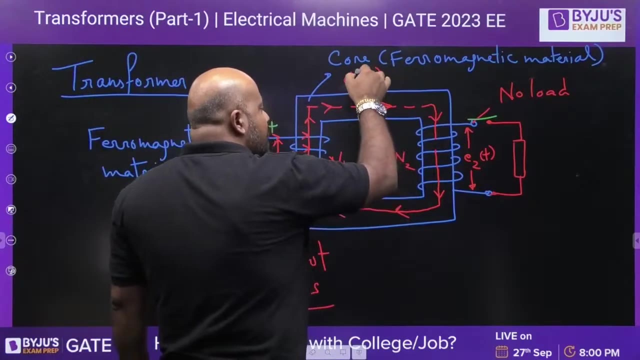 this induced emf e 2 t will try to flow a current so that it can oppose this flux. yes or no? now please try to understand. suppose i am assuming this switch is closed. if this switch is closed, this flux in the core is going from top to bottom. 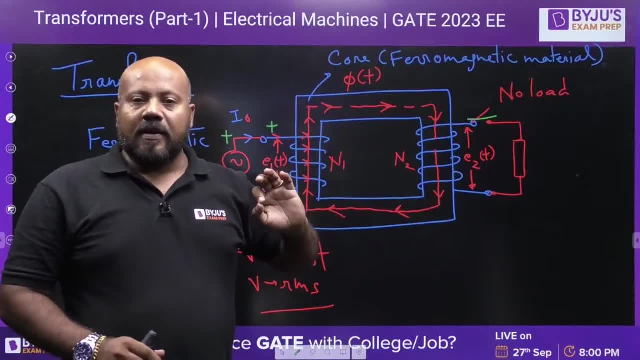 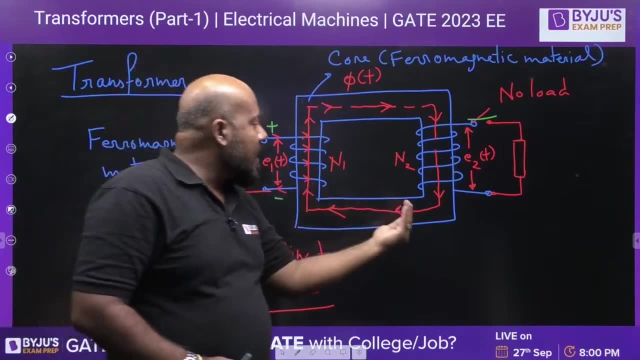 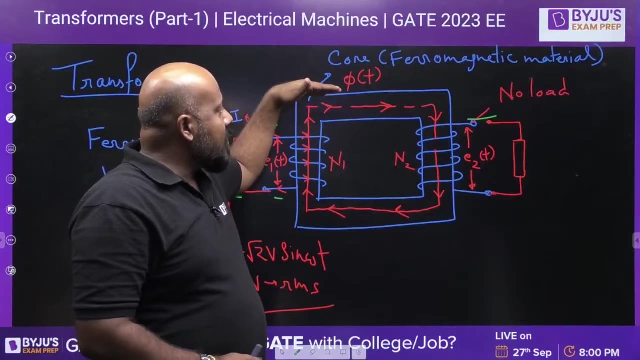 this flux in the core is going from top to bottom, then the current in the secondary winding will be such that it is going to have a flux which is opposite to this: bottom to up. yes or no? this main flux in the core is going from top to bottom. the emf e 2 induced in the secondary 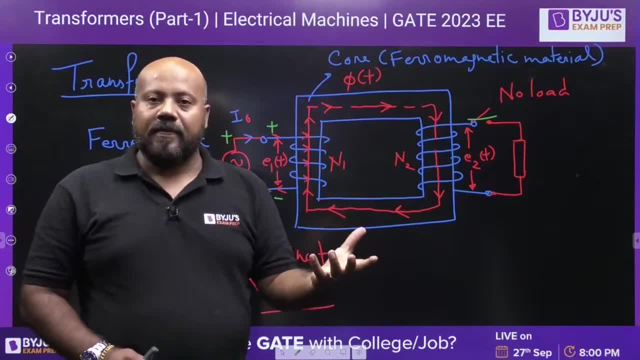 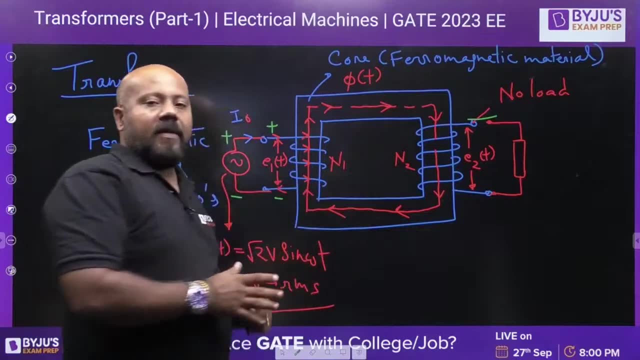 winding will be such that it will try to flow a current if this switch is closed, so that the flux is bottom to top. so you will again apply the right hand thumb rule. what is the direction of flux you want? main flux is top to bottom, you want. 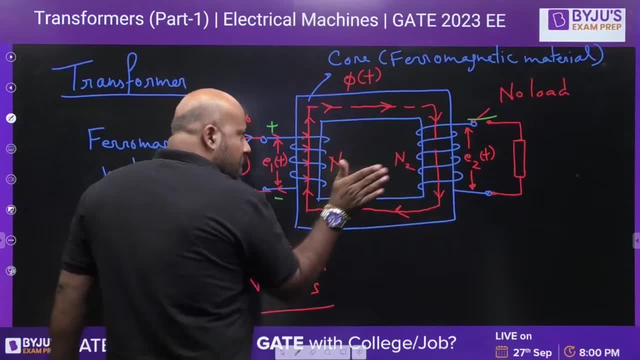 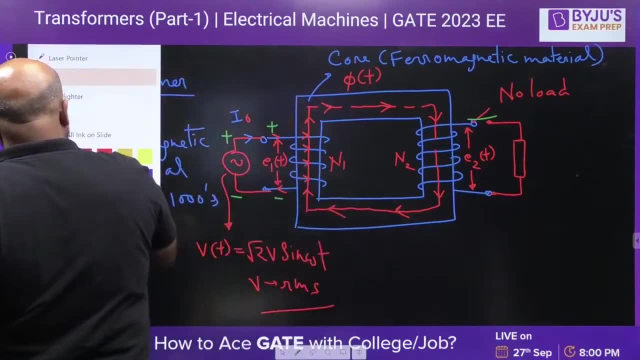 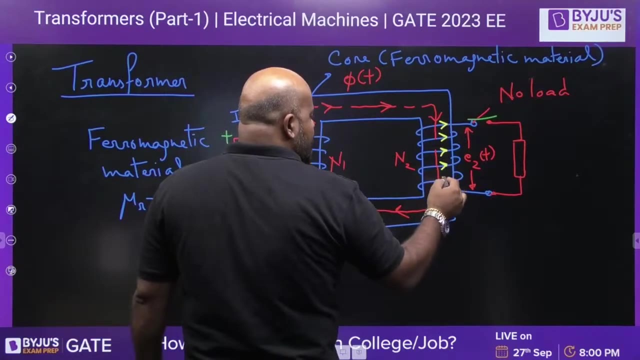 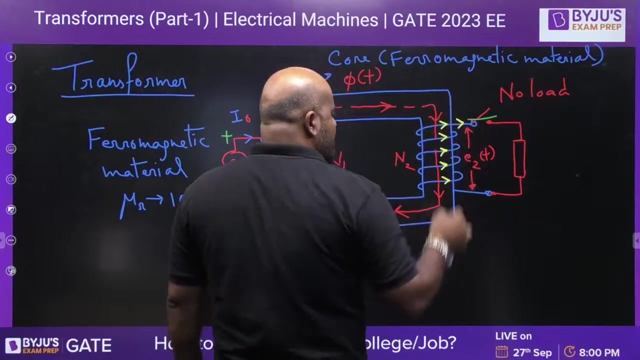 bottom to top, thumb in the direction of flux and fingers moving. fingers moving will give you the direction of current. it means the current is going to be something like this. the current is going to be something like this: yes or no, are you getting this or not? so if current direction is going to be like this, it 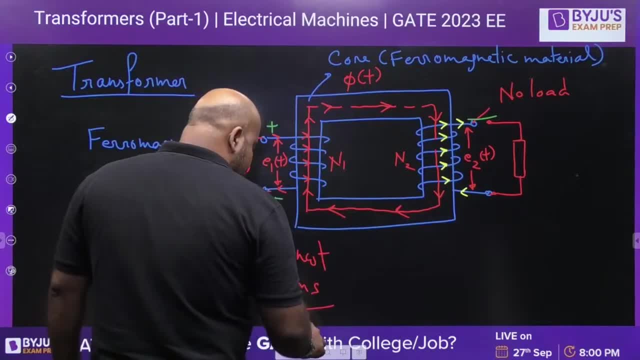 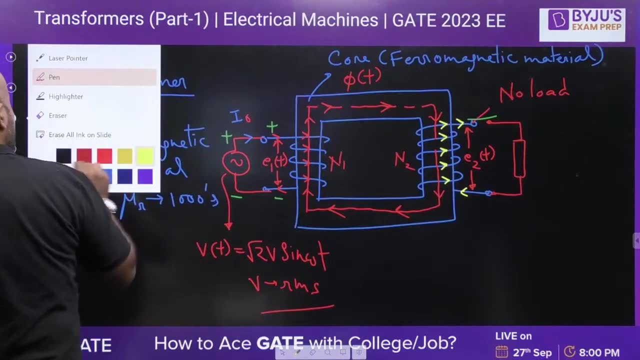 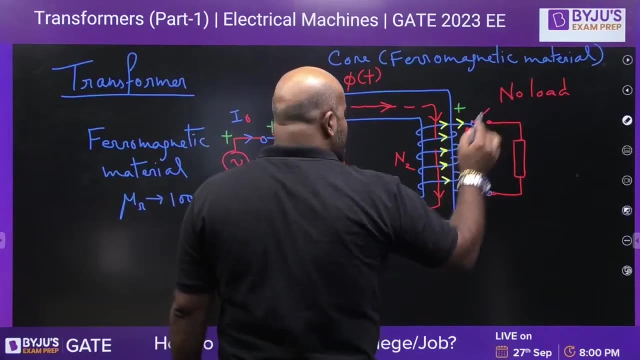 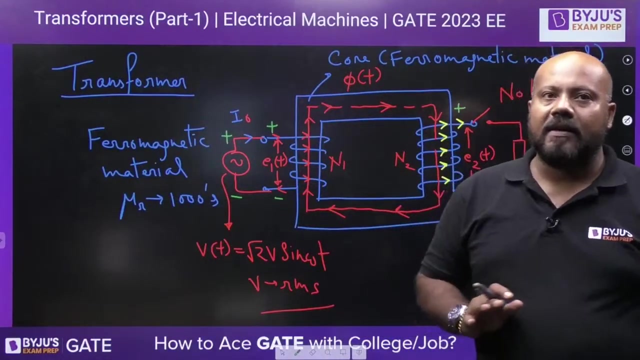 means what the polarity of even sorry e to the polarity of e 2 is going to be: plus here, minus here you. you just tell me yes or no. everybody just tell me this polarity of e 1 and e 2 is very important. you may get a direct question in the gate examination. 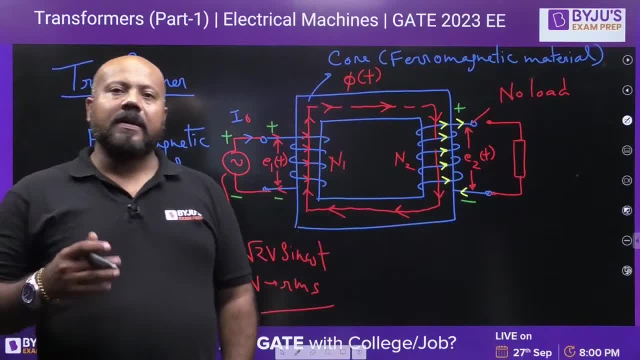 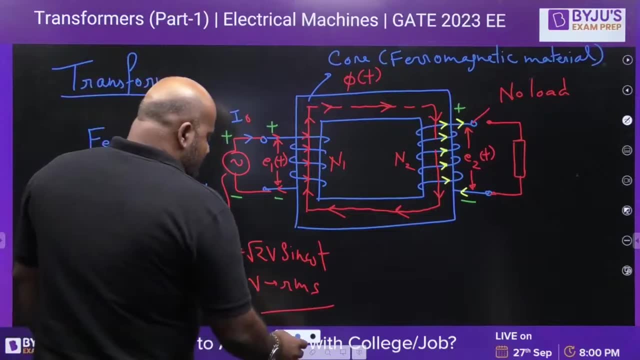 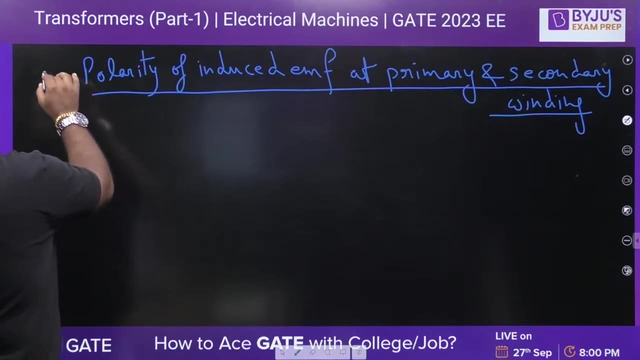 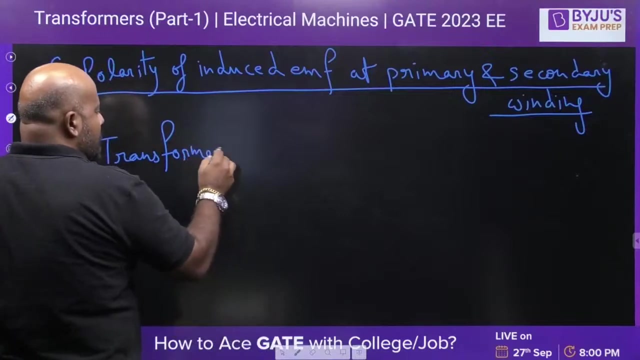 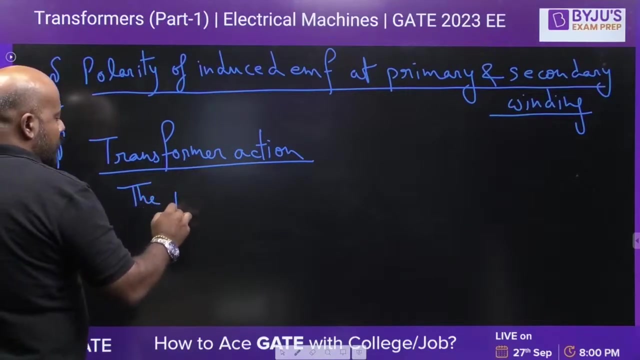 deciding the polarity of e 1 and e 2, and there may be multi windings also. is it clear now see, now see what is happening for transformer action, for transformer action, for transfer. this is the first thing. second thing: for transformer action, for transformer action, for transformer action, the primary and the 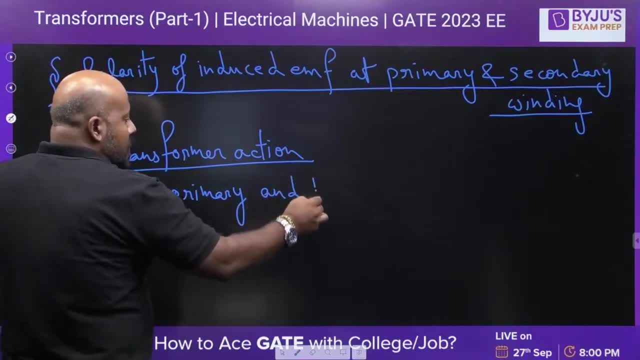 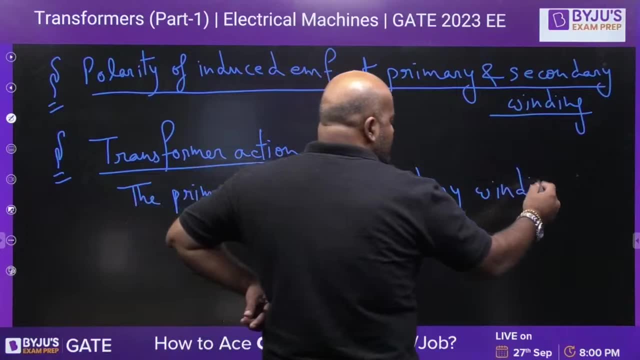 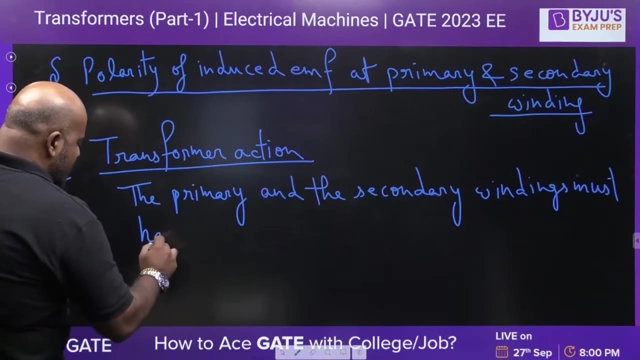 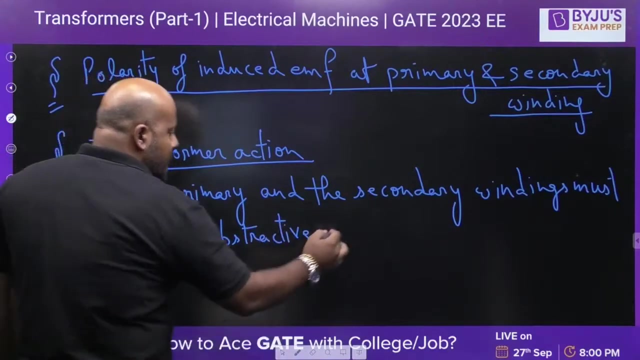 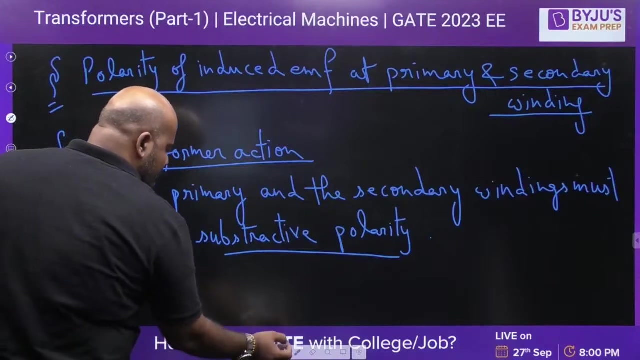 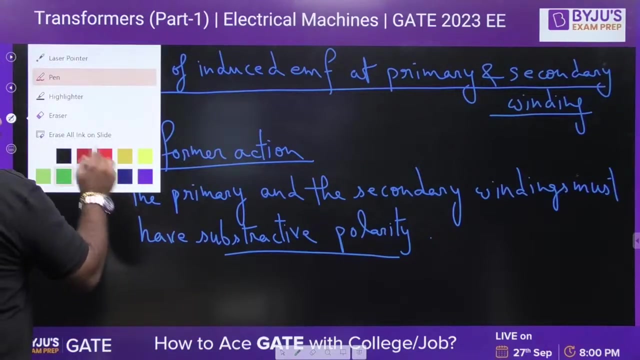 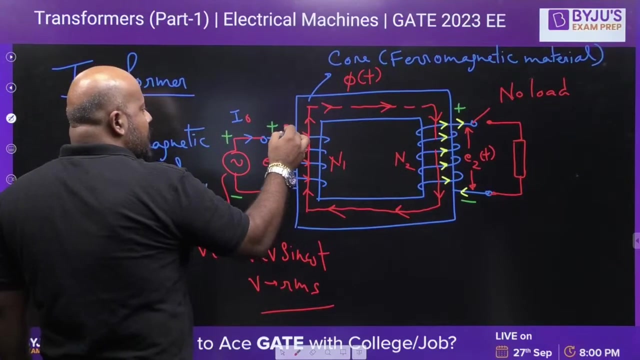 secondary windings. secondary windings means must have, must have subtractive polarity, subtractive polarity, subtractive polarity means what Substractive polarity means what Substractive polarity means what? Yes, It means if the current is going to enter the dot, if the current is going to enter the dot in. 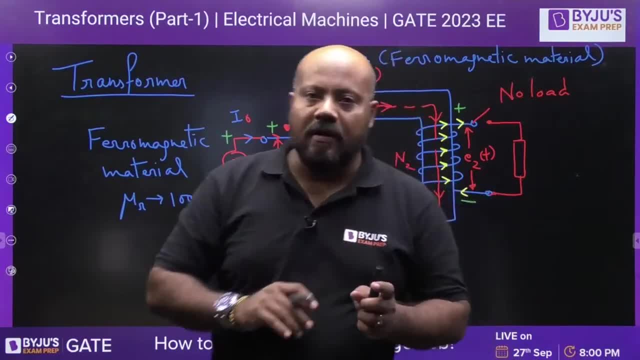 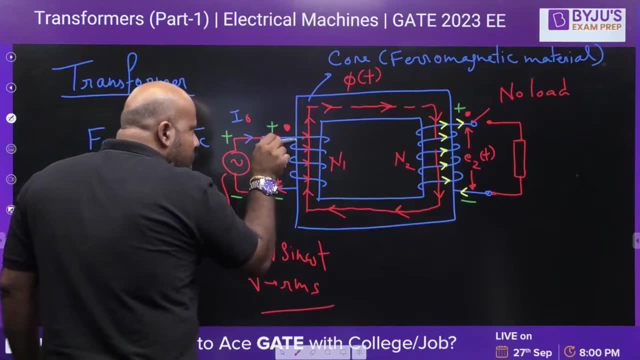 one winding, then the current is going to leave the dot in the other winding, then the current is going to leave the dot in the other winding. Can you see this? Current is entering the dot. current is leaving the dot. Is it clear for everybody, Are you? 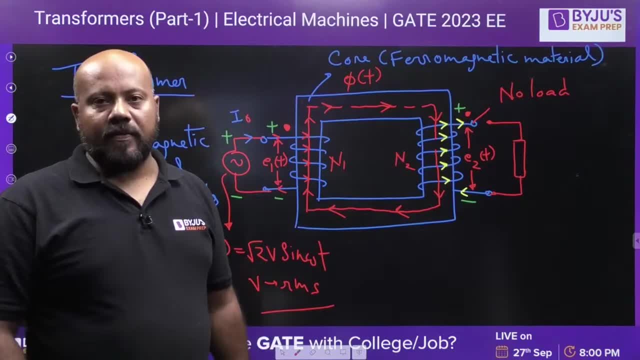 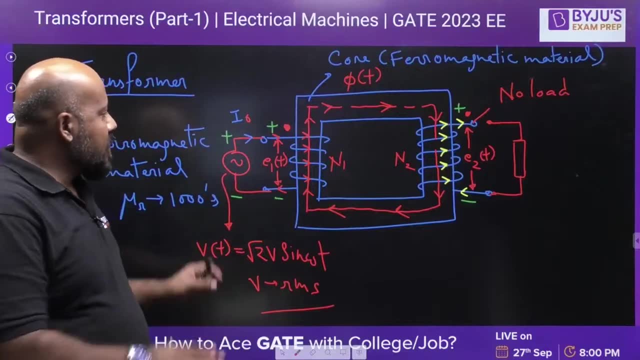 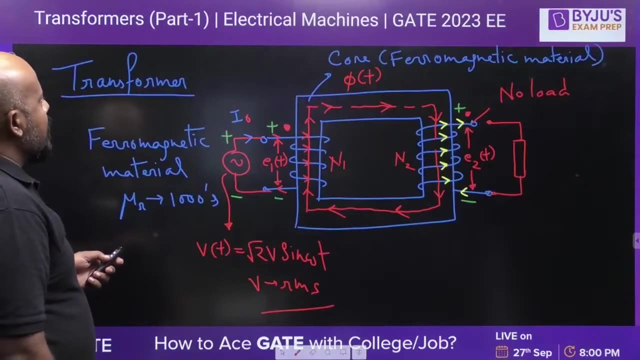 able to follow this. Say yes or no. Say yes or no, Yes, Murali. So this is clear Till now what we have said. Till now we have said yes, There was current I0 in the primary winding, because it is in the primary winding. 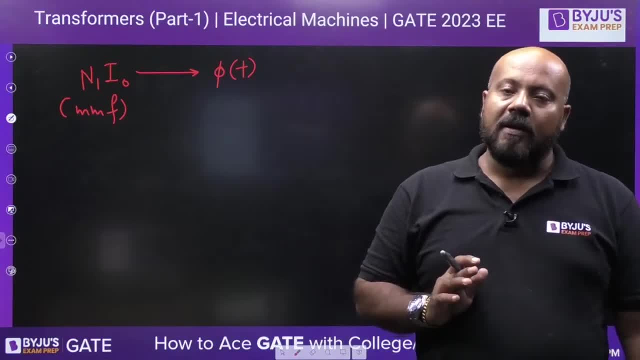 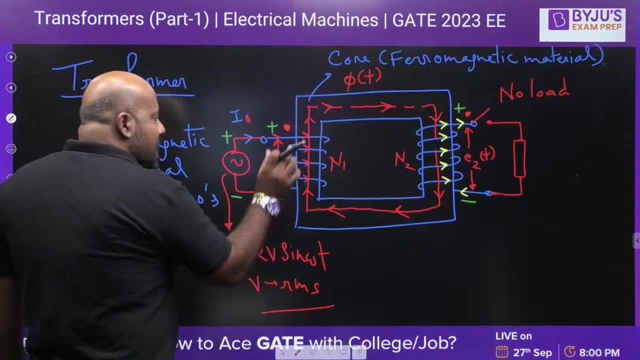 We know what is the final current. It is in no-load condition. So we are saying it is I0, no load current. Because of no load current flowing in the primary winding having n1 number of turns, the MMF developed in. 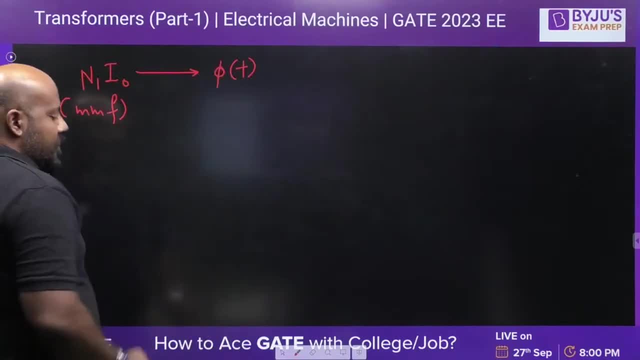 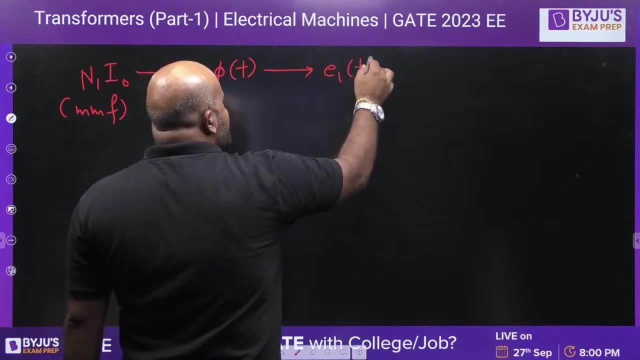 this primary winding is going to be N1–I0.. This N1–I0 will give rise to what E1 ≤ and E2 ≥…. Yes or no one is saying Yes, It is because the number of turns, This number of turns, what E1.. 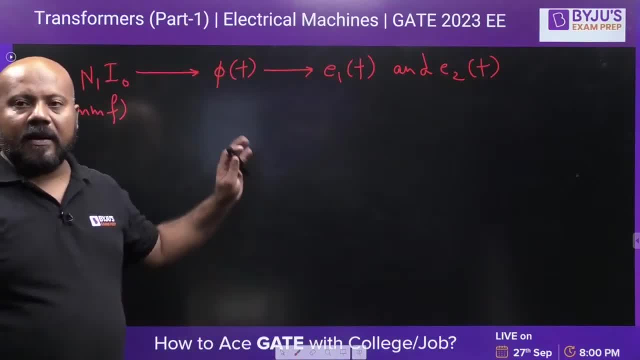 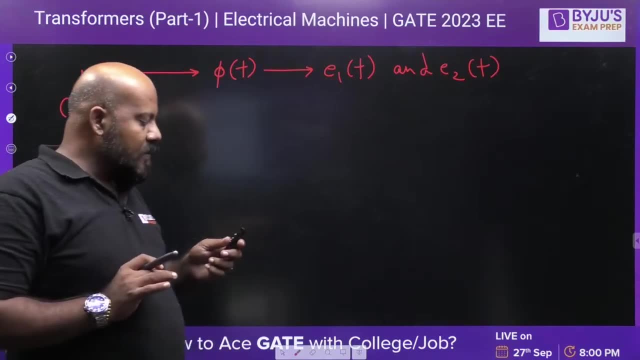 Yes, place that in the T0 section and it will speak G1 over E2.. The MF wouldn't it? yes or no. this much is clear now. this is the case when the transformer is not connected to the load, when the secondary winding load is not connected, is it? 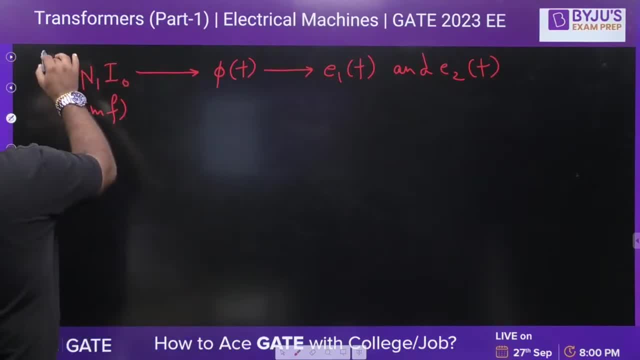 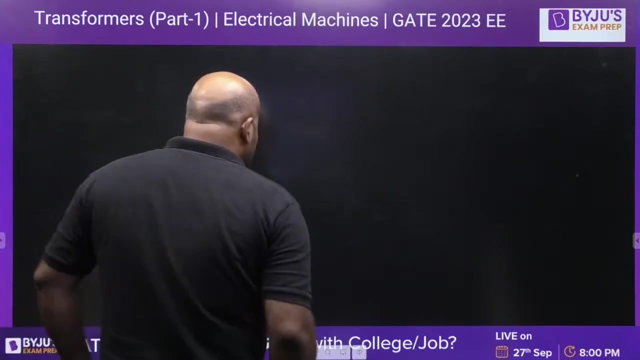 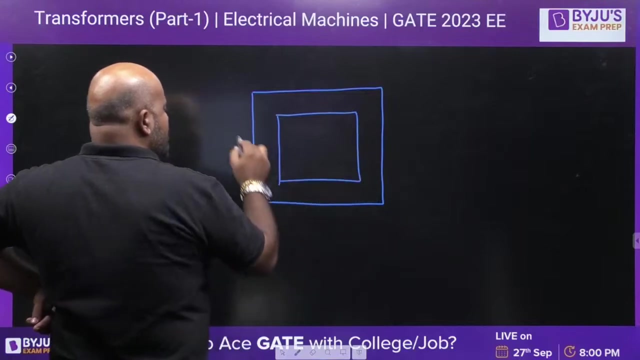 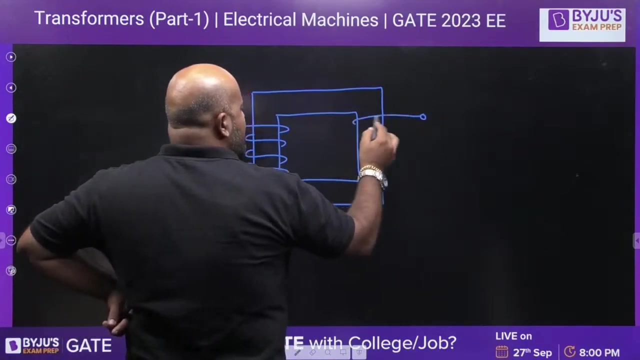 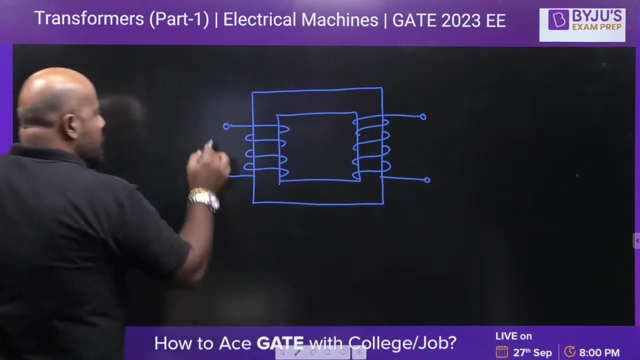 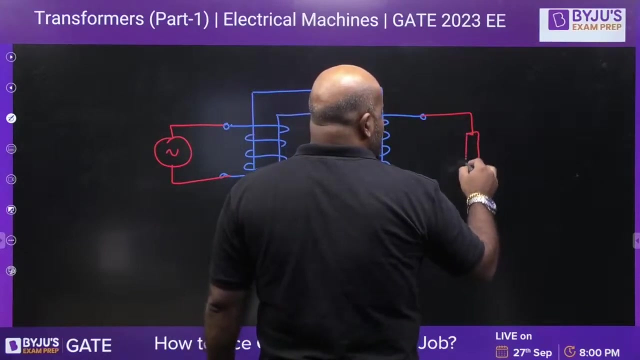 clear now. this is the no load condition. suppose second on load condition. now we are going to connect the load in the transformer. what will happen? what will happen? everybody see here: primary winding, secondary winding. you are connecting a source at the primary side and you are connecting a load at the 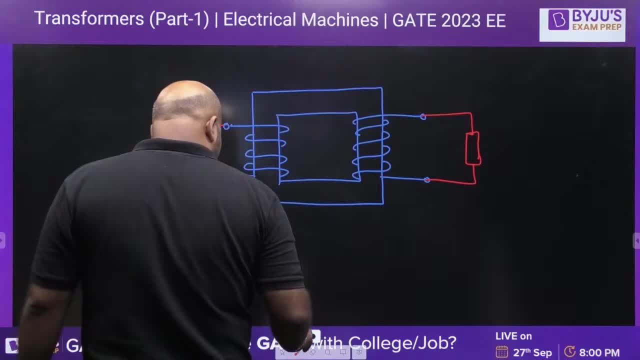 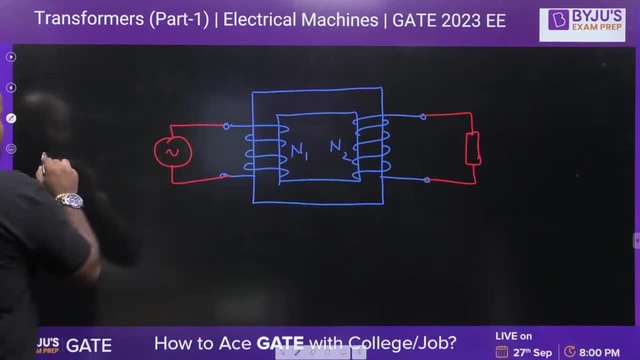 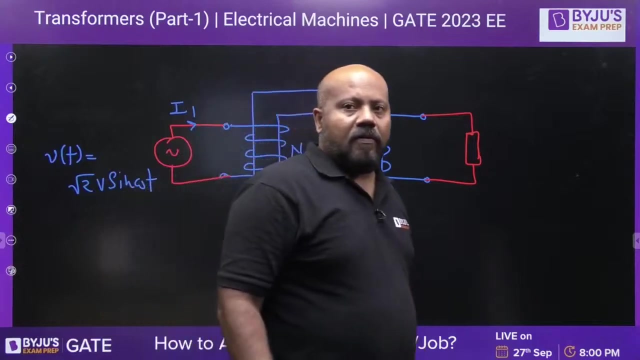 secondary side. number of turns are going to be n1 here. number of turns are n2. now again, the source VT is root to be sine Omega T current. here is i'm writing the rms value. suppose this is i1. suppose this is i1. why I'm writing I, when I will tell you. please have some patience. 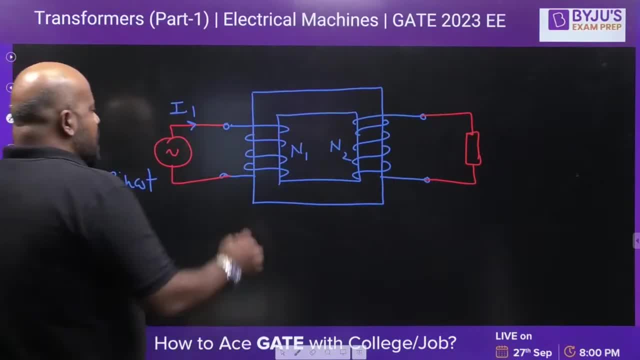 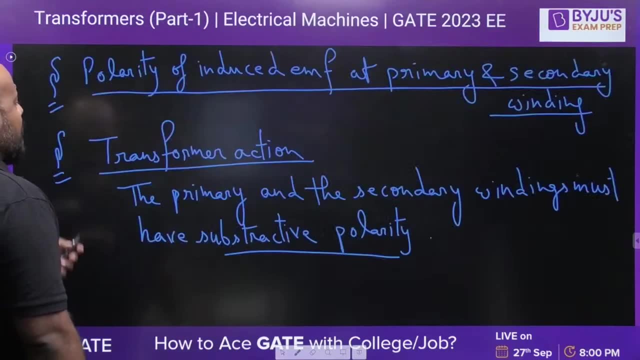 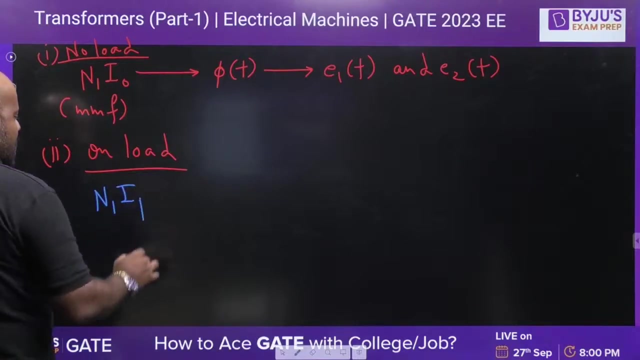 why I'm writing? I when I will tell you now, this current flowing in, this winding, what will happen. it will give rise to an MMF. it will give rise to an MMF and that MMF is going to be what? and 1, I, 1. now this n, 1 I 1 is going to do. 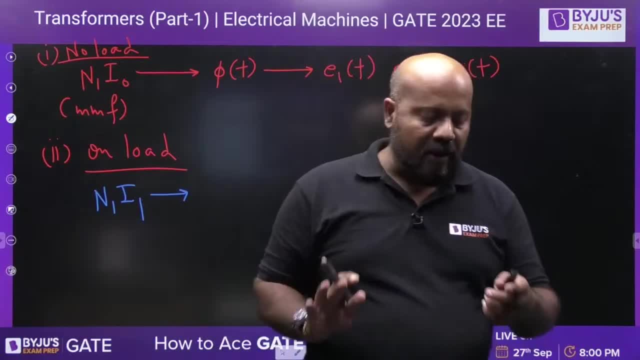 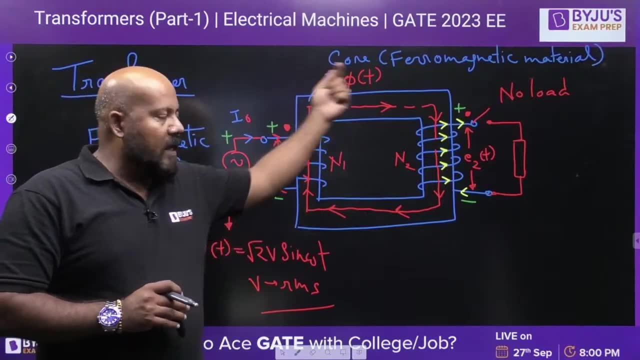 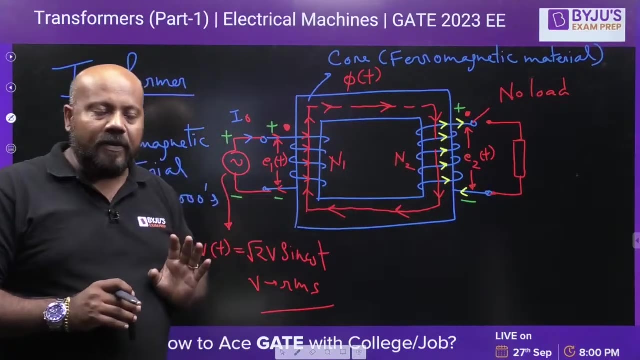 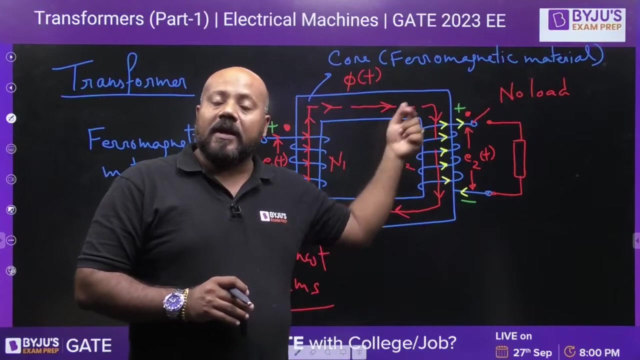 what this n 1, I 1 is going to do, what, please try to listen. already, because of the no load current, the flux was established, even an e to, even an E to. they were already induced or developed. the moment you have closed this switch, what will happen? this EMF e to will circulate or slow its current, that is. 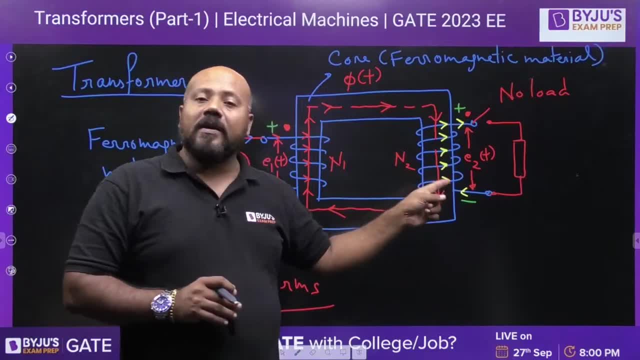 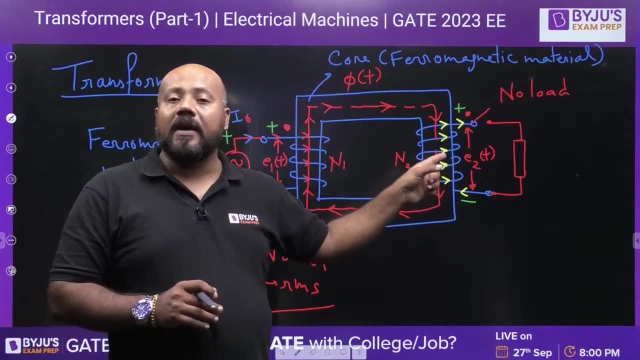 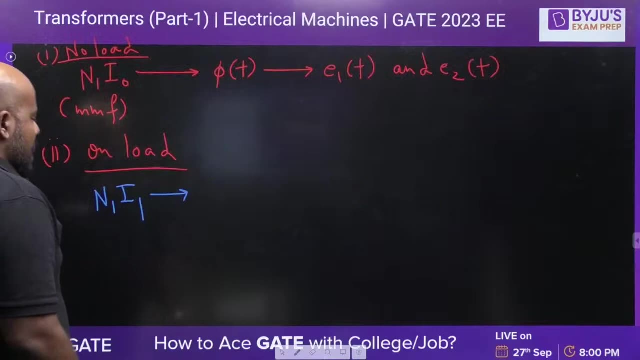 I to the moment. current is start flowing in the secondary circuit. there will be some MMF developed in the secondary winding. that is going to be you N 2 I 2.. That is going to be N 2 I 2.. Yes or no? Yes or no. N 1 I 1 gives rise to establishment. 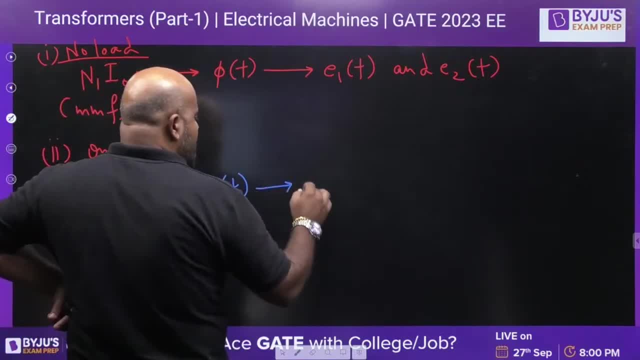 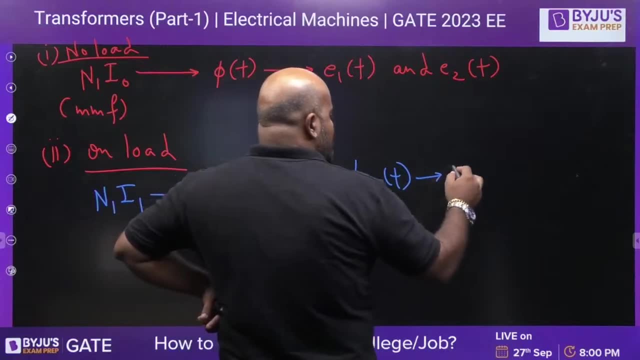 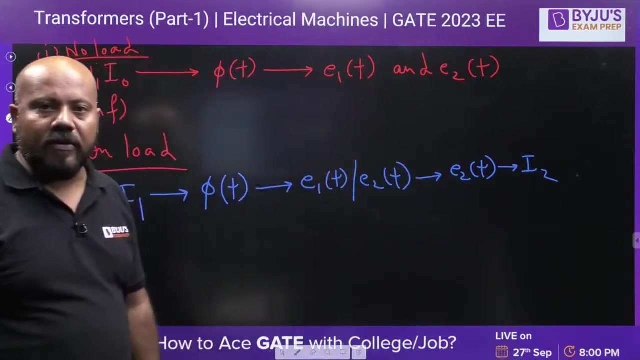 of flux Already. flux was there Then because of E 1 T and E 2 T. E 2 T will develop current I 2.. Yes or no, E 2 T will develop current I 2.. This current I 2 will give rise to MMF. 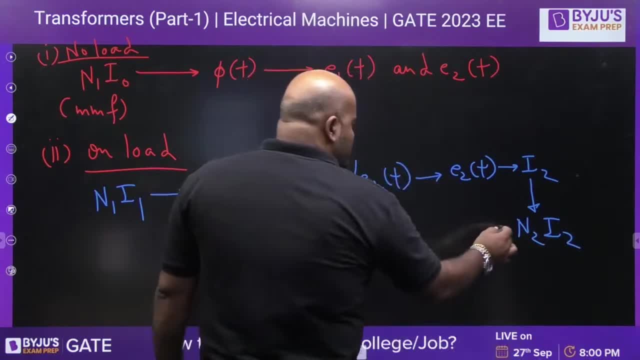 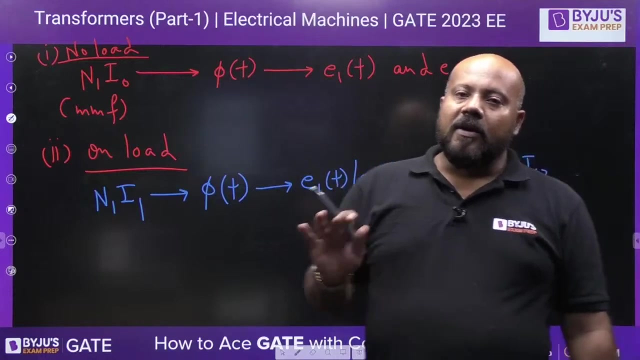 N 2 I 2.. This N 2 I 2 will try to oppose the flux. Oppose the flux Now. very important lesson for all of you in your life. Very important lesson: You can never, ever, change anything in your life. 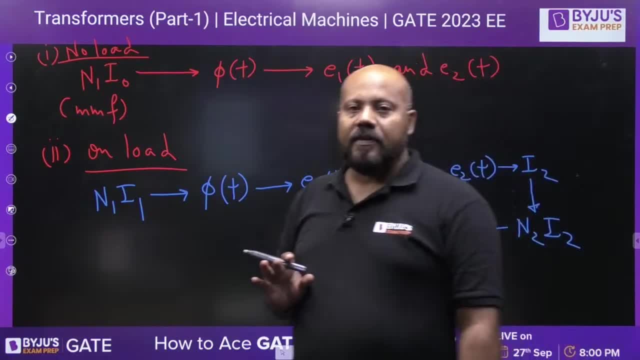 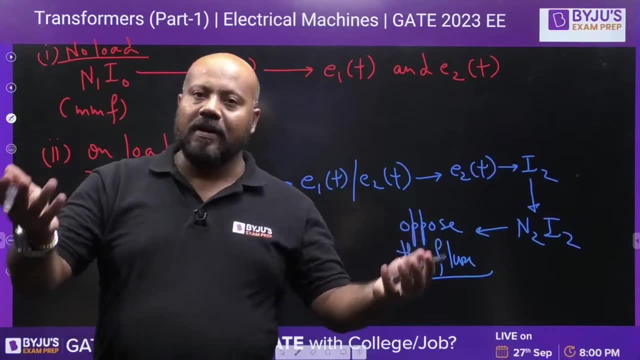 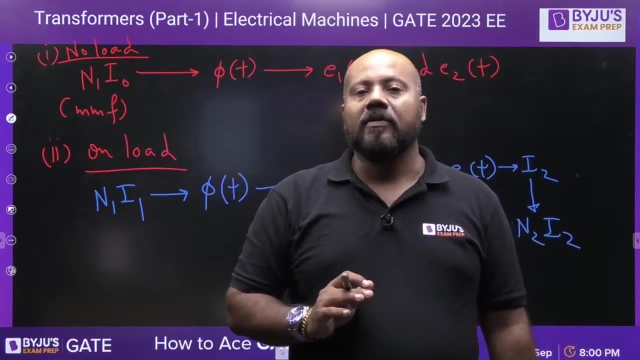 That you do not control? Can you change when the gate examination is going to be conducted? Can you change the date? You can think of, You can dream about it, But you cannot change. Can you change the way gate examination paper is set? No, Because it is not in your hand. 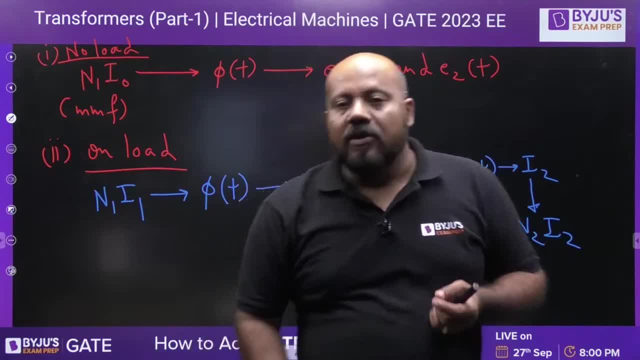 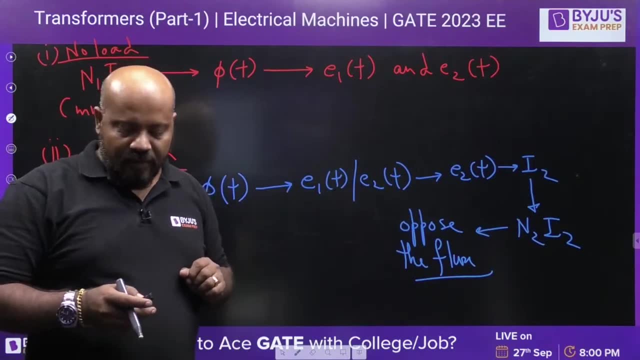 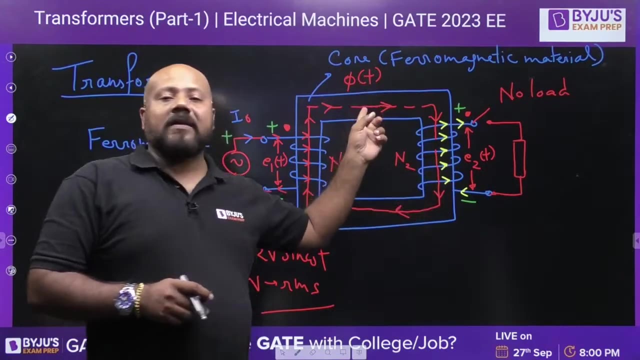 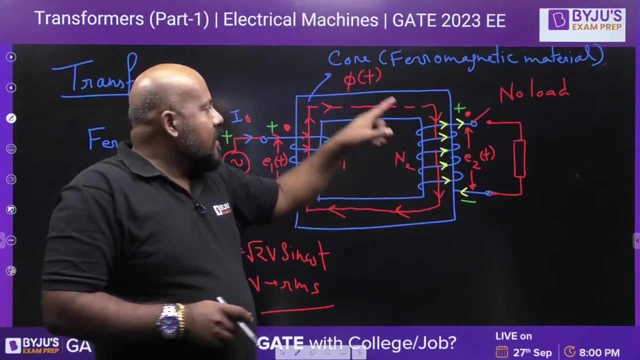 Yes or no. So when this flux is not controlled by you, how you can change the flux, Yes or no? It means the MMF in the secondary winding is opposing the flux in the core, But how it is going to reduce it. Why? Because this phi T is not decided by N 2, I, 2. This 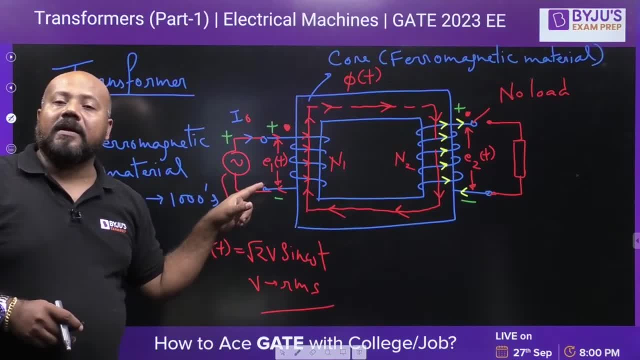 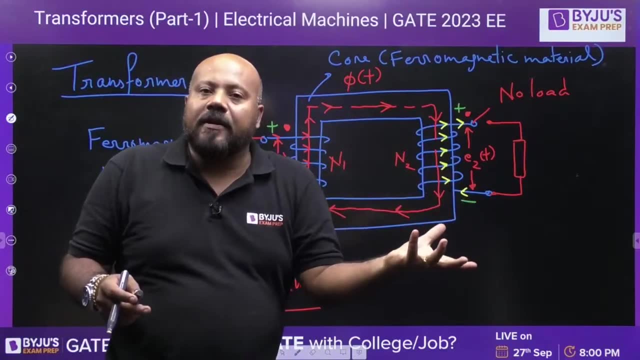 phi T is decided by the excitation or the current in the primary winding. It means what The secondary MMF has to be anyhow compensated. Now who is going to compensate this MMF at the secondary winding N 2, I, 2.. 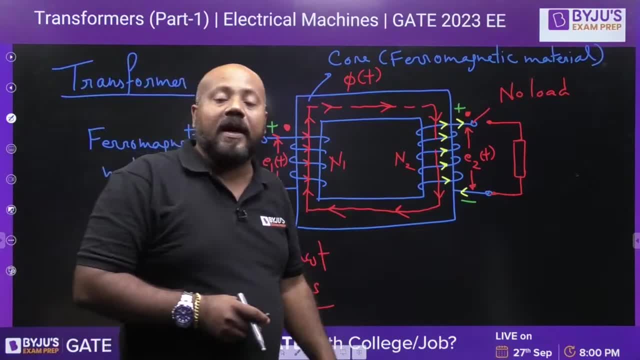 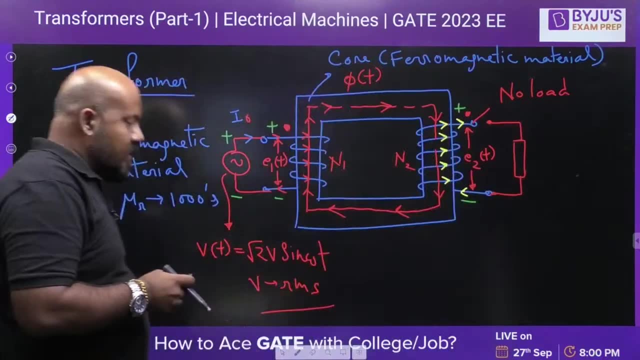 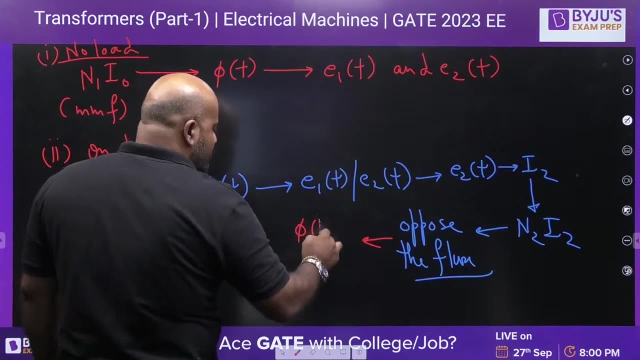 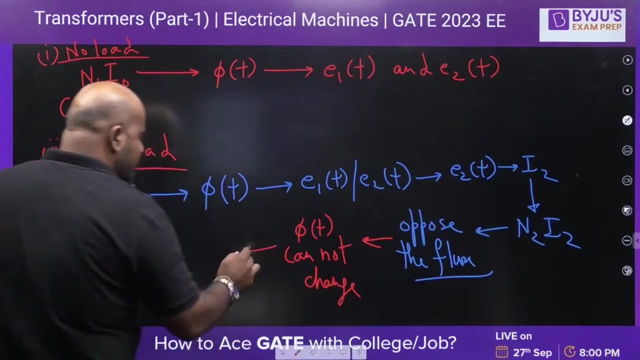 Only the source connected at the primary winding is going to compensate the MMF at the secondary winding. Hello, Are you able to follow this? Are you able to follow this? everybody, Are you able to follow this? Phi T cannot change. So what will happen? Extra current. 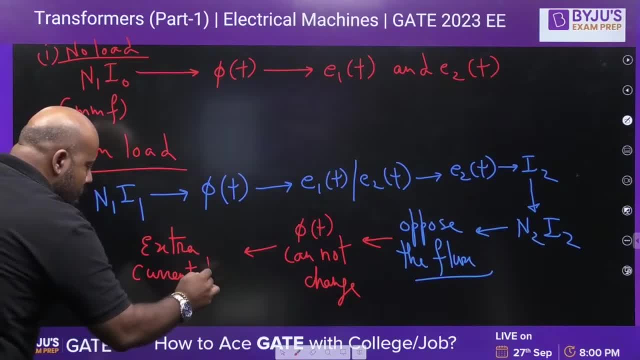 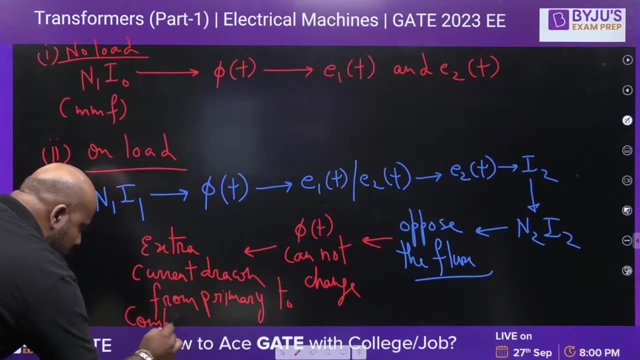 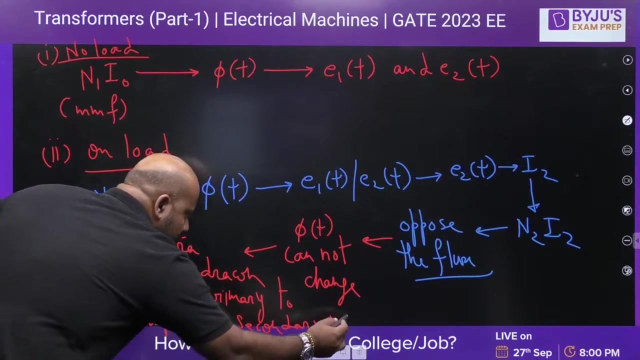 Drone from primary to compensate secondary MMF. I hope you are able to follow this. So this I 1 is not actually a monocular, It is a monocular. So this I 1 is not actually a monocular. It is not a monocular, It is an integral. 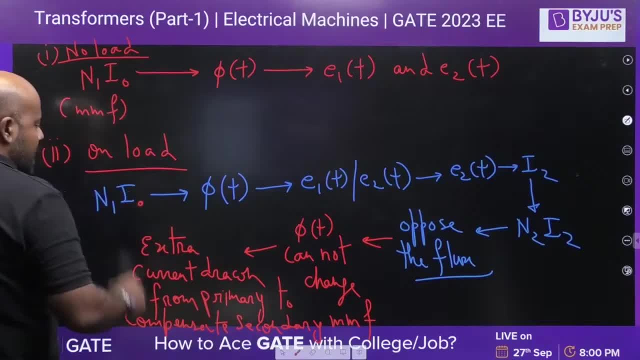 i 1. right now it was n 1, i naught again, but now it has become i 1, which is i naught, plus i 2 dash. what is i 2 dash? i will tell you what is i 2 dash. i will tell you what is i. 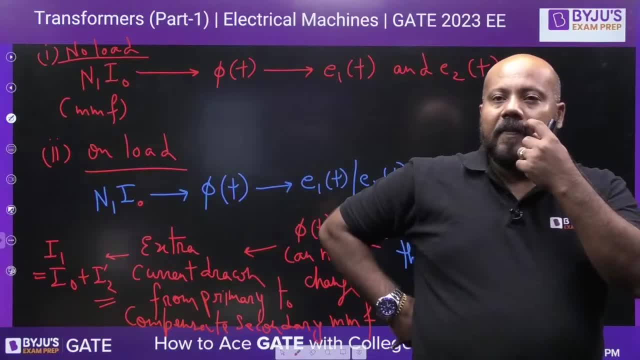 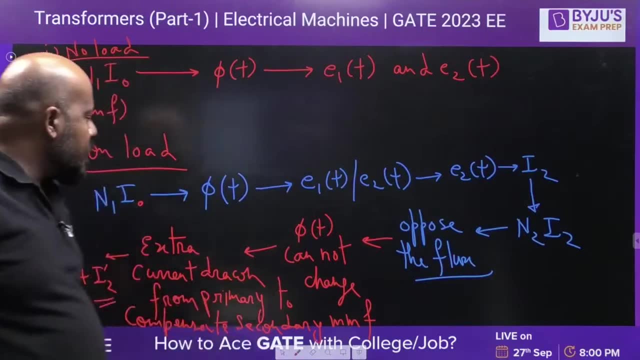 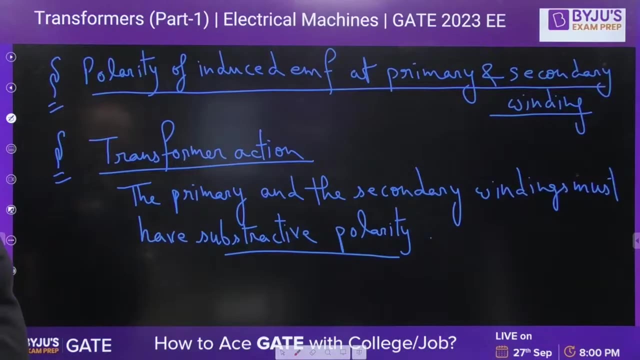 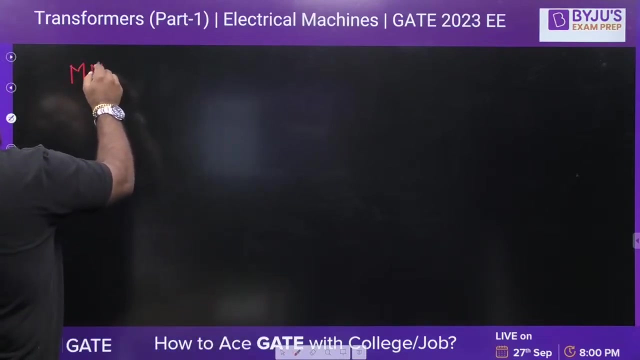 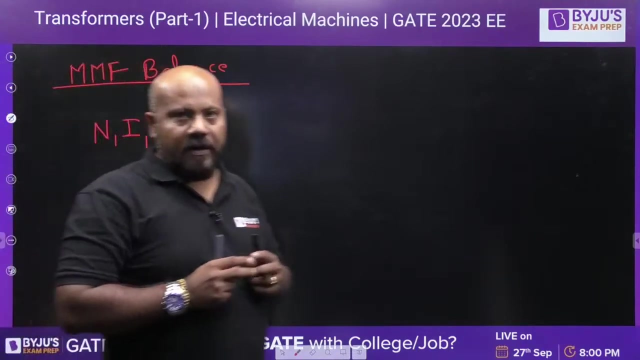 2 dash. i will tell you, mr gate 2027 aspirant, listen here now. what is this mmf balance? what i was telling you, please try to understand if you write the mmf balance equation. now, that is the main concept of transformer. okay, mmf balance. i am writing primary winding. mmf is n 1. i naught. it has two responsibilities. 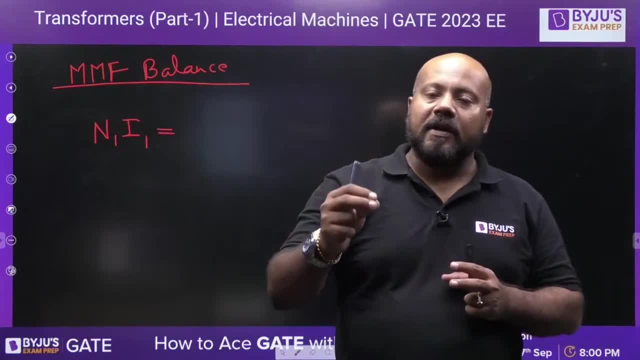 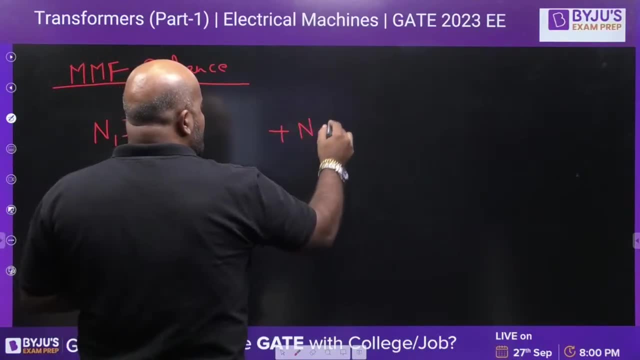 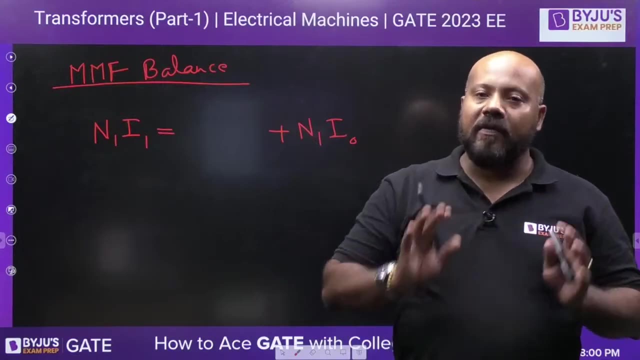 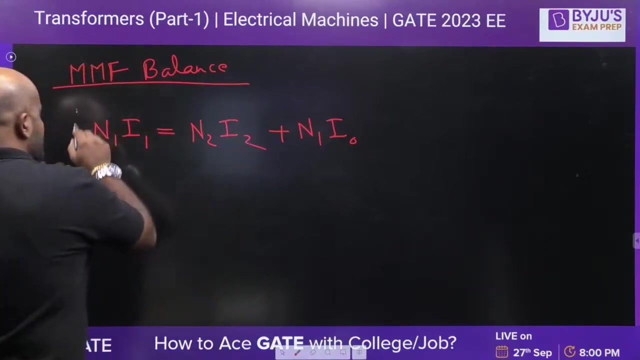 it has two responsibilities. one responsibility is to establish the flux in the core. that responsibility is n 1, i naught. it has another responsibility to compensate for the secondary winding mmf n 2 i 2. and that is how it is doing: n 2 i 2. everybody just tell me can you write this equation? everybody just tell me, can you. 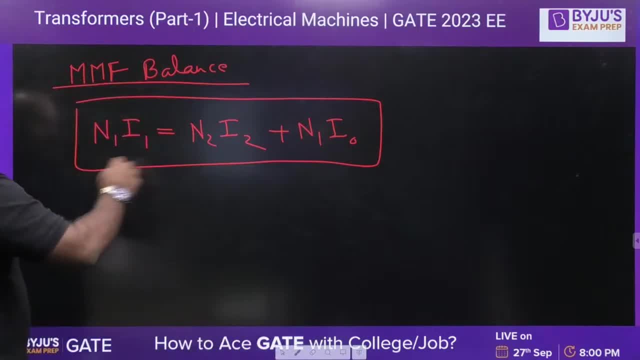 write this equation. and if you can write this equation, divide this whole equation by n 1, so you will be getting i 1 as n 2 upon n 1, i 2, plus i naught this n 2 upon n 1, i 2 we. are defining as n 2 upon n 3. i naught, i naught then this: n 2 upon n 1. i 2 we are defining as n 2 plus i shrine, which is n 2 minus Taylor series. the n 2 in square p is equal to n one. what this n 2 right to direction i 1. is with the point denoted by in one and n 2 and this n 2? why have you registered here n 1 plus n 2, all points, i, two, x, and this is by Professor sir as wel valer. 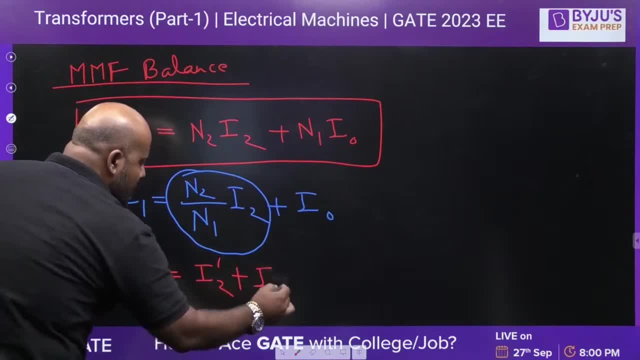 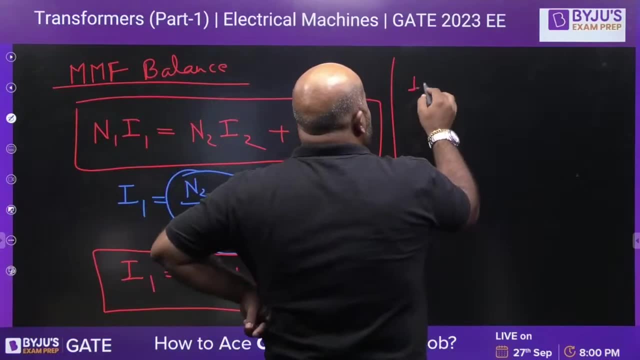 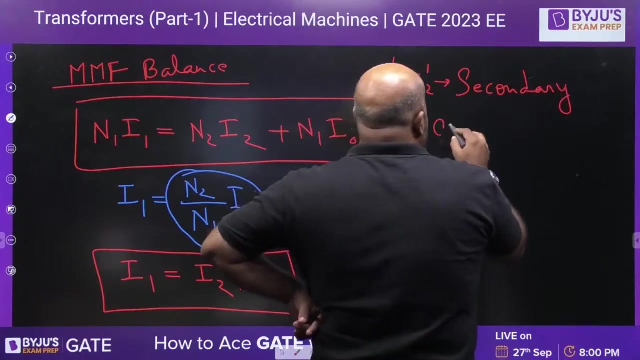 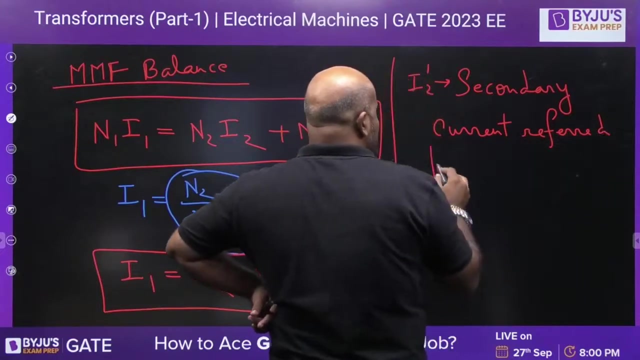 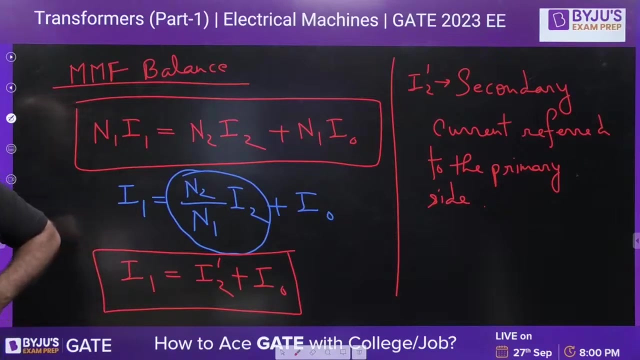 I2 dash plus. I naught Now. what is this I2 dash? What is this I2 dash? It is the secondary current. It is the secondary current referred to the primary side. Secondary current referred to the primary side. Everybody just tell me, are you able to follow this After this? I 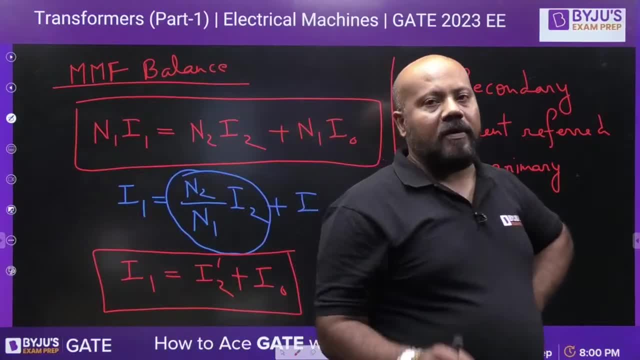 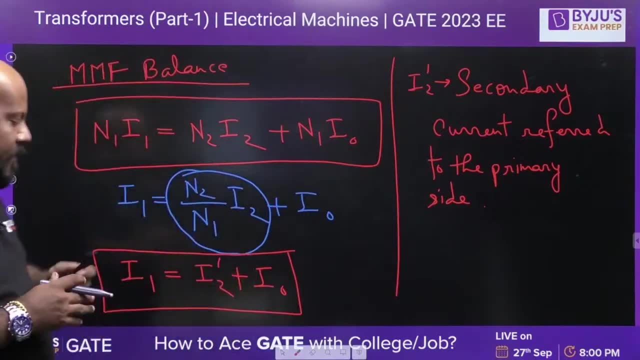 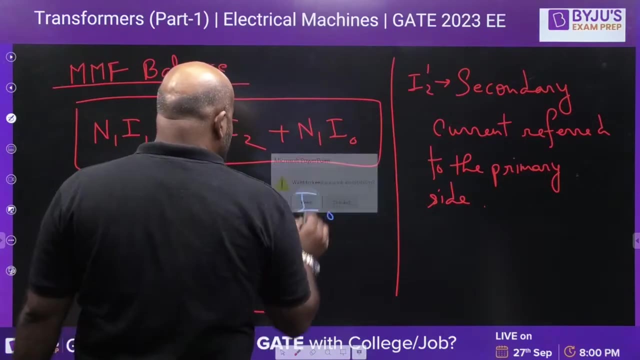 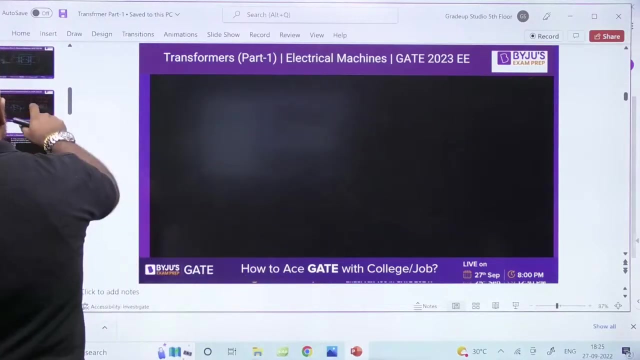 will be just giving you a brief idea about the current Transformer equivalent circuit and then we are going to discuss the questions. I hope it is sufficient for the time being. Just give me a moment. Just give me a moment, OK, OK. 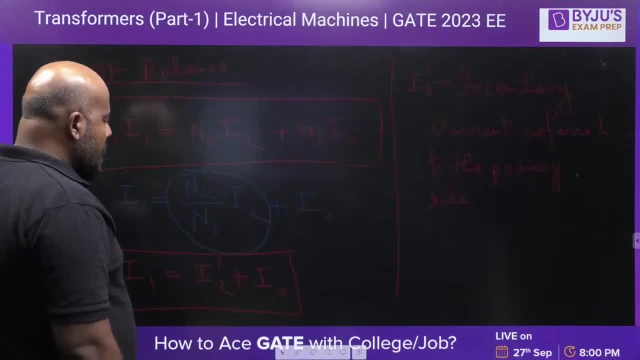 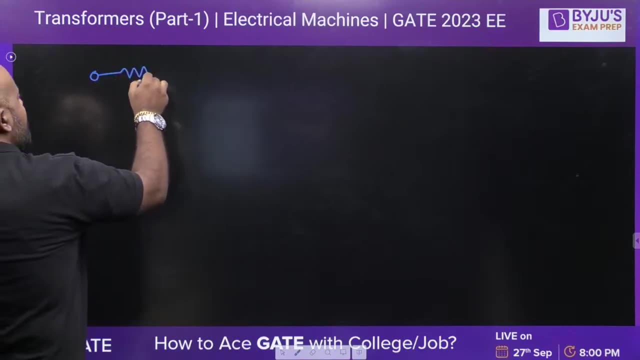 So how we are doing the equivalent circuit of our transformer. Just see here: This is our transformer, This is our transformer. The most simple representation of transformer is this. It is a two winding transformer. suppose this is primary side. current is V 1, voltage is: 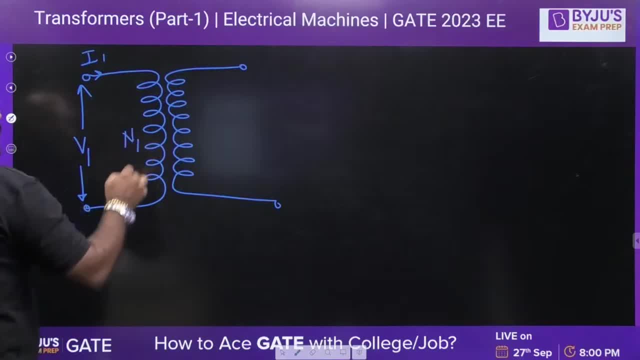 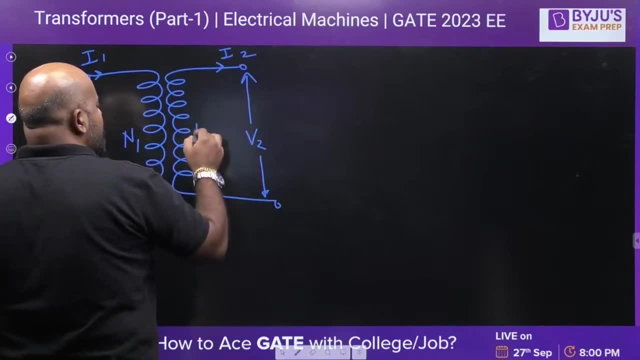 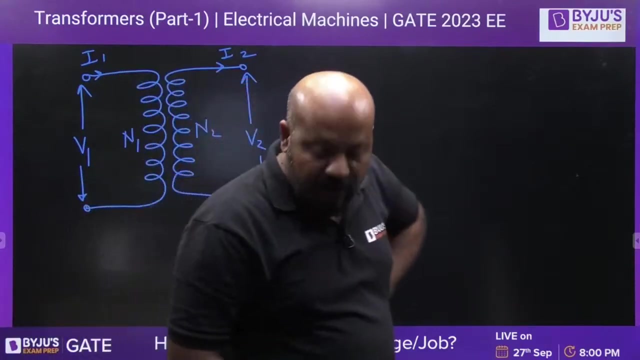 V 1. current is I 1. number of turns is N 1.. Again here, secondary side voltage is V 2. current is I 2. number of turns is N 2. ok, Now see what will happen. If you talk about a practical transformer in a practical transformer, we are going to. 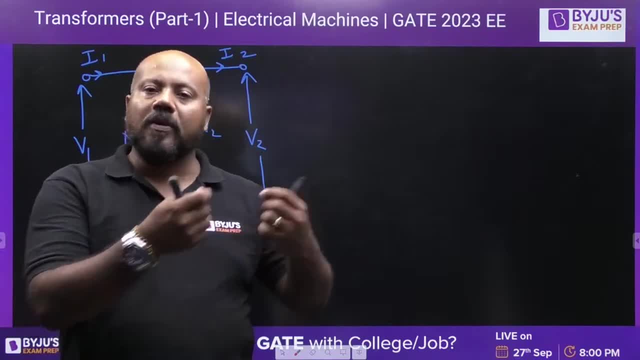 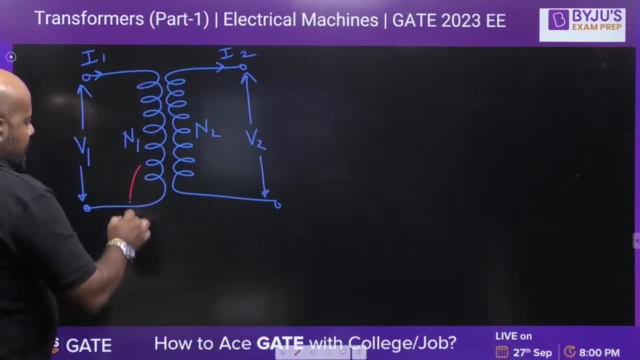 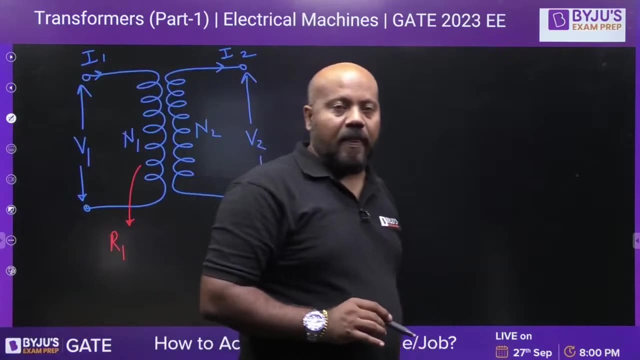 draw the equivalent circuit. equivalent circuit is nothing, but you are going to model your transformer because you want to analyze its performance or working. Now please try to understand this winding. this winding is going to have R 1 resistance. Why R 1 resistance? This R 1 resistance of the primary winding is going to represent what I square R losses. 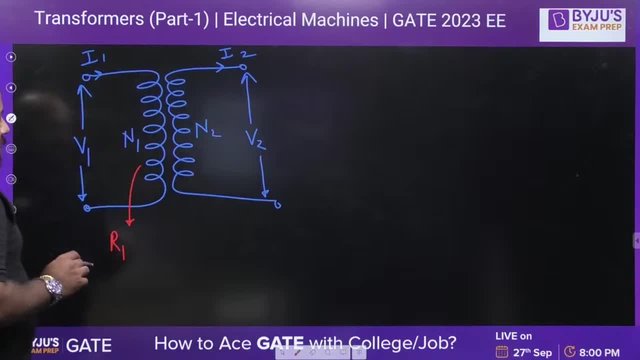 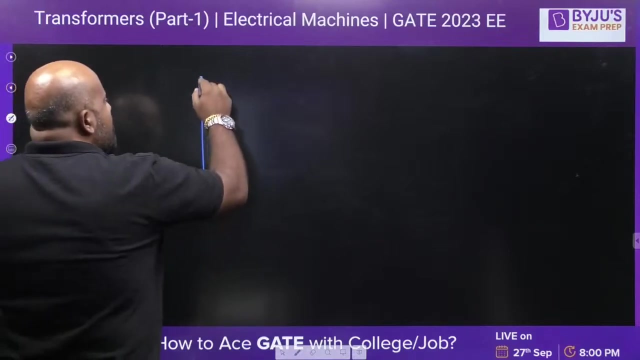 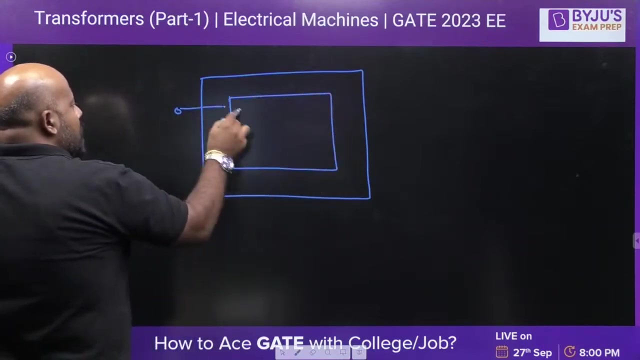 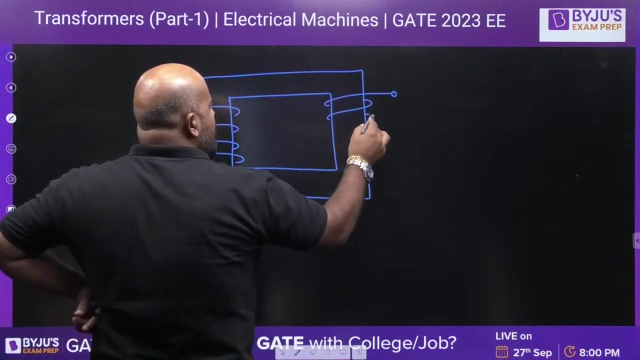 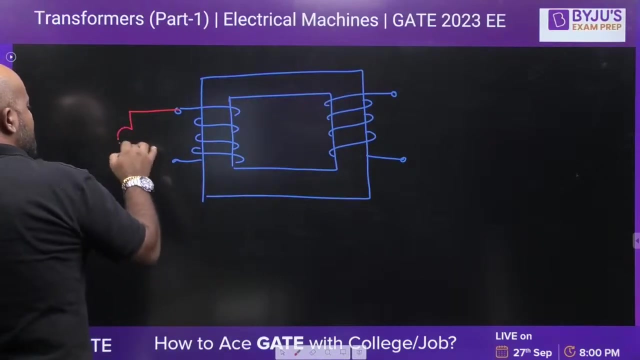 in the primary, That is, the copper losses, Then we will be having leakage reactance. this is leakage reactance. What is leakage reactance? What is leakage reactance? What is leakage reactance? Suppose this is your transformer. This is your transformer. ok, here you have connected the source. here you have connected. 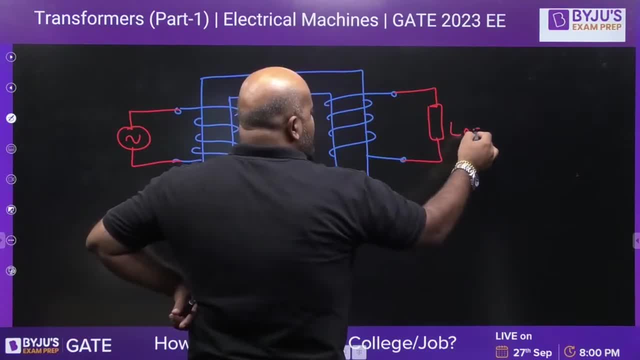 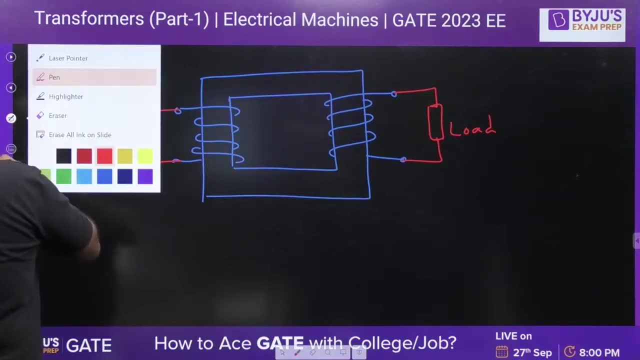 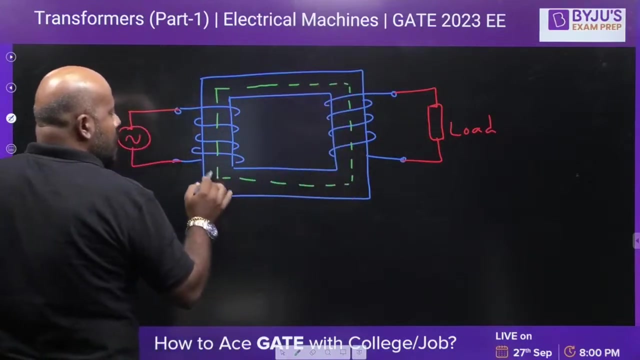 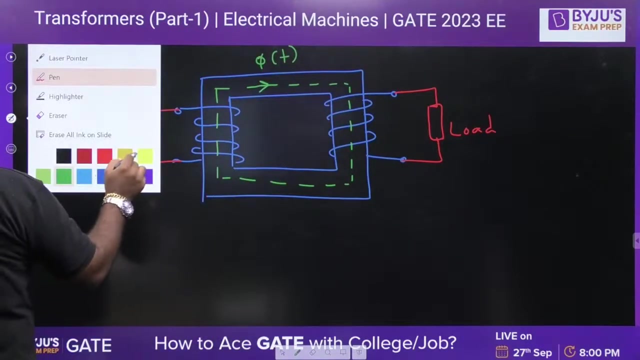 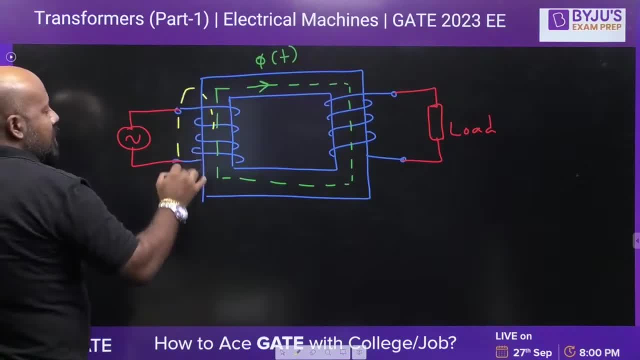 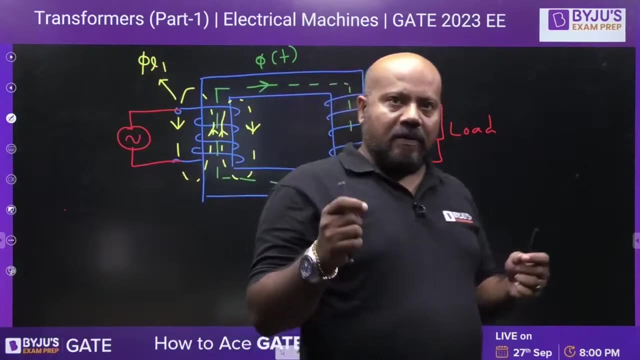 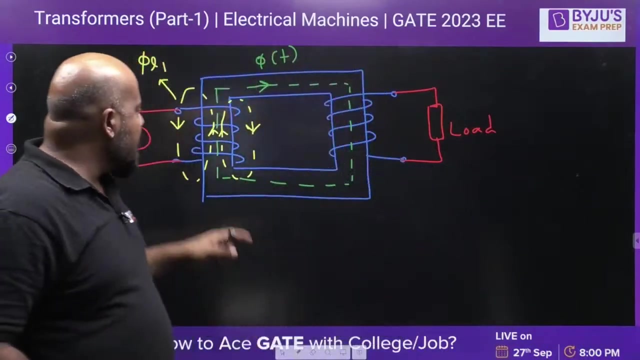 There will be some flux. There will be some flux. Phi l1 information ır. There will be some flux. There will be some flux which is going to be linked only with the primary winding, not with the secondary winding. This flux we are defining as the leakage flux for primary winding. 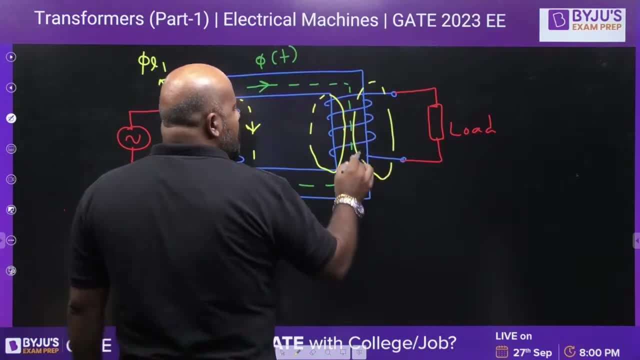 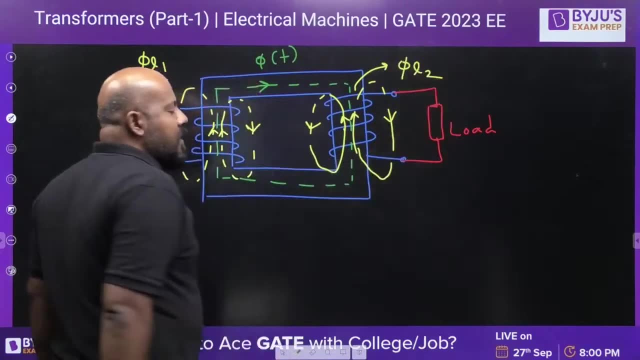 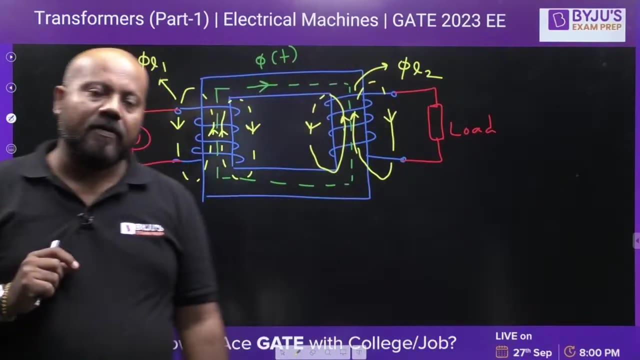 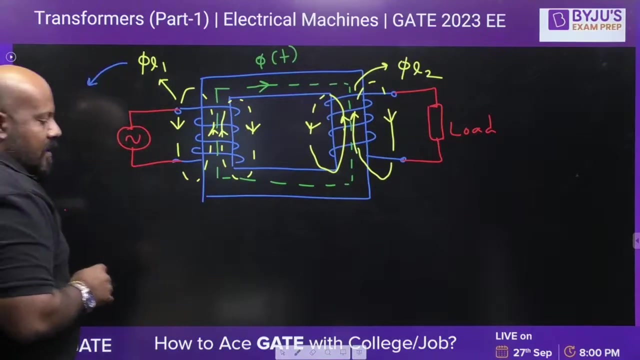 Then we will be having some flux which is going to be linked only with the secondary winding and not with the primary winding. This is what we are calling as the leakage flux for the secondary winding. Yes, Ramesh, from air path. Now, this leakage flux at the primary winding is going to be modeled in such a way because 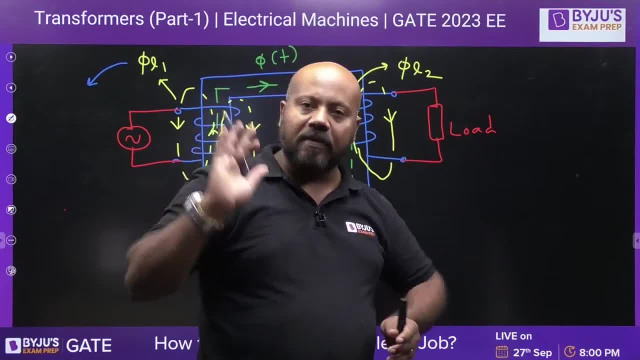 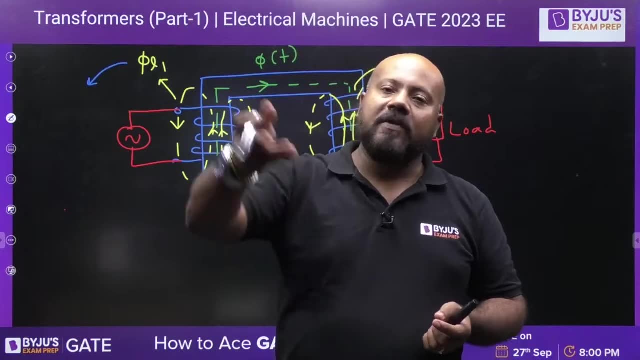 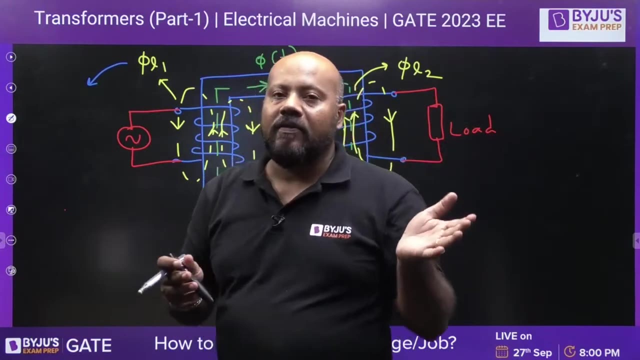 what flux is giving you Flux? is actually giving you induced EMF, yes or no? Primary winding or the secondary winding? induced EMF is d phi by dt Faraday's law, If some flux is leaked, if some flux is not linked with both the windings we are calling. 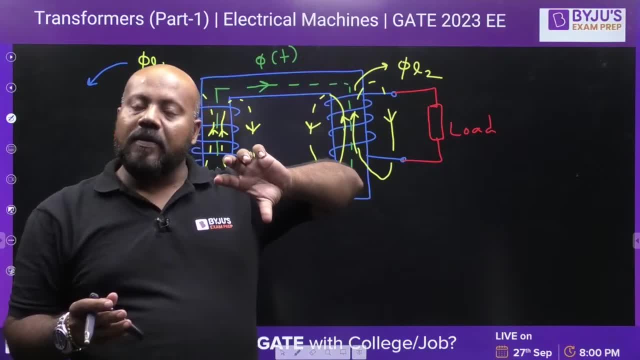 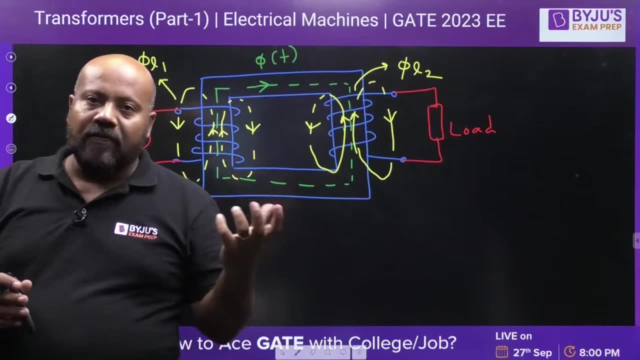 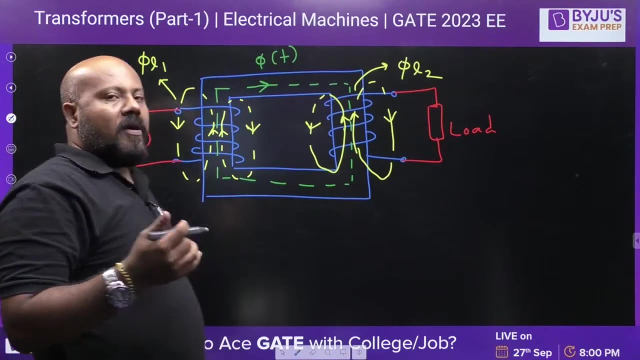 it leakage flux. So this leakage flux will be modeled in our equivalent circuit in such a way so that there is a drop in the voltage. So this leakage flux has the nature that it can be modeled in the form of a voltage drop. Now, voltage drop because it is the flux. 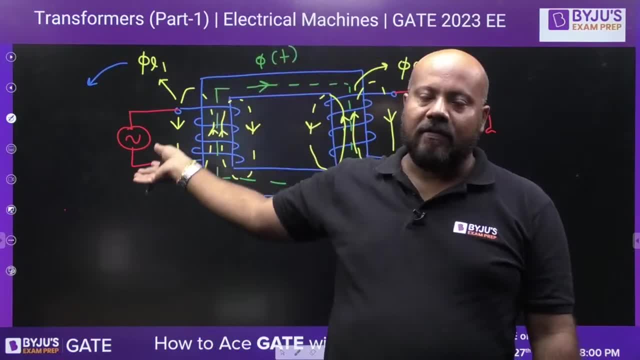 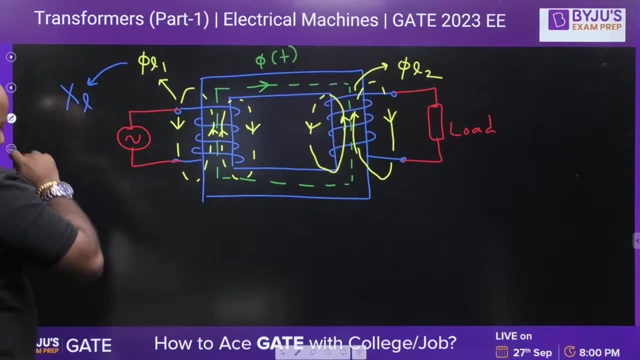 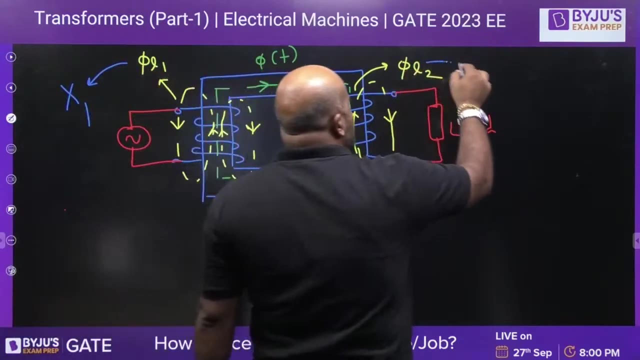 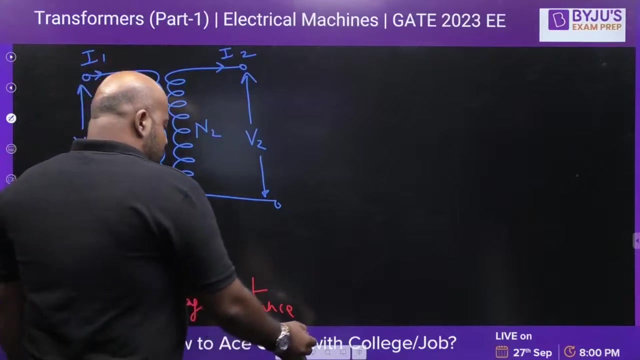 So we are representing this voltage drop because of this leakage flux as leakage reactance. So this will be represented as leakage reactance, or simply X1.. Similarly, at the secondary side, this leakage flux will be represented by X2. So this X1 and X2 is basically the leakage reactance. 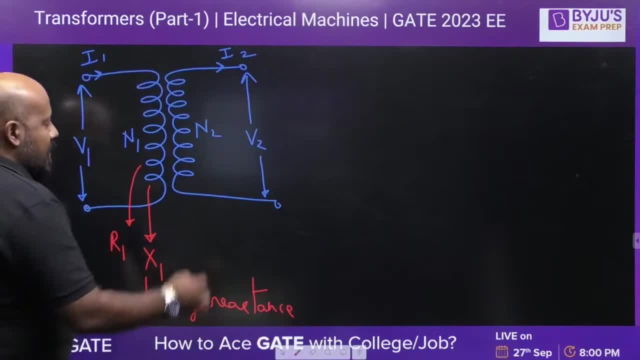 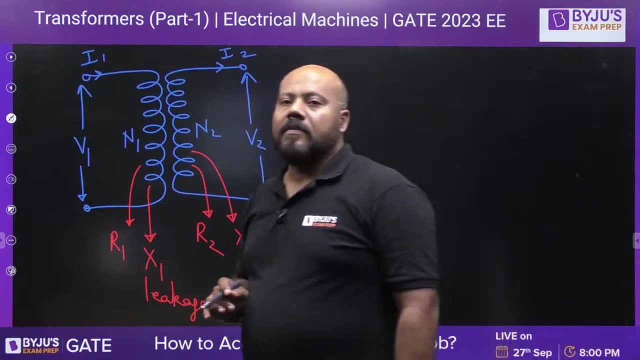 In the primary winding we have seen R1, X1.. Now at the secondary winding, there will be copper losses. R2 and X2 is the leakage reactance. Okay, Okay, Okay. So this is representing the leakage flux in the secondary winding. 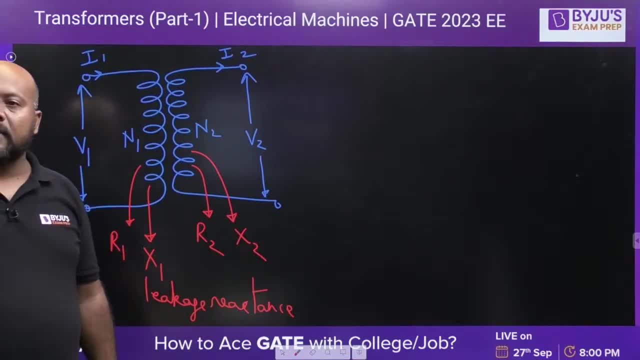 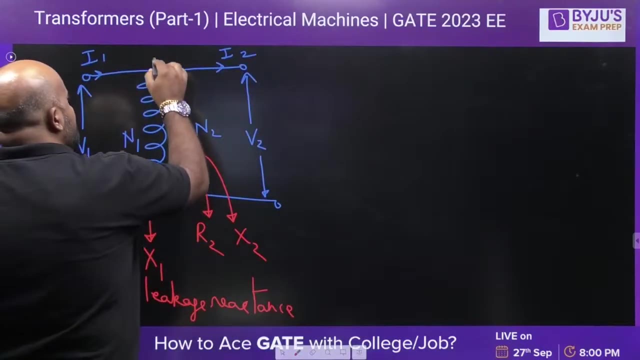 Yes, Karthik, please wait, please wait, listen. And in a practical transformer there will be two more components involved. The first component will represent the core losses, So Rc we are using to represent the core losses. And there will be one more component, Xm- or you can write Xmu, whatever you want- as the 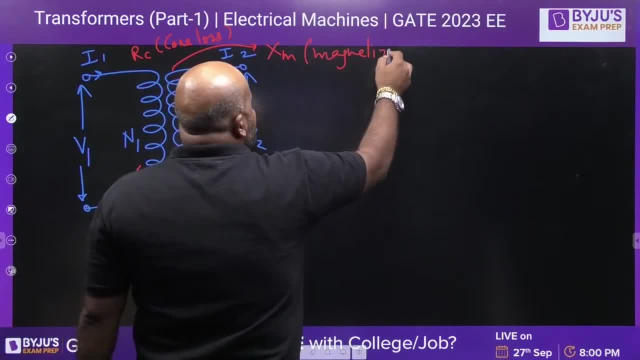 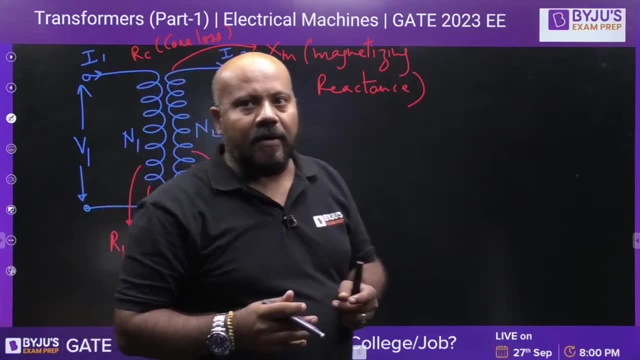 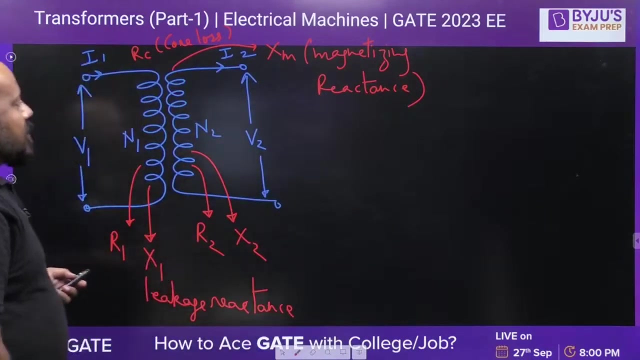 magnetizing reactance. magnetizing reactance, which represents the magnetizing current, to establish the flux in the core. I hope it is clear. So now you can draw the complete equivalent circuit of the transformer. It is going to be something like this: 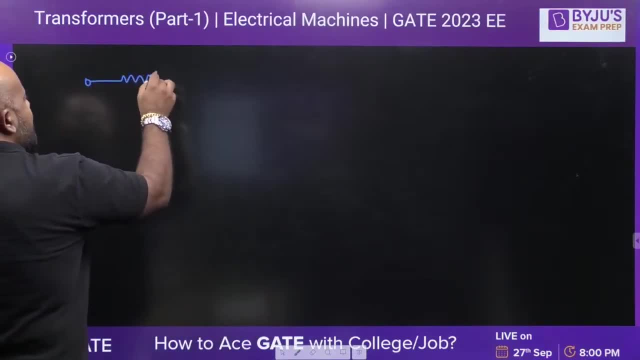 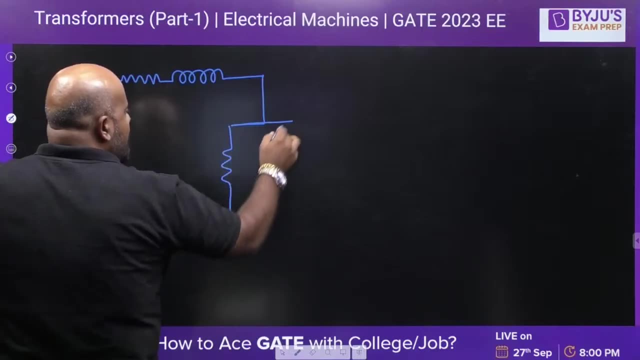 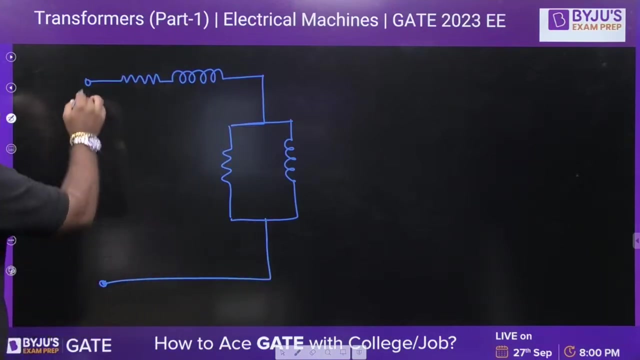 At the primary side, some resistance and then you have a shunt branch, something like this: This is the input voltage, supply voltage V1, this is the current I1, this is R1, this is Jx1,, this is Rc and this is Jx1. 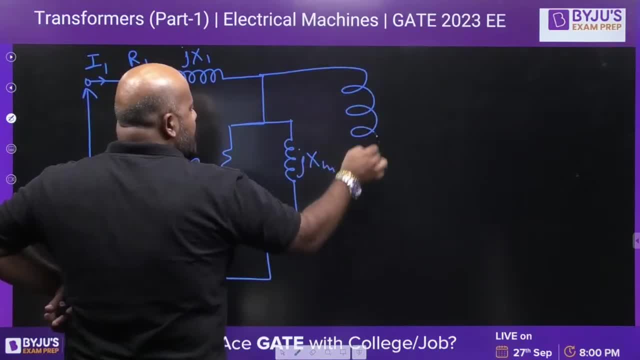 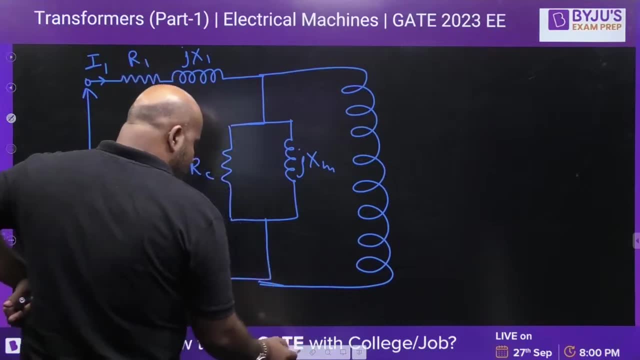 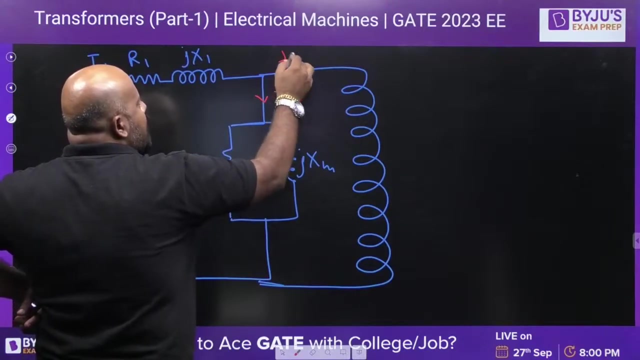 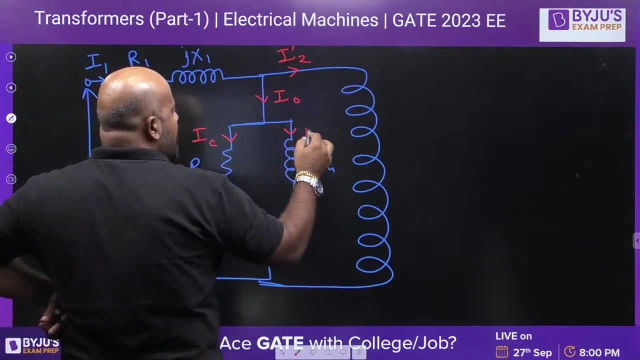 This is M. okay, And this is your primary winding. okay. Now see here: the current I1 here is going to be divided as I0 and this is going to be I2. dash, This I0 is further divided into Ic, that is the core loss component, and Im, or you can 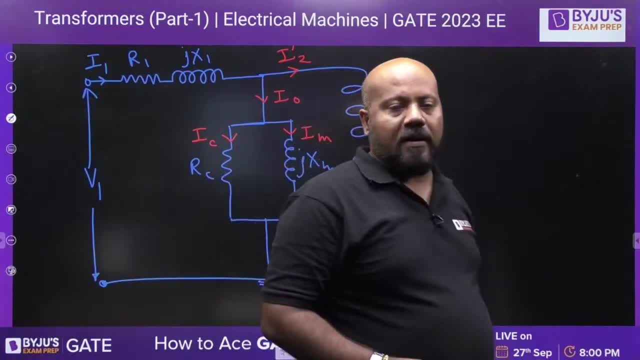 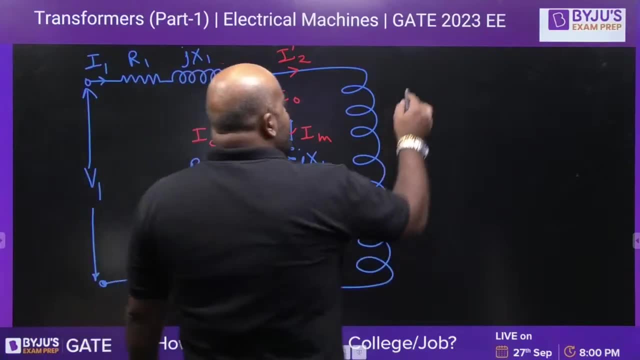 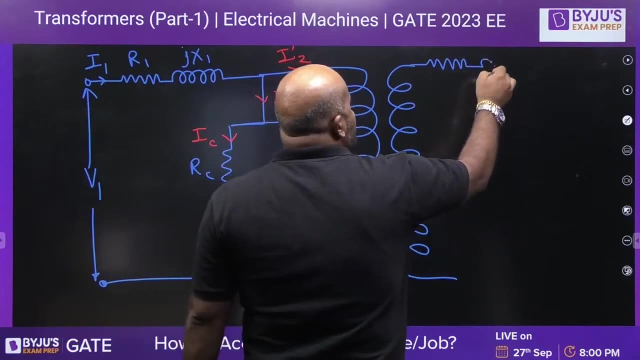 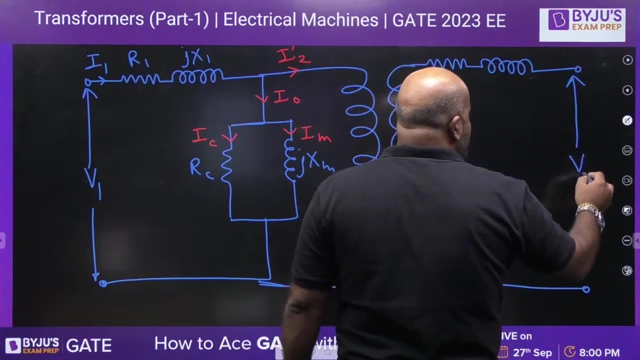 write Imu also to represent the magnetizing current. Okay, In the no load current. is it clear? Now for the secondary winding. again we have resistance leakage reactance. This is going to be V2,. okay, Current here is going to be I2.. 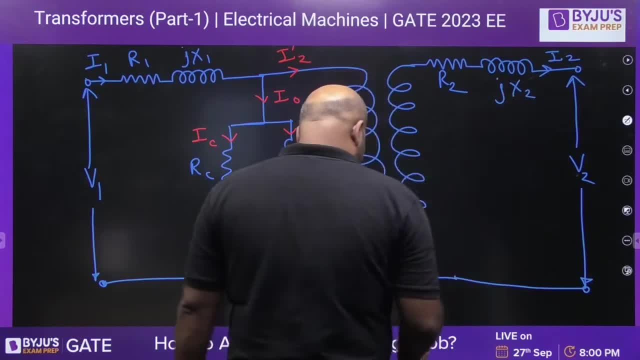 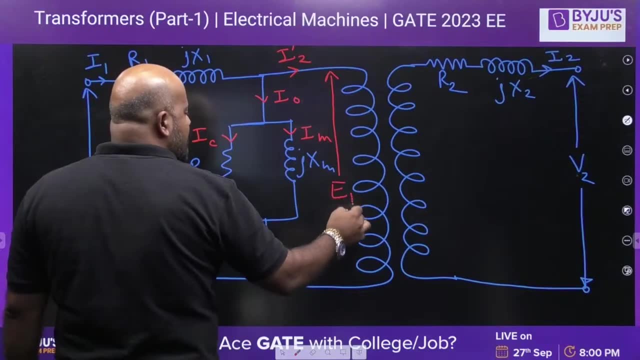 This is going to be R2.. This is going to be J. This is going to be X2.. If you see the EMF induced, the EMF induced at the primary winding is going to be: I am writing the RMS value, so this is E1.. 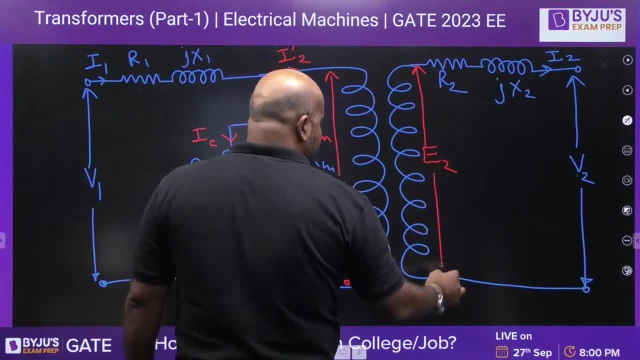 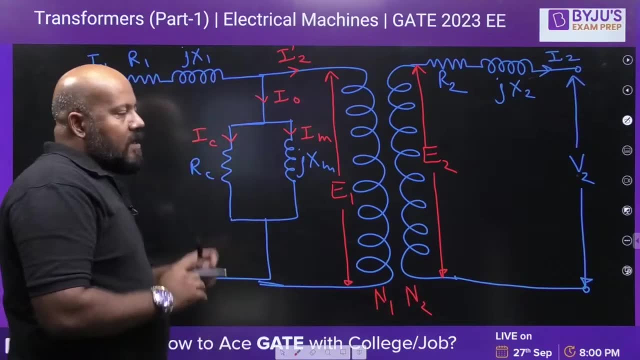 At the secondary side, the EMF induced is going to be E2, yes or no, And the number of turns are going to be N1 and N2.. But still, the equivalent circuit that you are having for the transformer is not the final equivalent circuit. 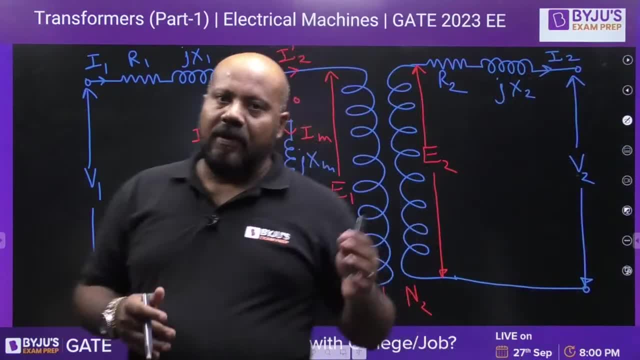 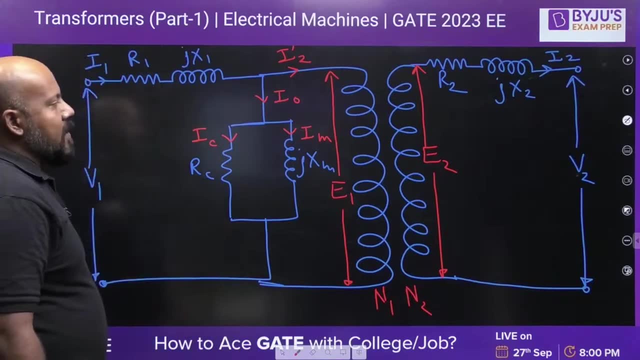 Why? Because Because the circuit is still primary and secondary, is isolated and it is very difficult to solve or analyze this particular circuit. So we are going to have some simplification. We are going to refer the secondary winding to the primary side, or you can refer primary. 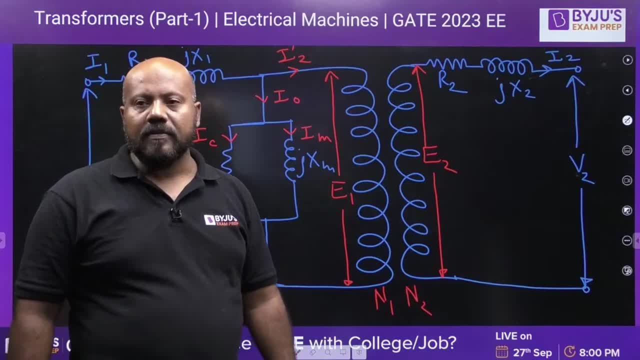 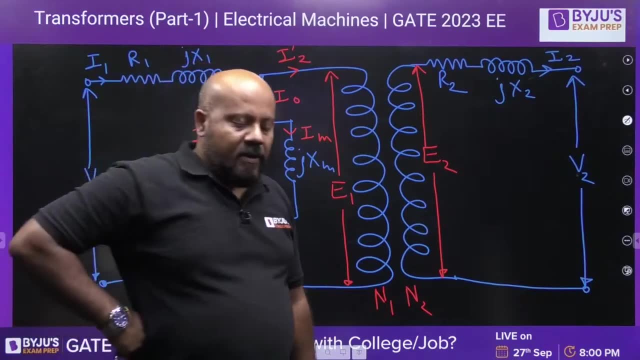 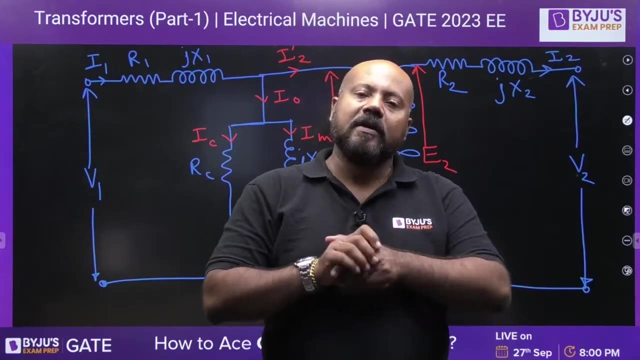 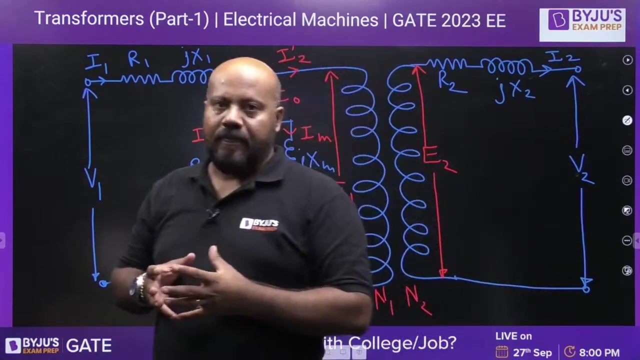 side to the secondary side also, Ramesh is saying: sir, please explain, See that V1 is equal to minus E1.. That is not actually a confusion. Okay, That is not actually a confusion. It depends how you are deriving the formula, how you are drawing the phasor diagram. 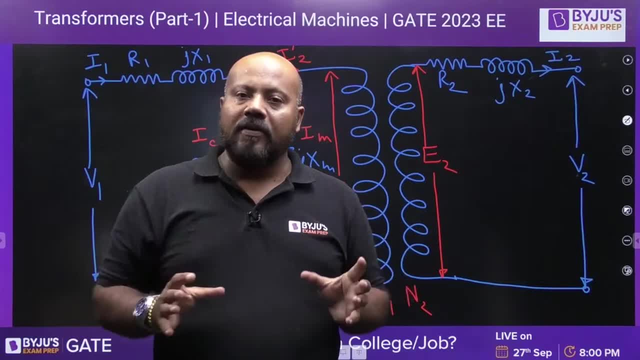 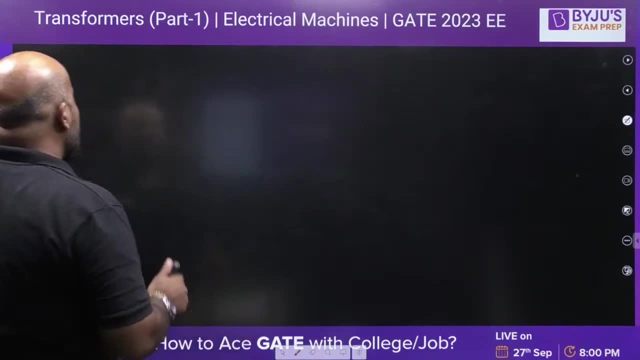 It depends on that. Okay, Some people what they are doing. suppose, if I am writing the expression like this, see If I am writing the induced EMF like this, minus N d phi by dt, Okay. Okay, Now, this will solve your doubt. 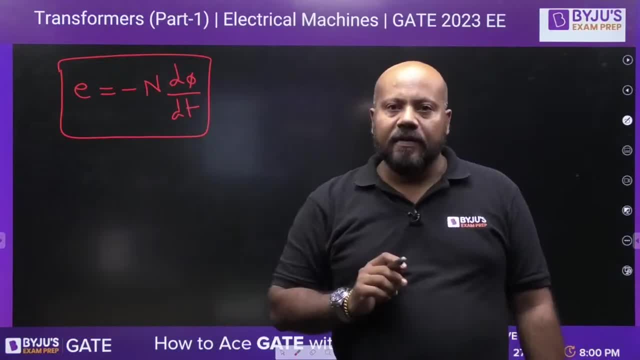 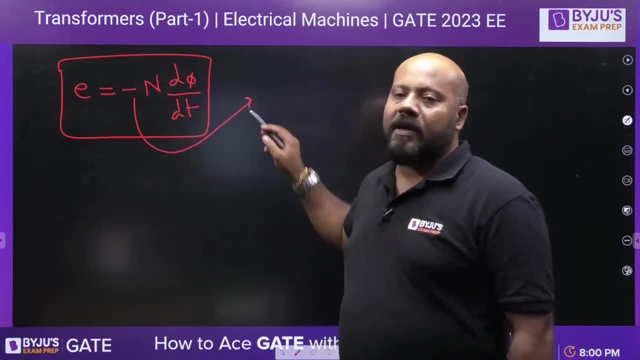 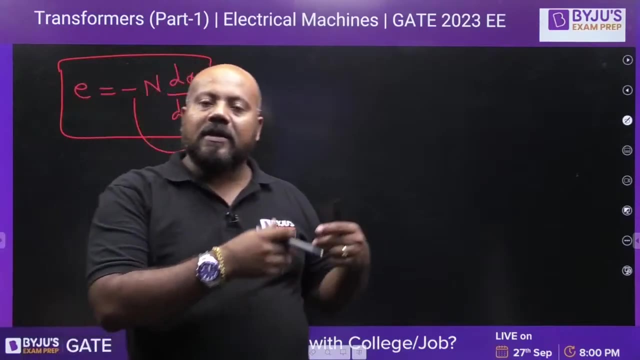 Okay, You are writing the induced EMF like this: This is the Faraday's law. But already, when I am discussing the transformer action, I have taken care about this negative sign. This negative sign already I have taken care of. I have already said it is a subtractive polarity dot. current enters the dot at one winding. 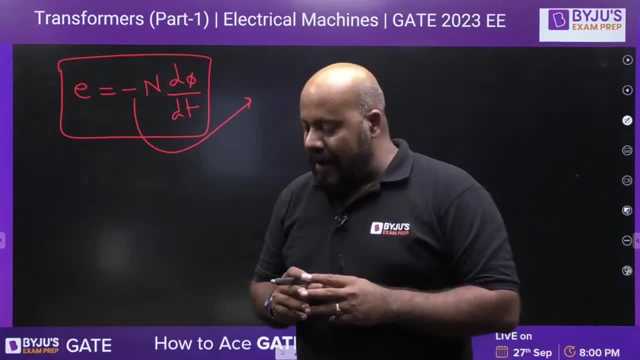 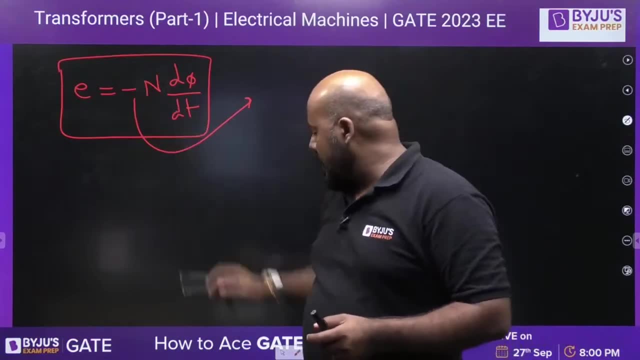 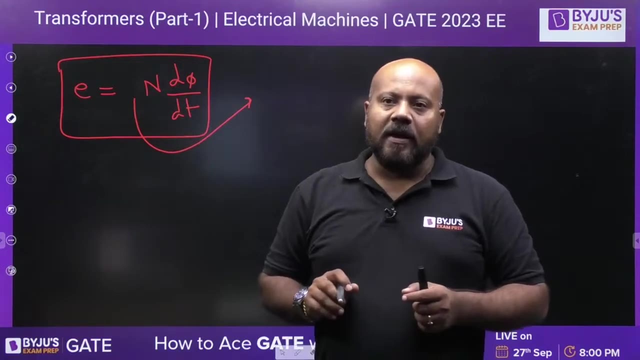 and leave the dot at the other winding. And I have already discussed the polarity of E1 and E2.. Accordingly, I have taken the polarity of E1 and E2.. So there is no meaning of using this negative sign. So if you do not use, if you do not use this negative sign, then you will be getting E1. 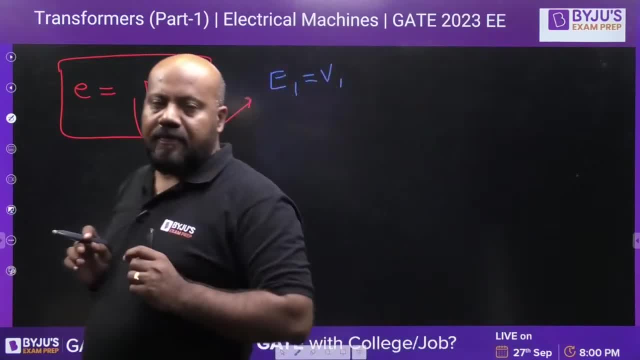 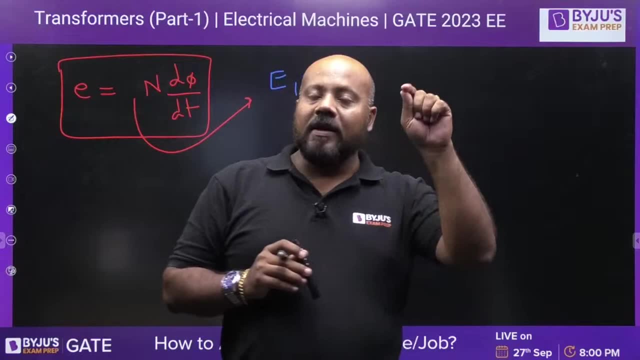 is equal to V1.. Are you getting that? And if you are using that negative sign, then you have to write. While doing that, you have to write, Okay. Okay, While drawing the phasor diagram or while deriving the expression, you have to write. 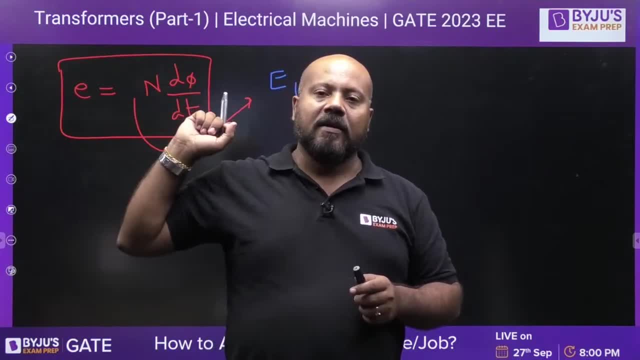 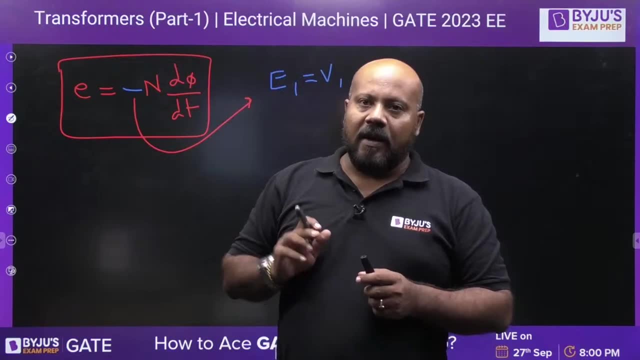 what is the significance of this negative sign, why you are taking it So in some of the standard books. what they are doing, they are simply blindly writing like this: And then they are drawing the phasor diagram. That is also okay. 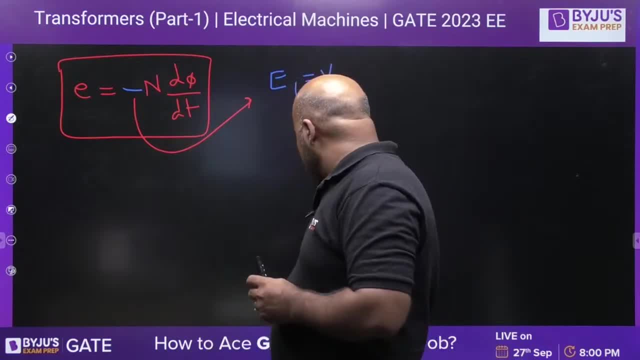 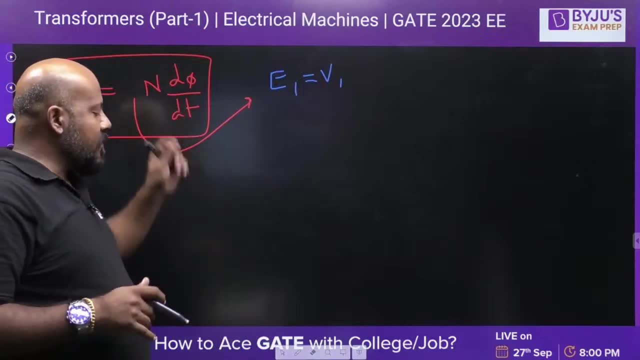 That is also okay, But I do not prefer this. Why? Because already we have taken care of the Lenz law, taken care of the polarity and the primary and secondary winding. So why do you get confused? But both the methods are correct anyways. 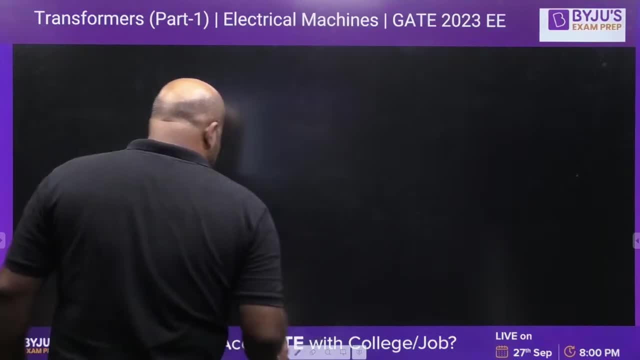 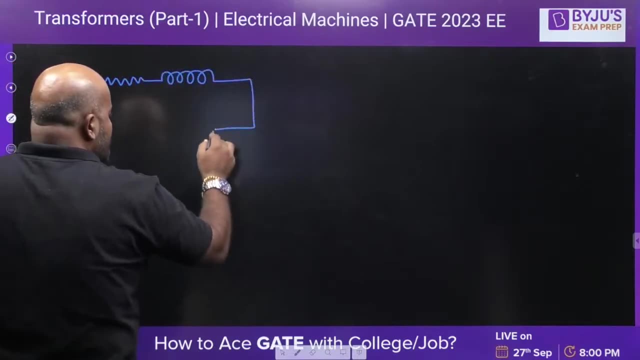 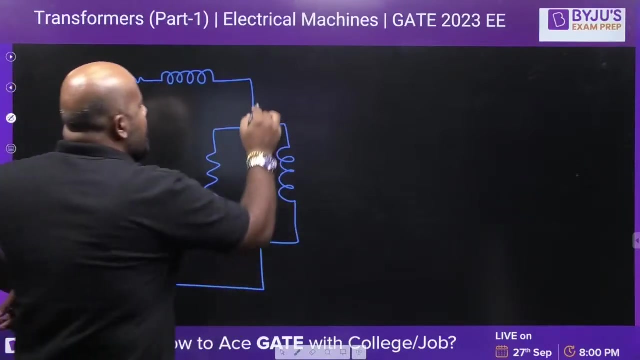 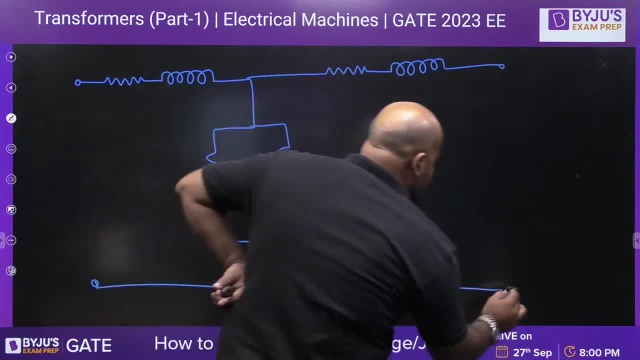 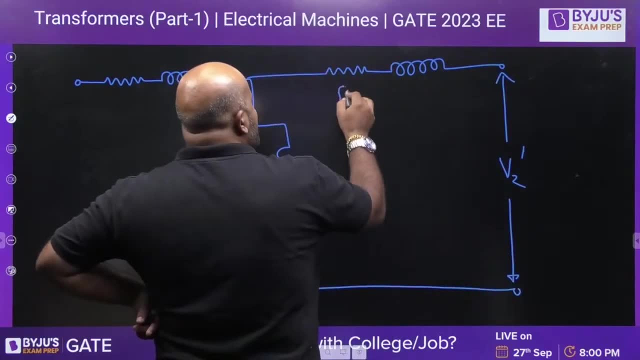 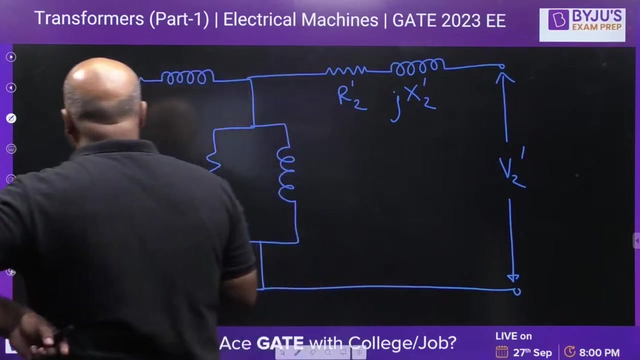 Okay, This is going to be V2 dash because it is referred to the primary side. This is going to be R2 dash, referred to the primary side. This is jx2 dash because it is referred to the primary side. Primary side: unaffected. 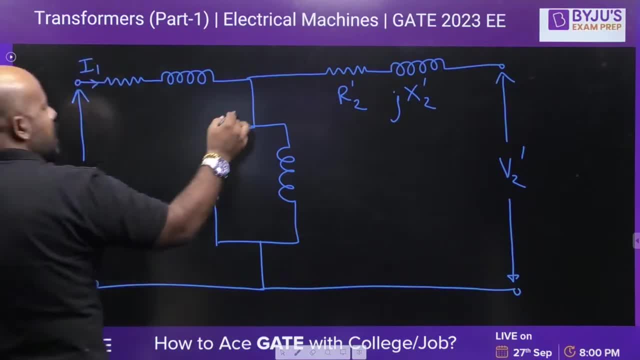 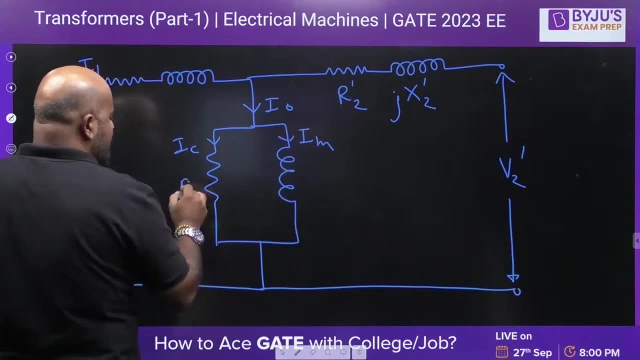 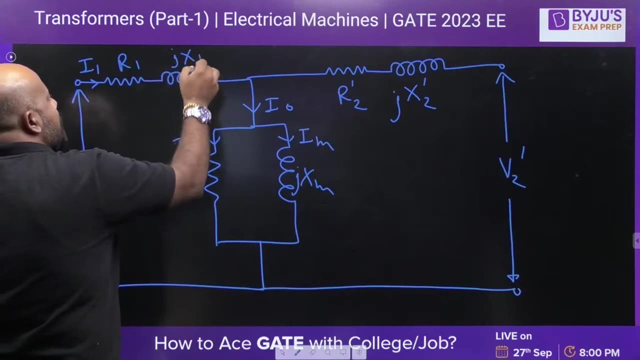 It is V1,. it is current I1.. This is I0.. This is IC, This is IM m, this is R c, this is X m, this is R 1, this is J X 1 and this is I 2 dash because. 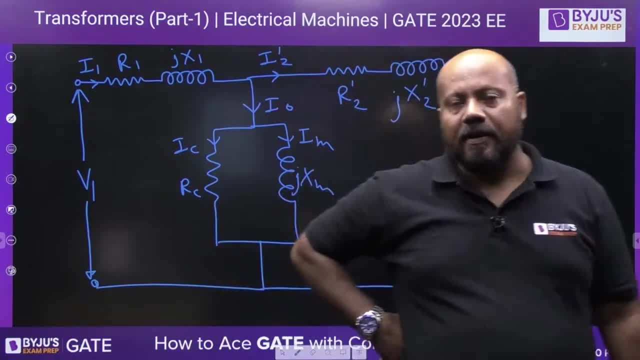 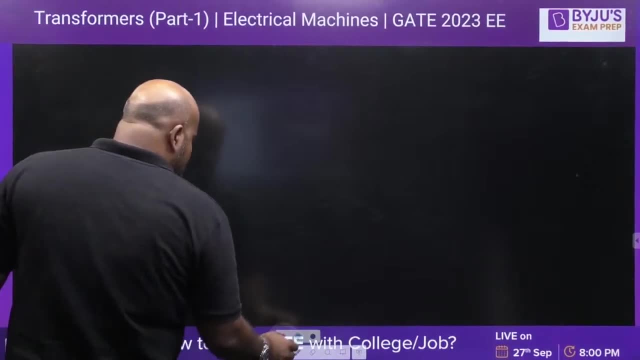 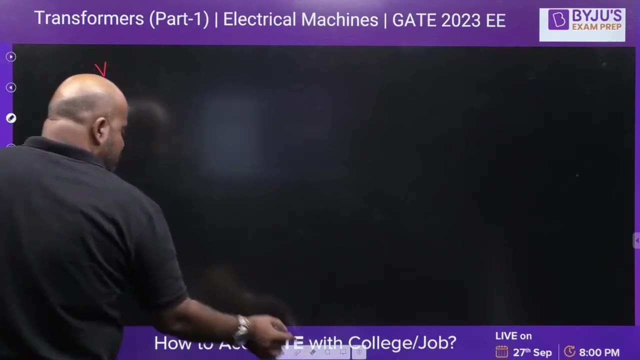 refer to the primary side. refer to the primary side. What is this? V 2 dash, I 2 dash. please try to understand. We are defining. we are defining. let me write like this: E 2 upon E 1 as N 2 upon N 1, this: 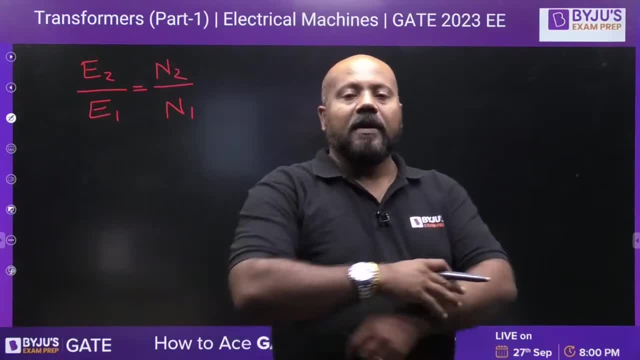 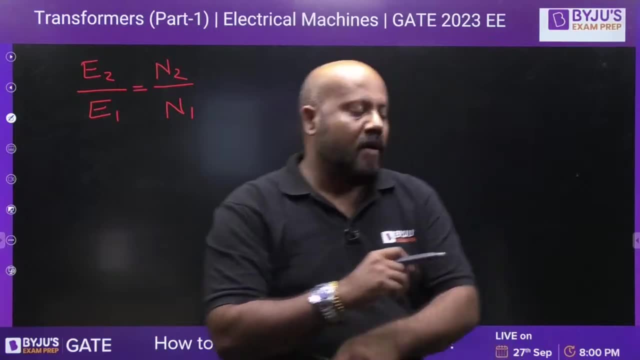 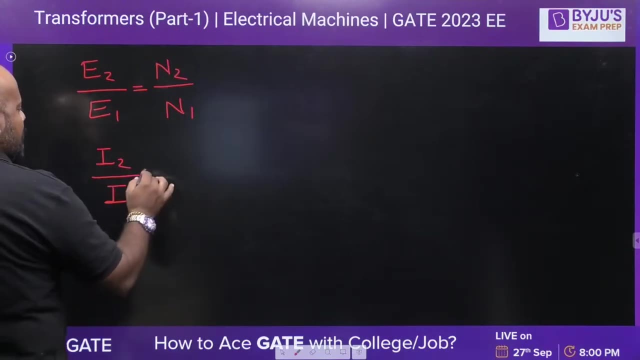 is the best thing you can write instead of writing V 1 and V 2, because if you are having a practical case, in the practical case you cannot directly relate voltages with the turns ratio directly. ok, Anyways, And we are having I 2 upon I 1. listen very carefully- is equal to N 1 upon N 2, this is 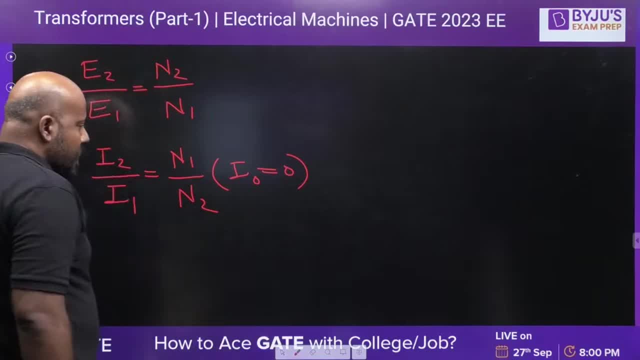 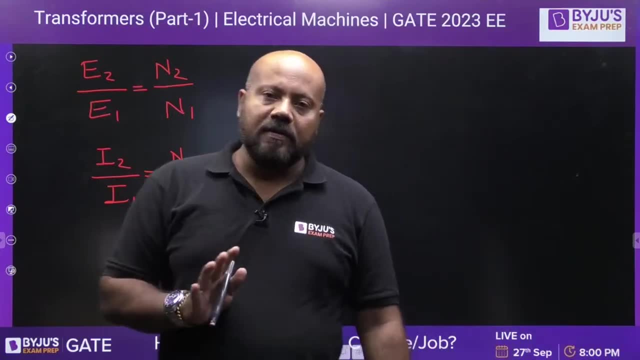 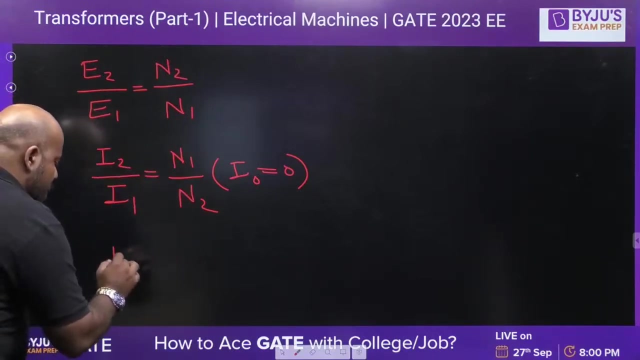 only possible when you are saying I naught is equal to 0,. this is only possible. this relation you can only use when I naught is 0, are you getting this or not? because we have seen the M- M- F balance equation. So how we are writing I 2 dash, see here. 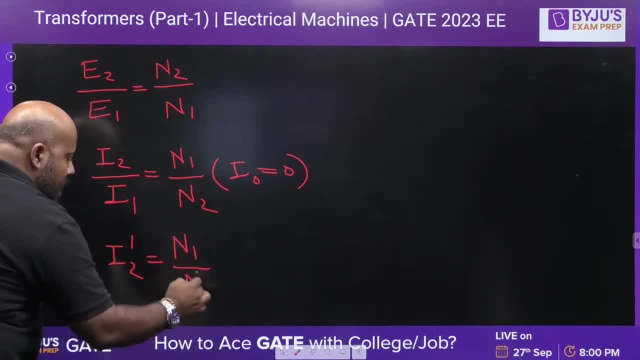 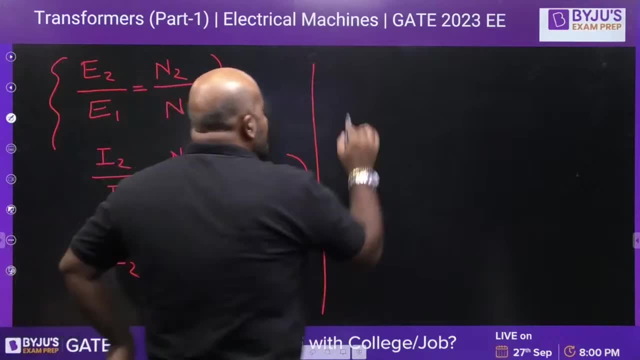 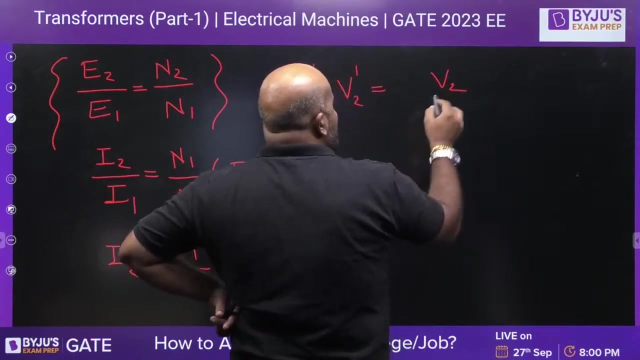 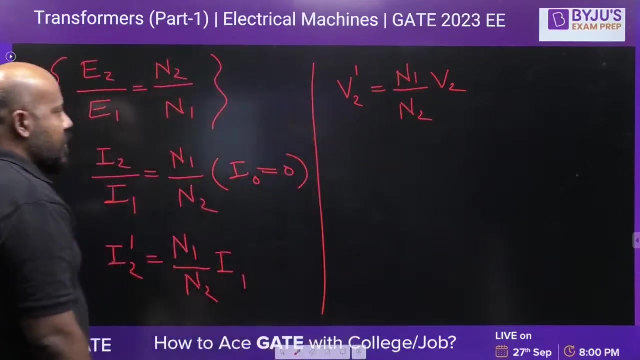 I 2 dash. I 2 dash. we are writing as N 1 upon N 2, and this is I 1.. By using this voltage relation, we are writing V 2 dash. as this is V 2, ok, it is divided by N 2 and multiplied by N 1. is it clear, ok? 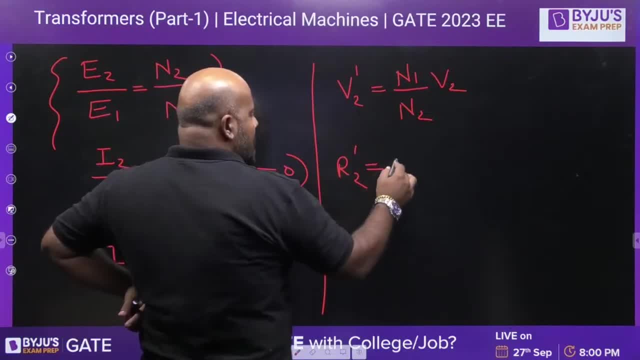 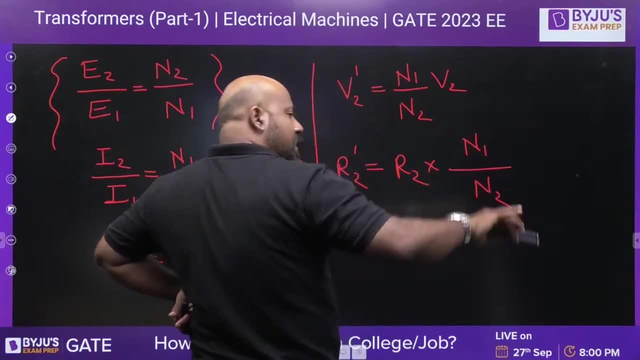 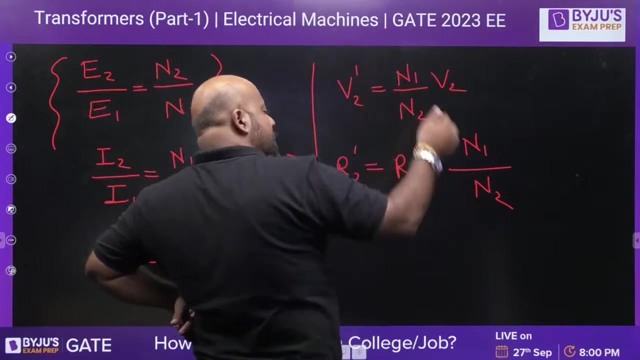 How we are writing R 2 dash. See here R 2 from where you are going to where from. from where you are going and to where you are going you are coming from N 2.. So write N 2 in the denominator. you are going to N 1, primary side. to write N 1 in. 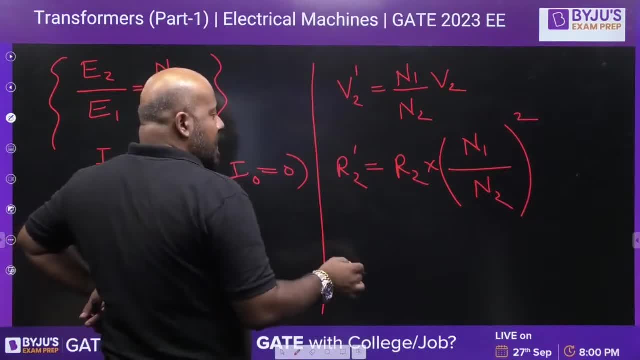 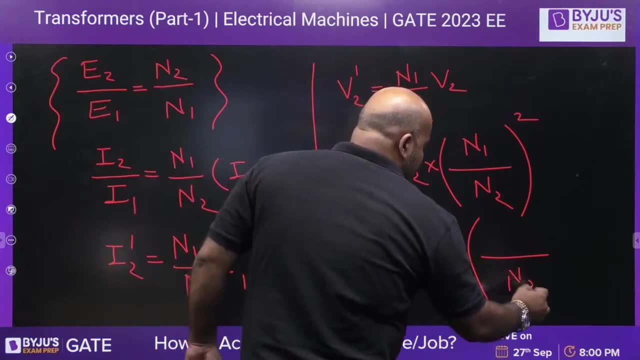 the numerator and make the square For impedance R and X. you have to do like this: X 2 dash. it is X 2, this is again N 2.. So I have to write this as X 2.. So I am writing X 2 dash. 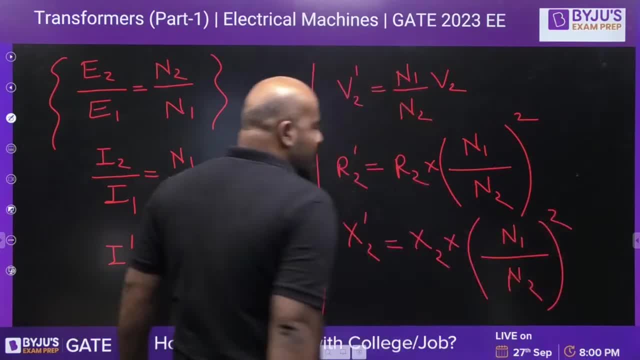 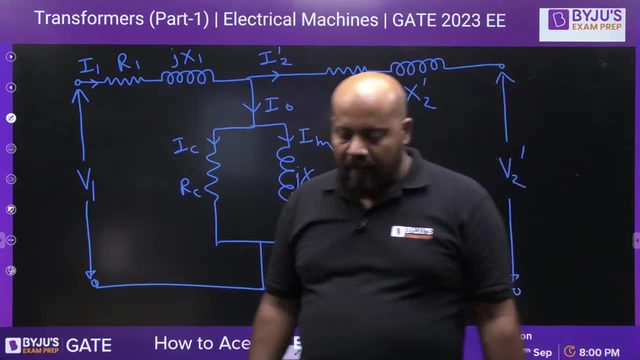 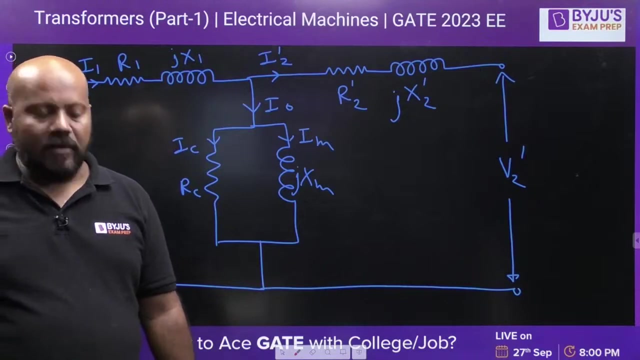 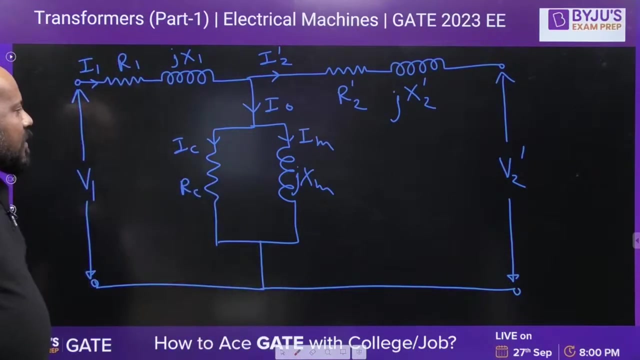 I am writing X 2 dash. This is n 1. do the square. Is it clear? everybody, Everybody, just tell me, are you able to follow this? Say yes or no. At least say yes or no. Clear Now. this equivalent circuit is going. 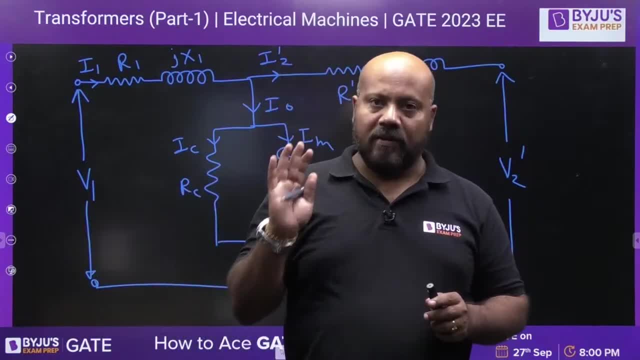 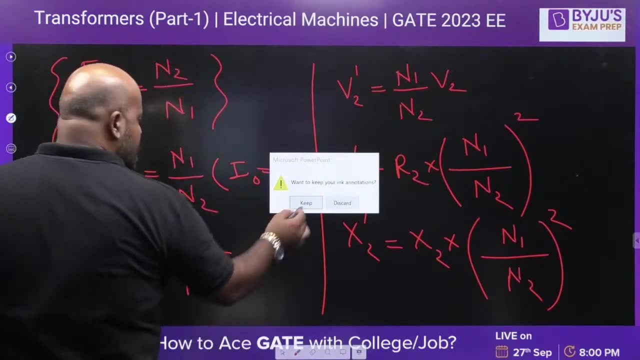 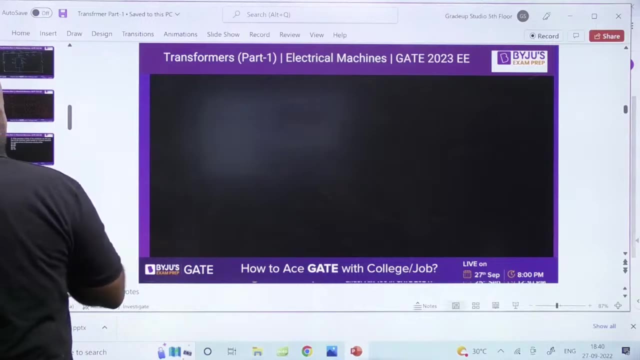 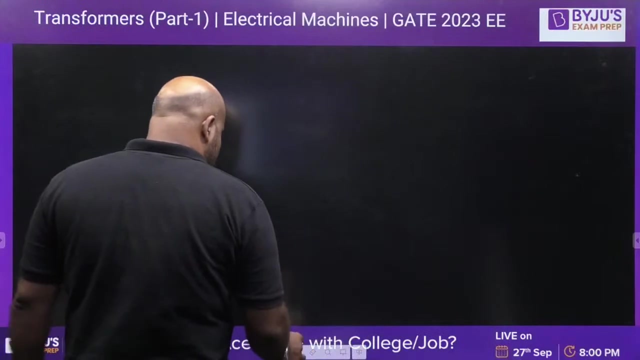 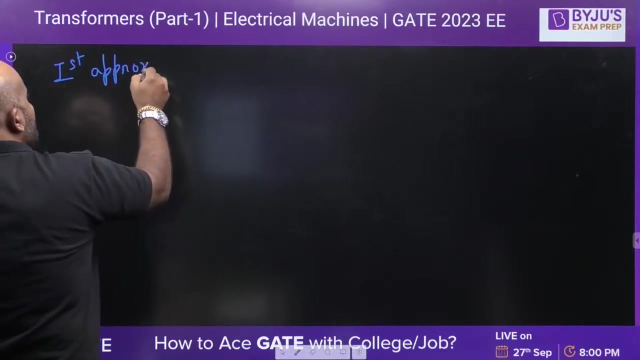 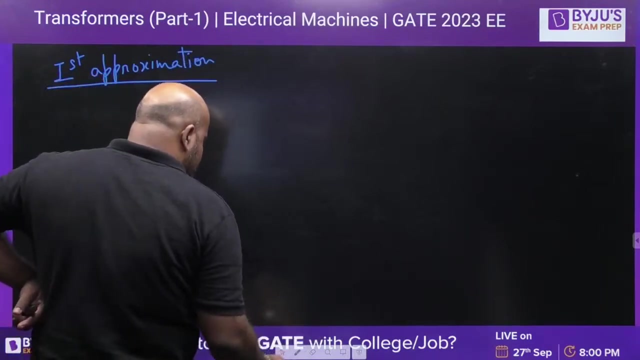 to be the actual equivalent circuit which you have to use. But there are two simplifications. One simplification again. let me add two more pages. Anyways, The first approximation circuit. What is the first approximation circuit? Please see here. First approximation circuit is something like this: 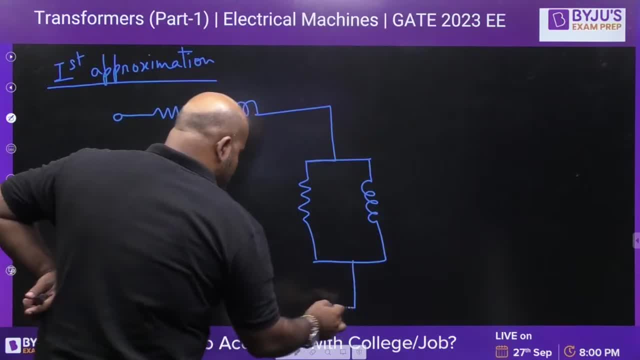 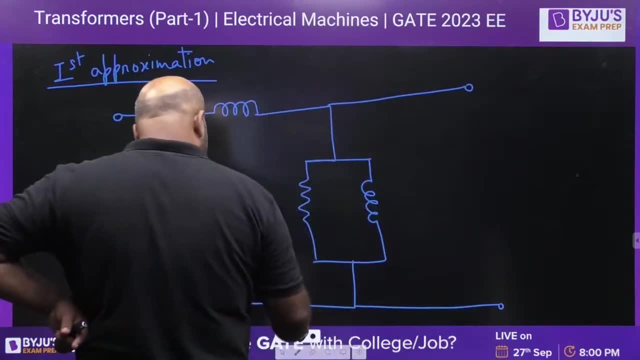 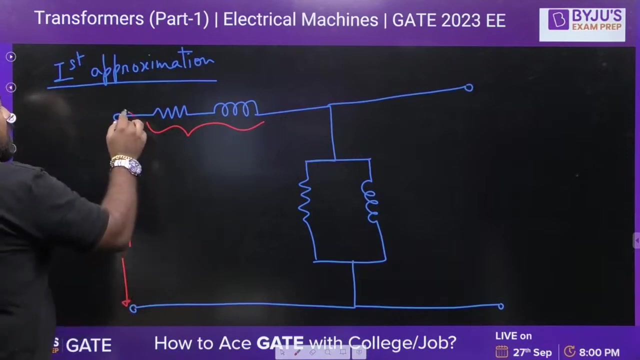 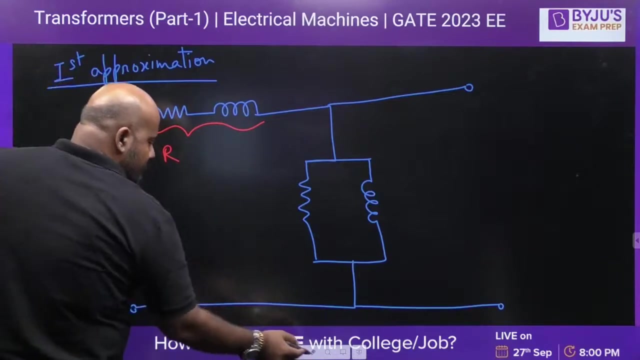 This is what we are writing as this is v 1.. This is current i 1.. This is what we are writing as see here. We are writing here as this: It is z 0, 1. 1. 1.. 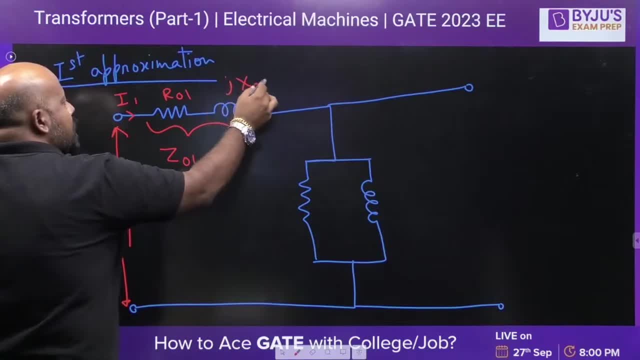 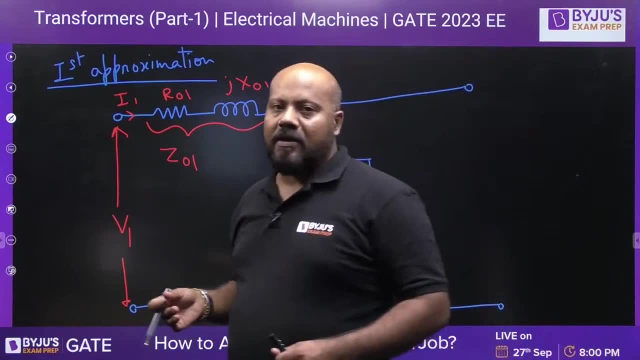 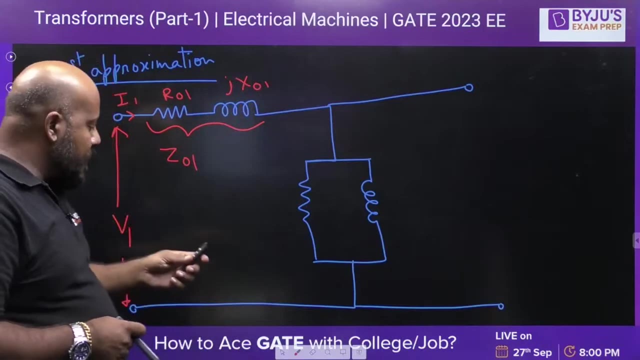 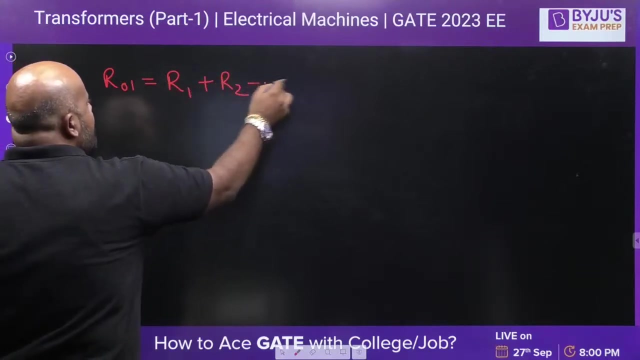 is R 0- 1. this is X 0- 1.. So it basically gives you the equivalent or effective resistance referred to the primary side. equivalent or effective reactance referred to the primary side. How we are writing this: R 0- 1. we are writing as R 1 plus R 2, N, 2, N, 2 upon. this is: 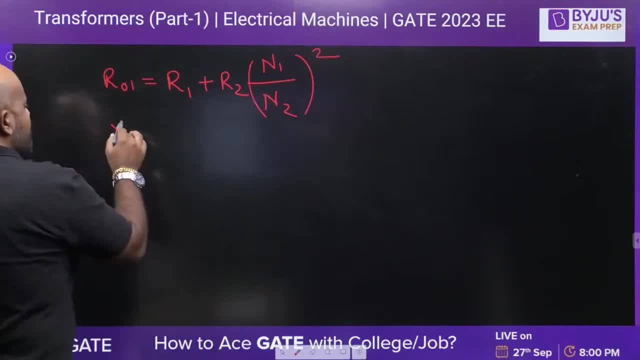 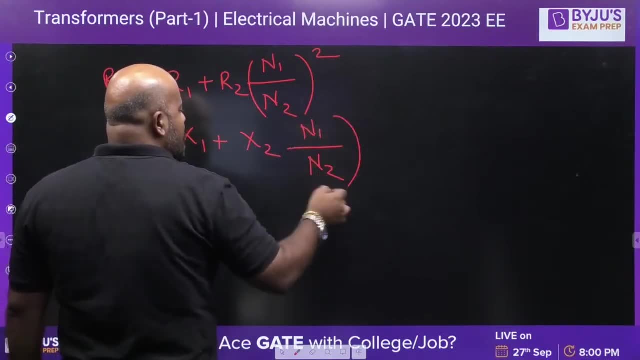 N 2. this is N 1 to the square. X 0: 1. this is X 1 plus X 2. N 2 here, N 1 here to the square. Is it clear? This is going to give you the equivalent or effective resistance referred to, the primary. 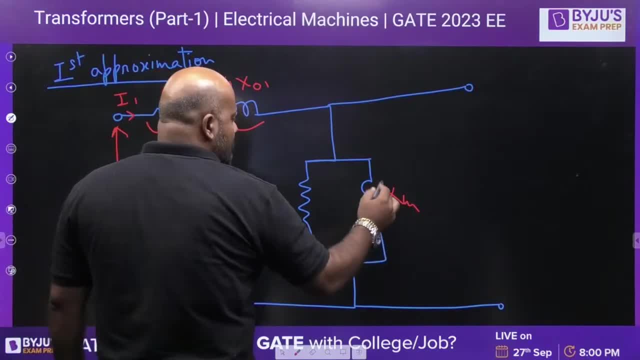 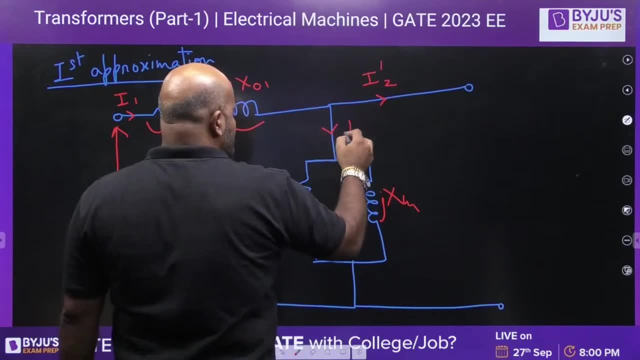 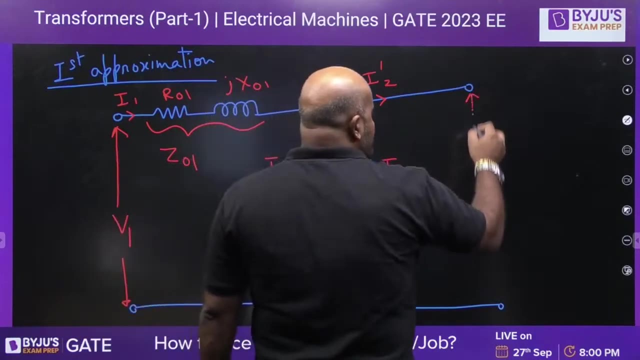 side. So this is going to be R C, this is going to be X M. ok, This is going to be your I 2 dash. this is going to be I 0, this is I C and this is I M. this is V 2 dash, like this: 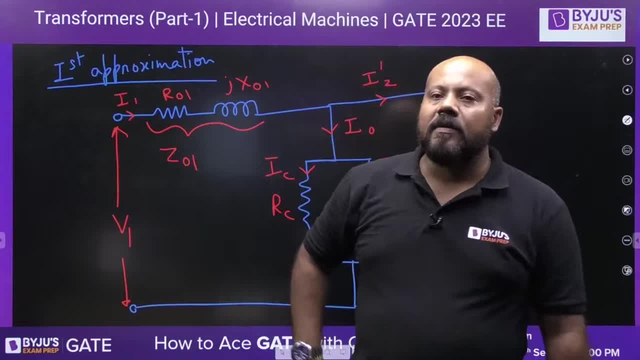 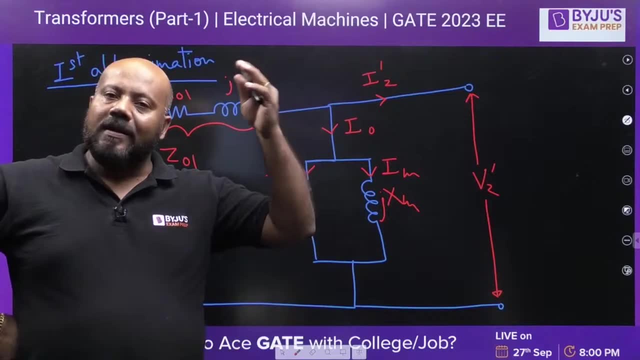 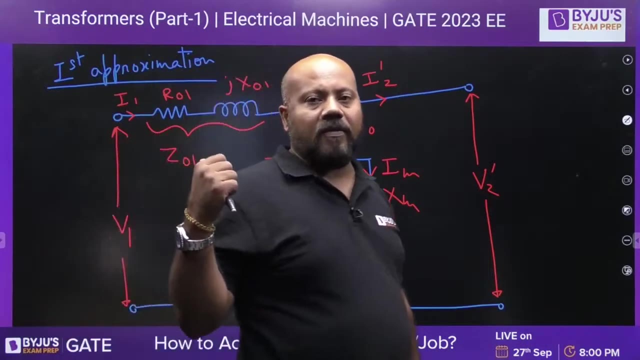 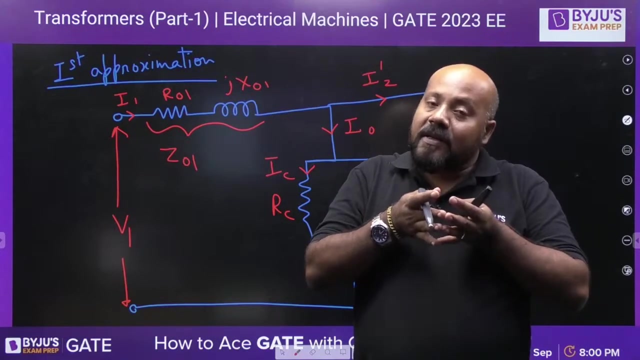 This first approximation circuit, shunt branch is already modeled in the primary side. we have referred secondary side to the primary side in this equivalent circuit of the transformer. this is the first approximation. what we are doing we are actually trying to separate the constant losses and the variable. 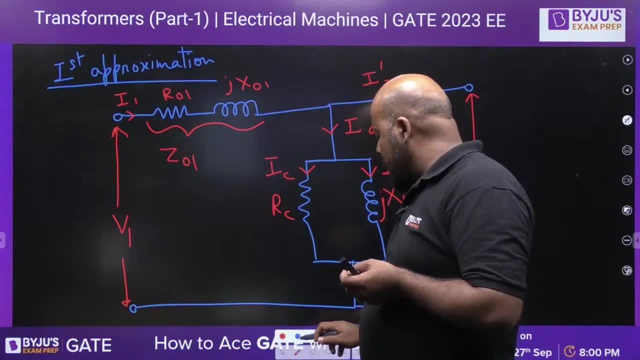 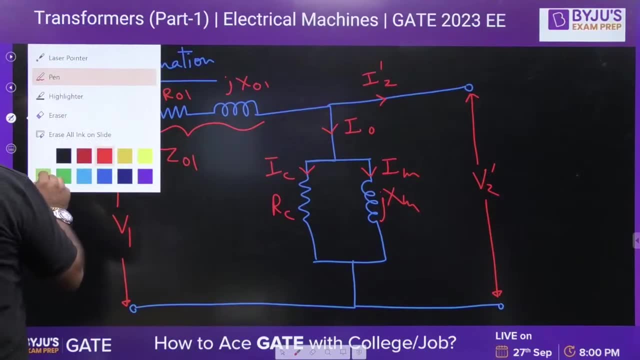 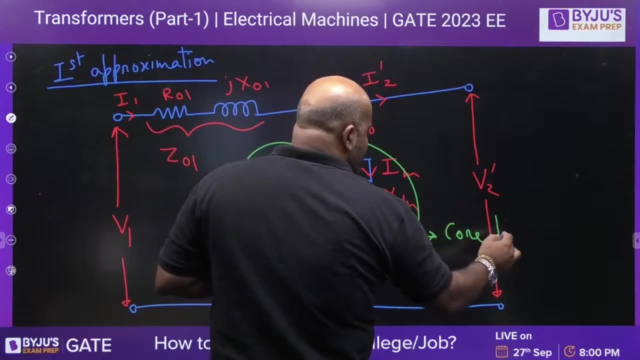 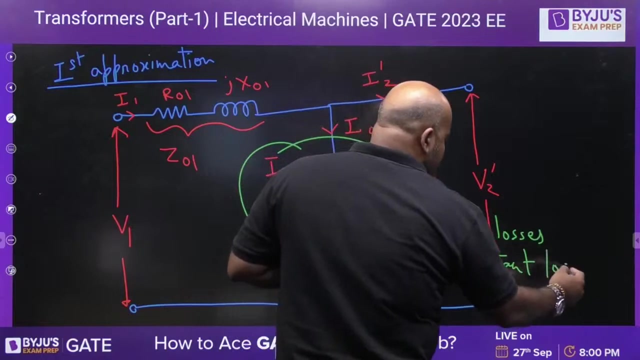 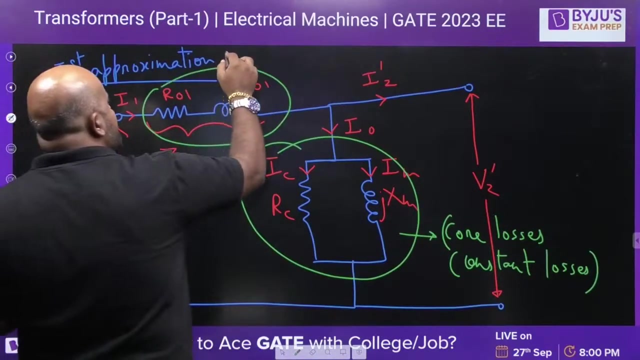 losses, the shunt branch. the shunt branch refers. the shunt branch refers the constant losses or the core losses. it represents core losses or the constant losses. So whenever you have to make the efficiency calculation and this series branch is going to represent the copper losses, 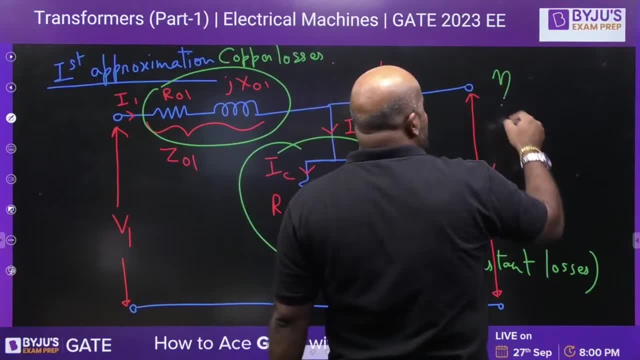 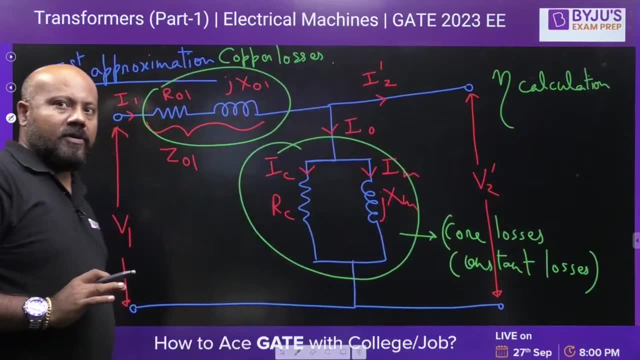 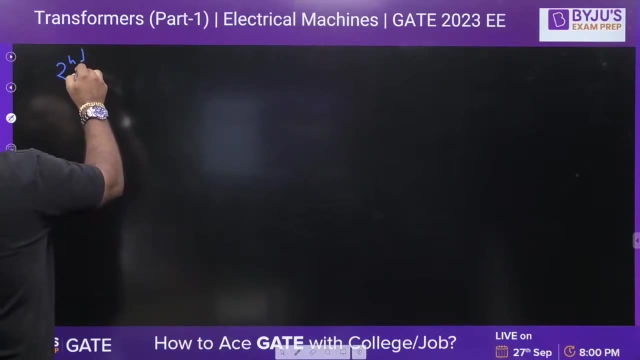 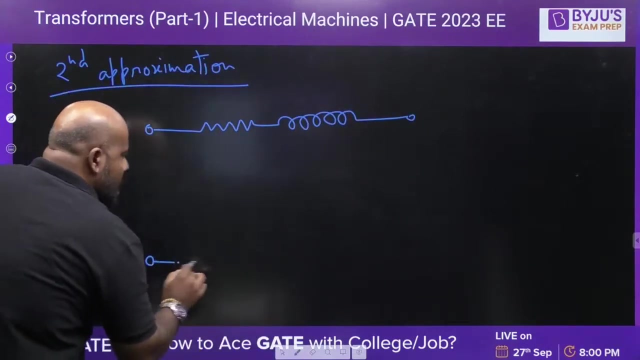 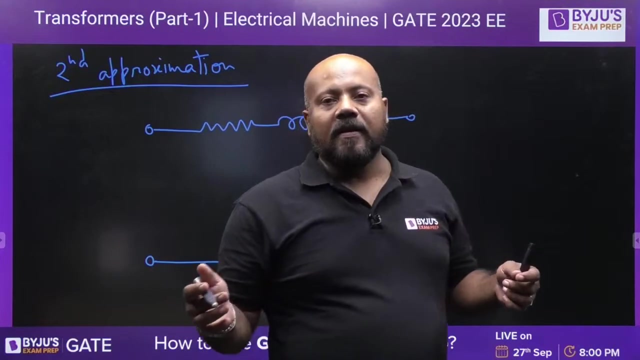 So basically, for efficiency calculation, For efficiency calculation, this approximate circuit is going to be the best choice. if you have to solve the questions, Then we have second approximation. Second approximation is going to be something like this: So now this transformer has undergone a weight transformation surgery. ok, 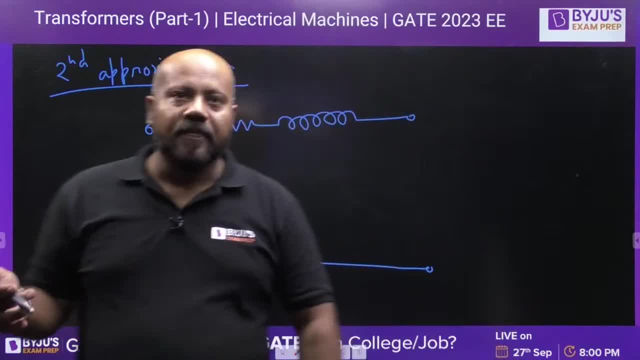 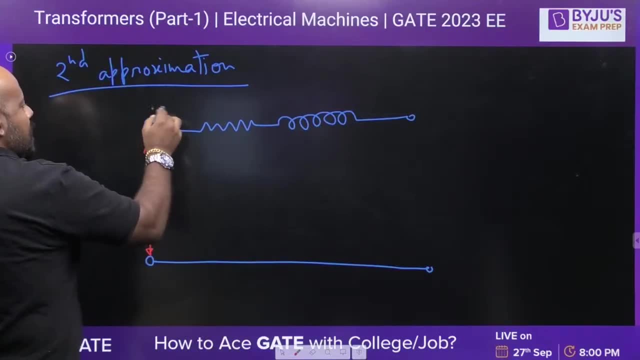 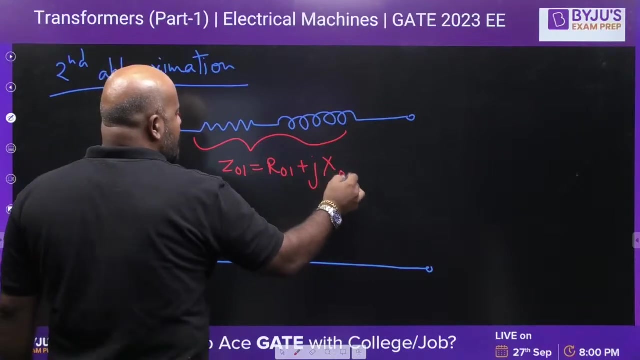 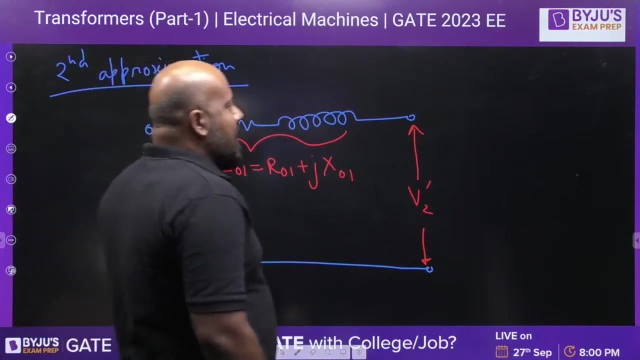 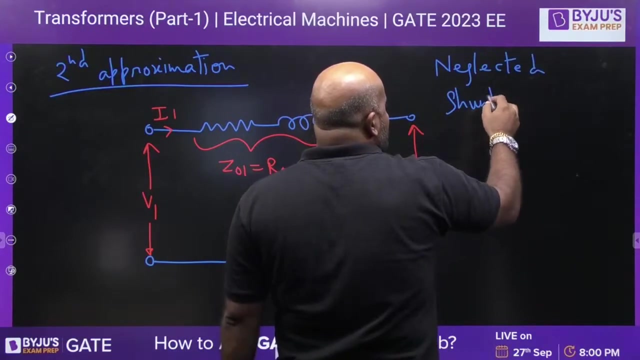 So you can enjoy this. you understand. This is actually V 1, this is I 1. this is again Z 0, 1, that is R 0, 1 plus J X 0, 1.. This is V 2.. V 2: dash, we have neglected the shunt branch. neglected shunt branch and this equivalent. 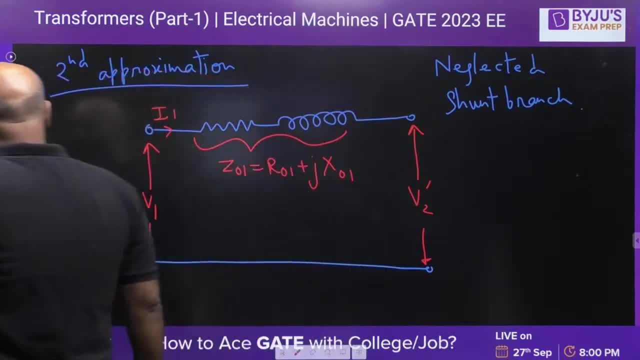 circuit you can follow. you can use in the gate examination when you have to solve the questions related to voltage regulation. when you have to solve the questions related to voltage regulation, Is it clear for everybody? just tell me yes or no in the comment section. Thank you. 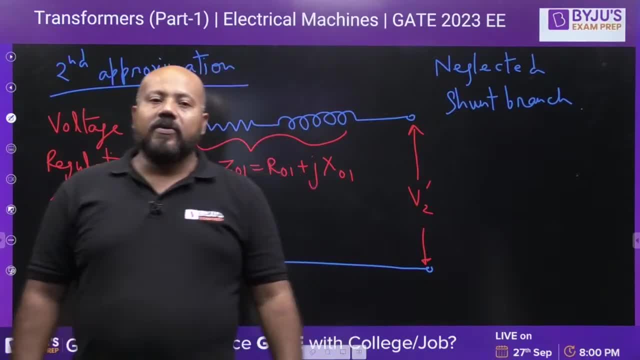 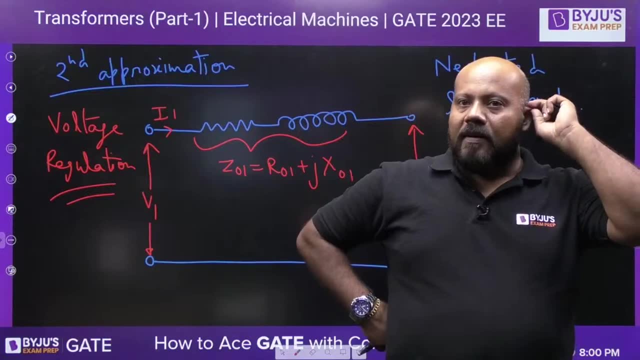 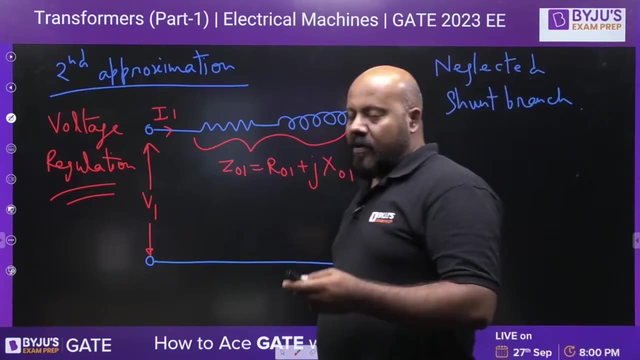 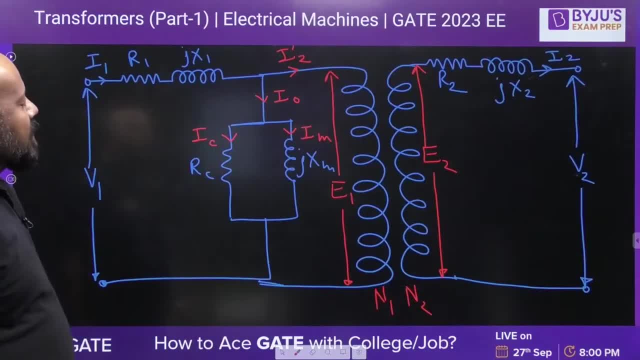 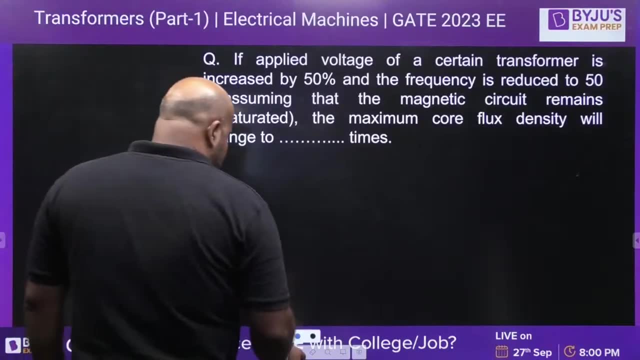 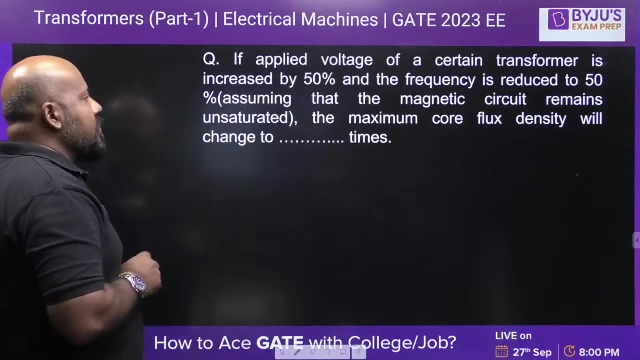 Let us now discuss the problem. See the first problem. He is saying: if the applied voltage of a certain neck to neck circuit is to produce resistance of a certain transformer is increased by 50 percent and the frequency is reduced to 50 percent, assuming that the magnetic circuit remains unsaturated, 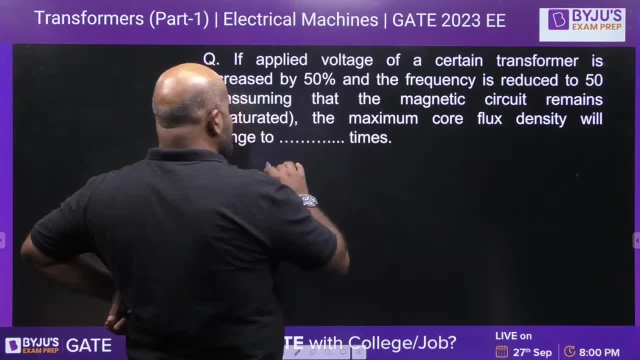 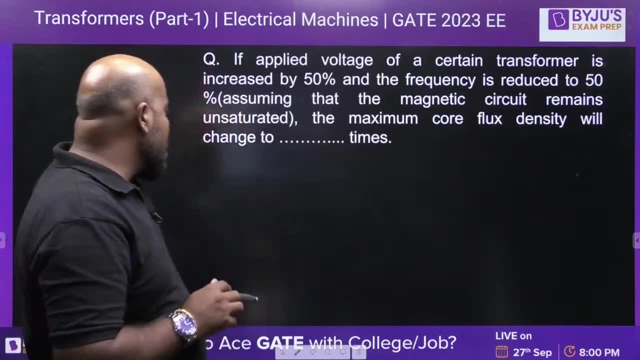 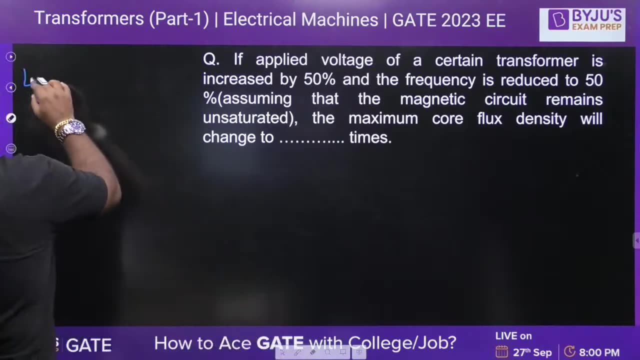 the maximum core flux density will be will be changing to how much times you first understand how magnetic flux density is related to voltage and frequency. what is the emf equation if you write for the primary side, if you write for the- let me add some pages here- okay, why to compromise? 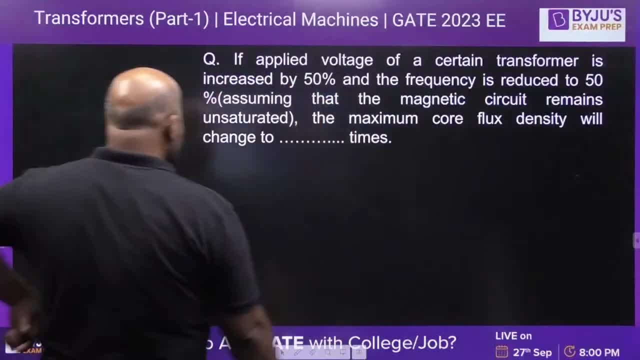 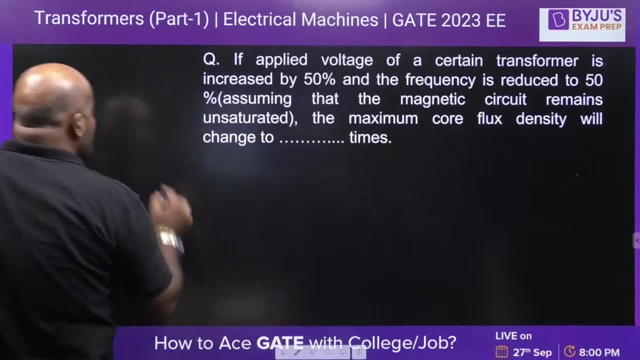 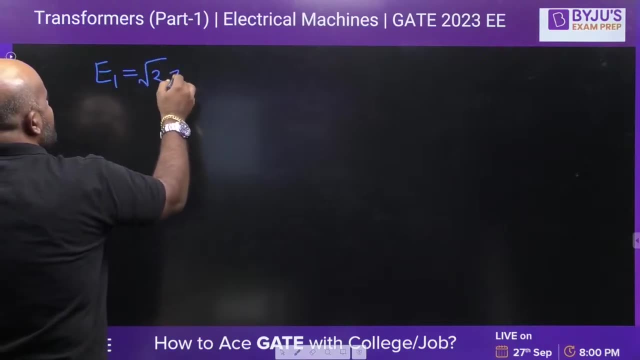 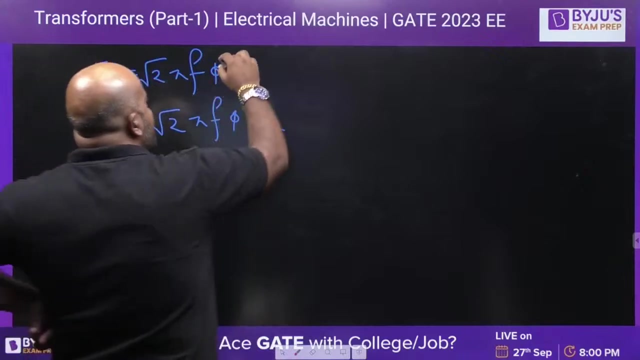 that is sufficient. so if you write the primary side voltage, primary side voltage e1 is going to be root 2 pi f phi. this is n1. and what is e2? this is root 2 pi f phi and this is n2. what is this phi value? can you tell me what is this phi value? 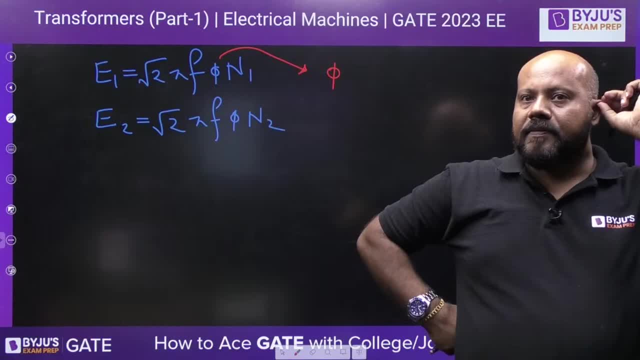 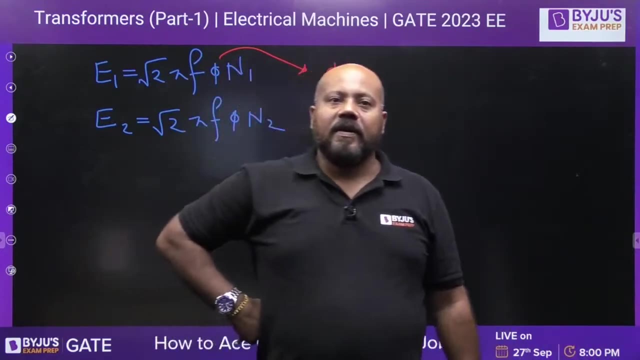 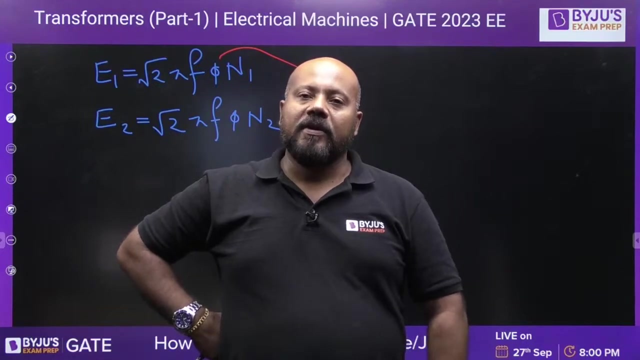 yes, anyone can you tell me? yes, karthik, you are very smart. we are not discussing the condition for maximum efficiency and you are writing this okay. okay, when you will get a good rank in the gate examination, then you do not need to show it to anyone, people will come to you. okay, nobody is asking you. 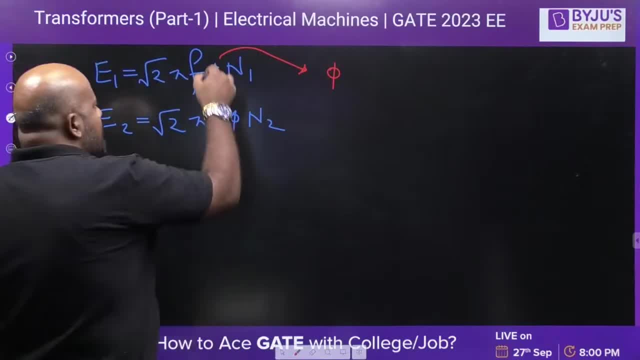 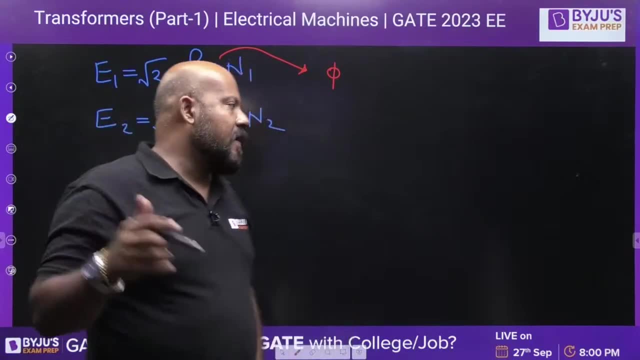 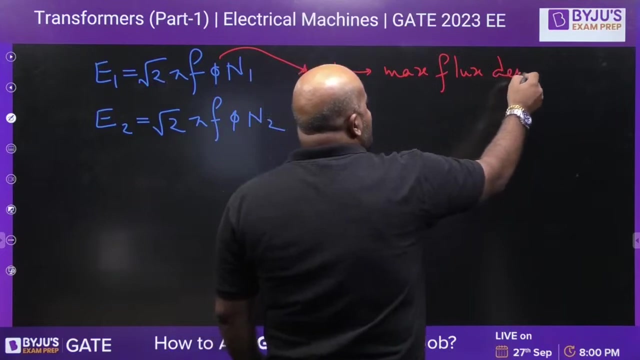 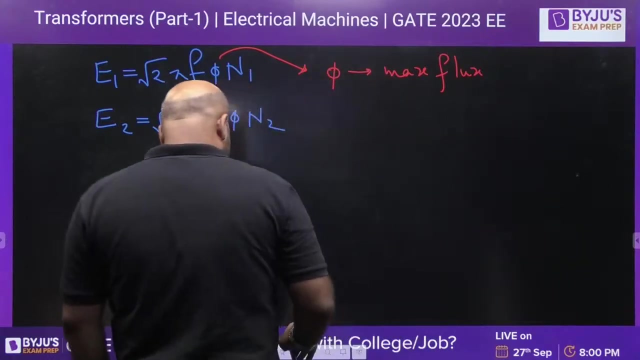 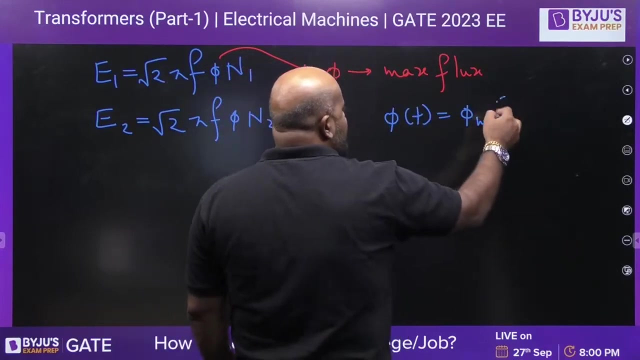 listen here. this phi is what you see, the derivation of this induced emf e1 and e2. you will understand this phi is the maximum flux density, actually maximum flux. you remember we were defining it as phi m sine, or cos omega t, whatever you want. so this phi m we are using here, 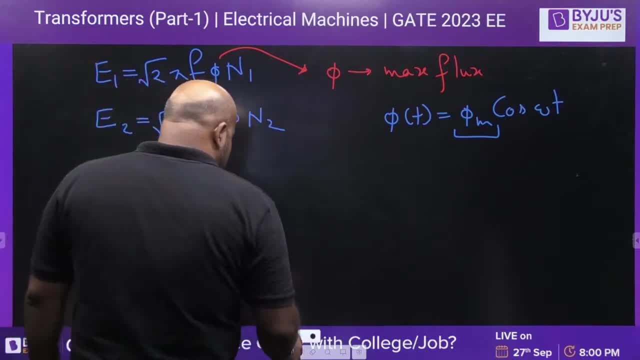 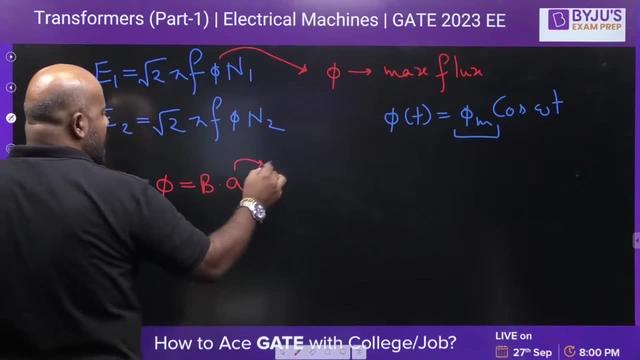 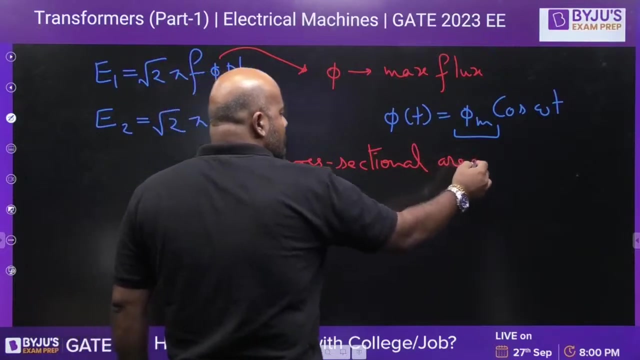 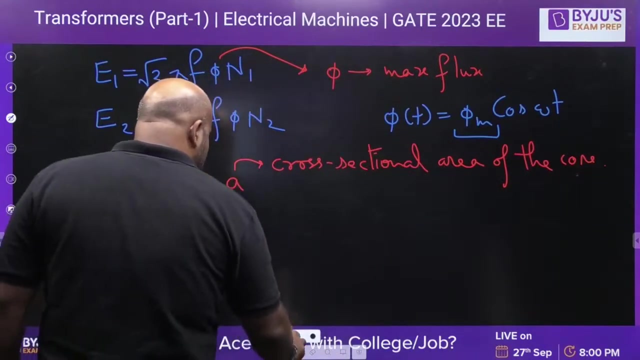 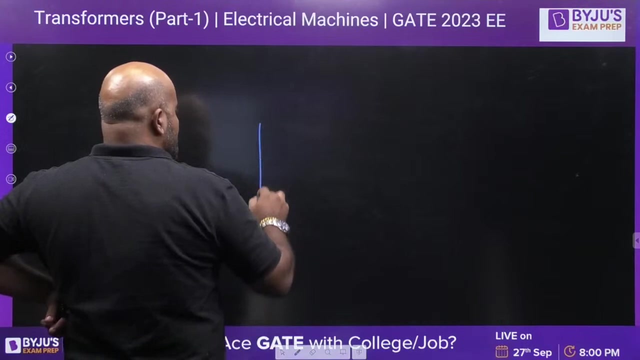 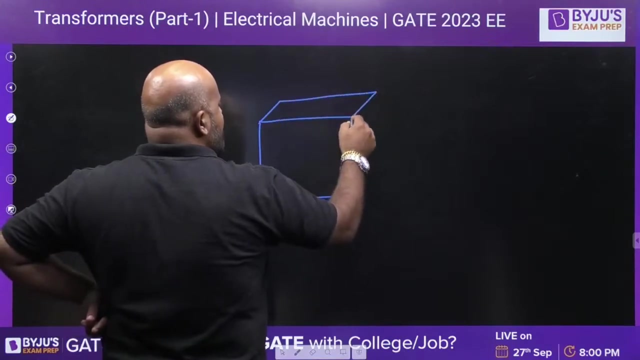 yes or no. so how you are writing this phi m. please see here this phi you can write as magnetic flux density multiplied by a, what is a cross sectional area of the core. i hope you understand what is the cross sectional area of the core. okay, so do not become mad after watching this diagram. okay, i have no guarantee. 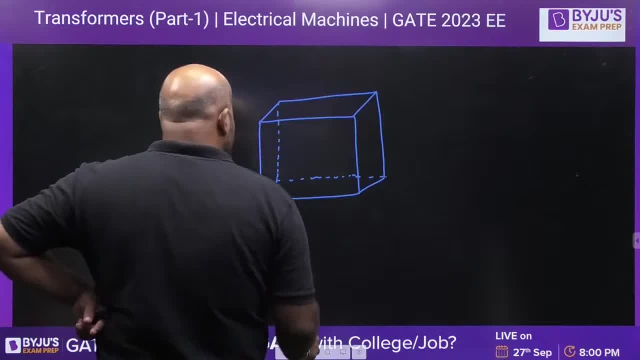 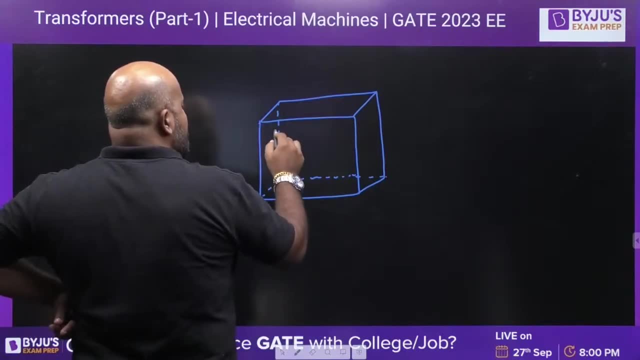 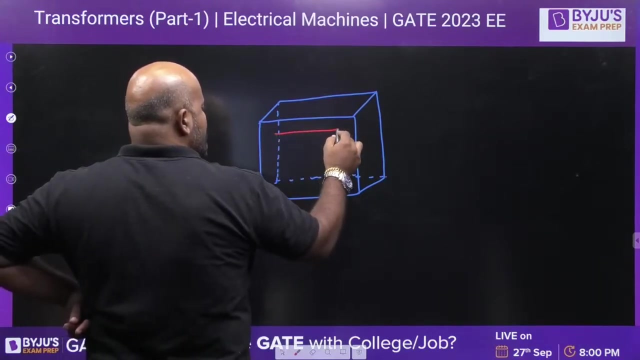 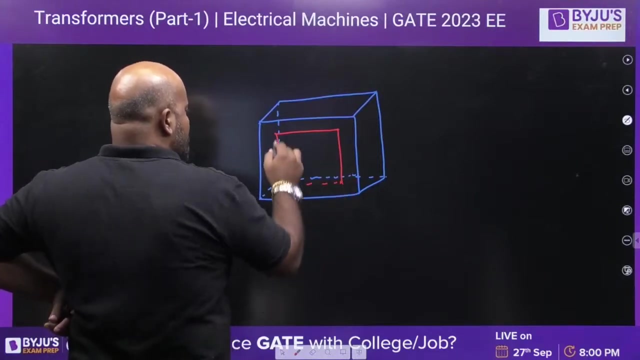 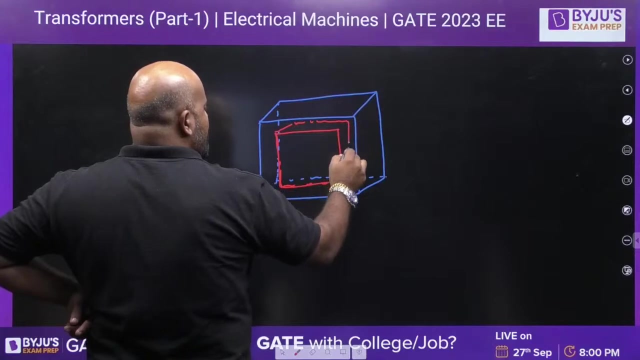 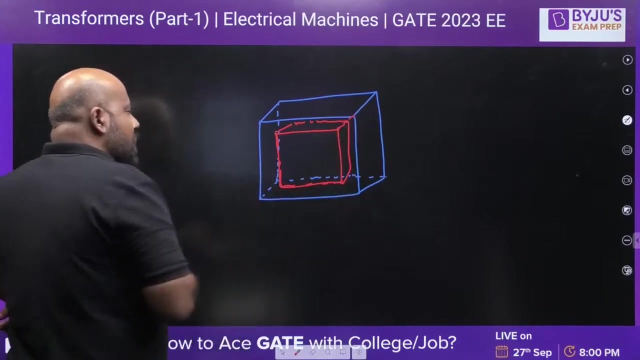 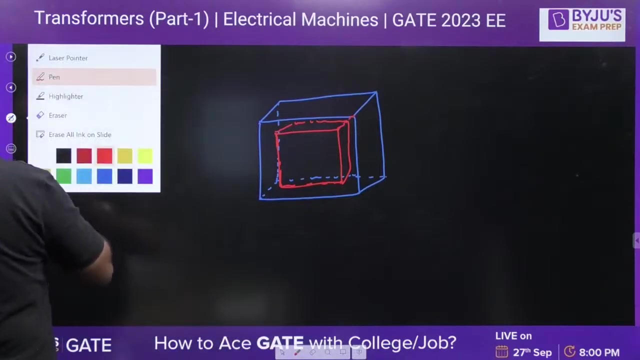 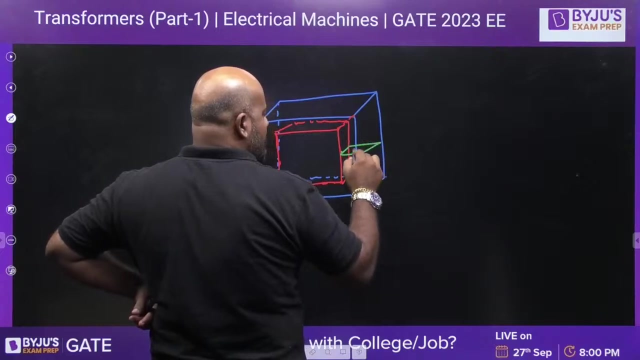 okay how i have to write. i am using another color, please wait. anyways, let me draw like this. only i hope you will understand, okay, okay, something like this. now, what cross sectional area? please try to understand. it is something like this. i am interested in this. are you able to follow this? 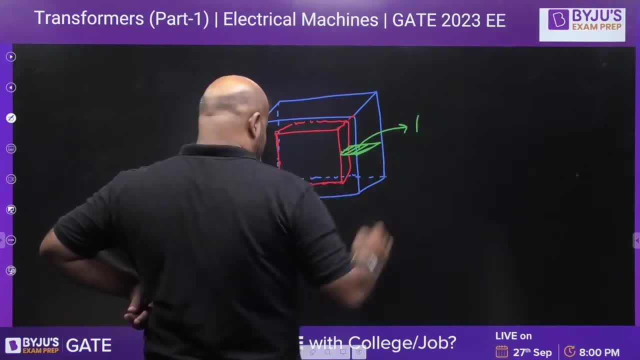 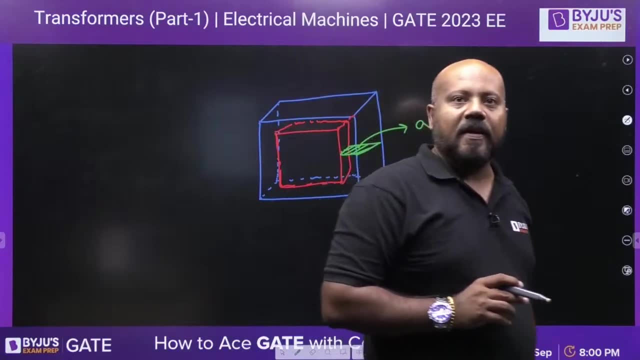 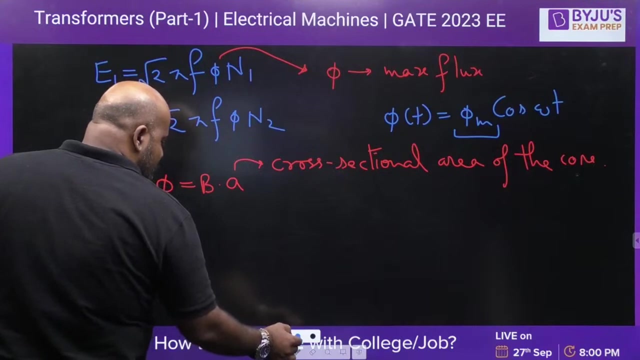 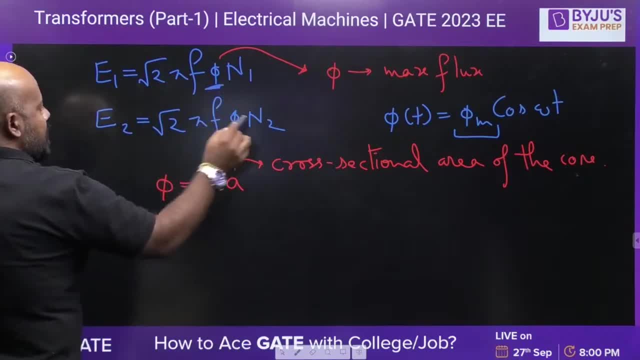 to write. you can write this flux, whether it is primary or secondary side. you can write that this flux is going to be directly proportional to, because root 2, pi constant, n, 1 is constant. So you can write: phi is directly proportional to E upon F. Now this E is going to be directly. 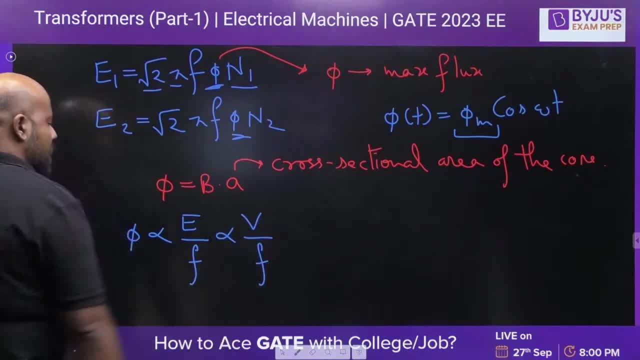 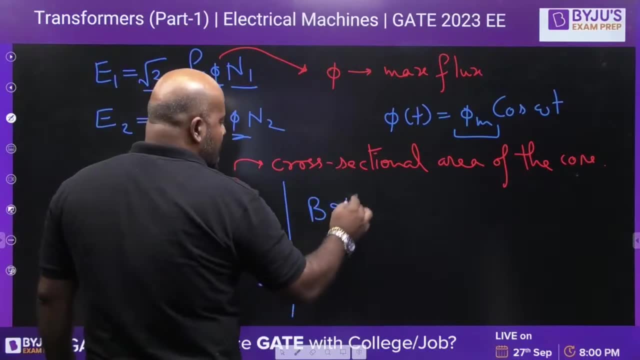 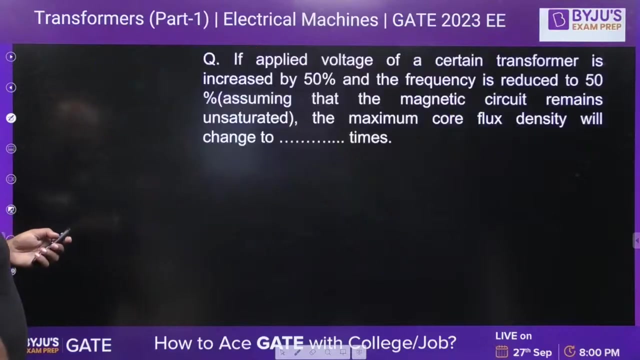 proportional to the applied voltage. So you can say V upon F, because flux is directly proportional to B. So you can write: B is directly proportional to V by F and you have to use this relation. If you write it, then you can write: B 2 upon B 1 is equal to V 2 upon B 2, V 1, then you 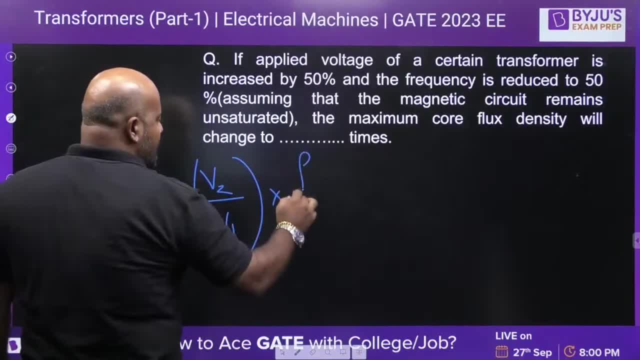 call it F, So you can write this as V 1.. If you write this as V 1 and you call it V 2, then you upon V 1, and this is F 1 upon F 2.. So if you write, V 2 has become increased by 50 percent. 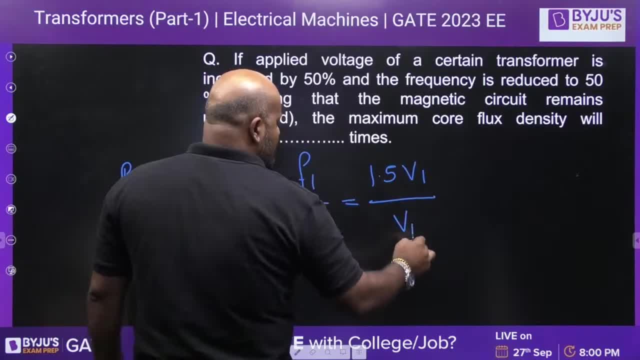 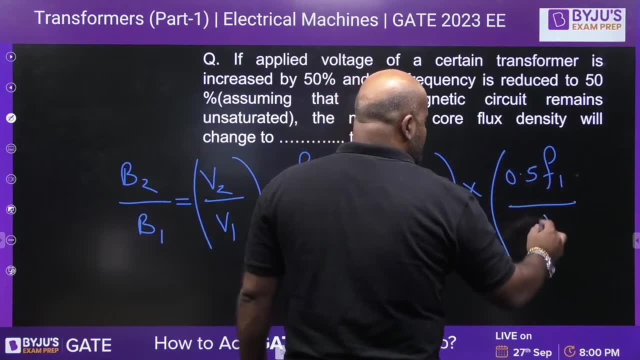 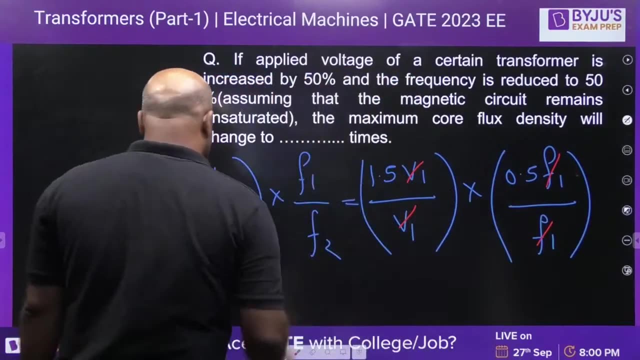 So it is 1.5 times V 1 and frequency is reduced to 50 percent. So this is 0.5 F 1, this is F 1.. So if you see V 1, V 1 cancelled, F 1, F 1 cancelled. if you simplify this, it is going: